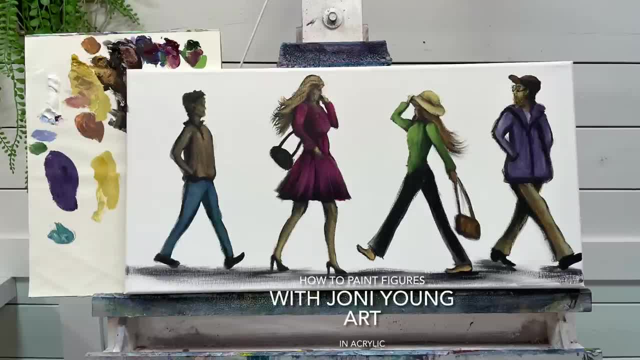 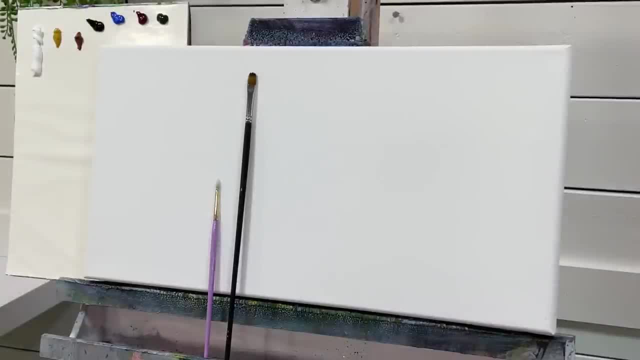 Hi everybody, it's Joni Young here. Welcome back to my channel for another painting tutorial in acrylics. Today I'm going to be showing you some more figure paintings: very simple, easy, basic steps so that all of you can follow along and learn how to add these into your paintings. 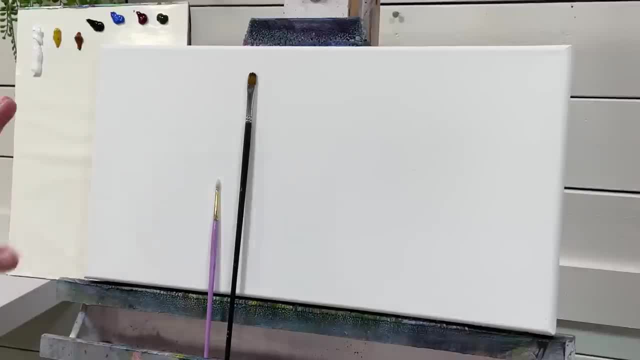 So I'm going to be working on a 10 by 20 canvas today, but you can paint yours on any size canvas you want. You can also use any colors you want. For this specific demonstration and tutorial, I'm using the following: titanium, white, yellow, ochre, burnt, sienna, mars, black, cobalt, blue, quinacridone, crimson and sap green. 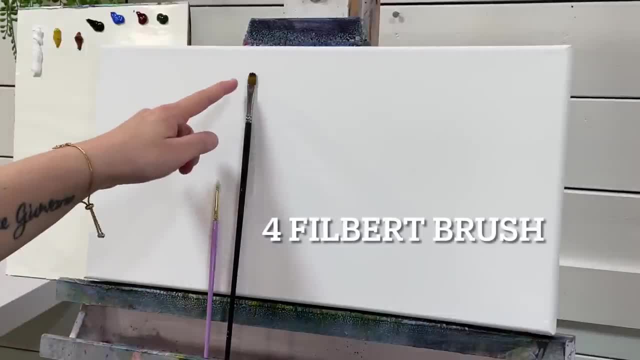 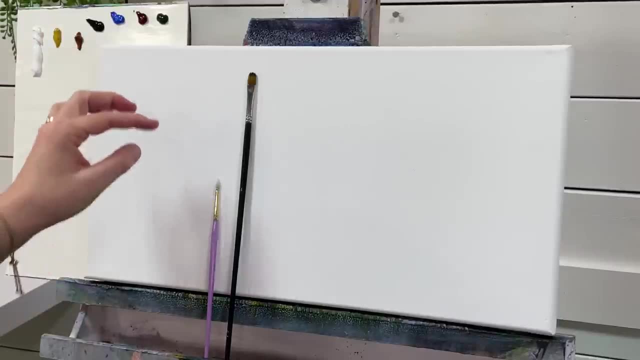 I have two brushes. I'll be using a number 4 filbert brush and a number 3 round brush. I'm going to use the round brush for smaller details and lines, the filbert brush for the basic shapes and silhouettes. 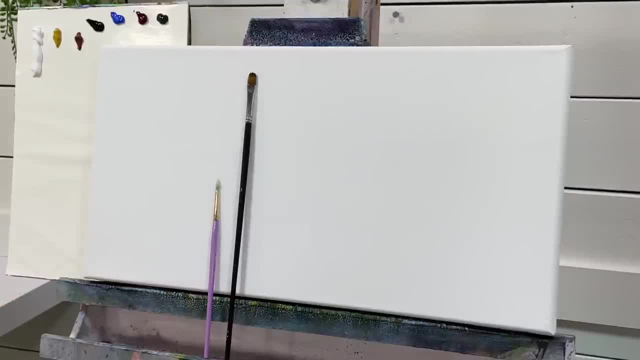 So if you guys are ready and excited to learn how to paint some figures today, hit subscribe and let's go ahead and get started. Okay, so we're going to go ahead and get started. I'm going to be using my filbert brush. 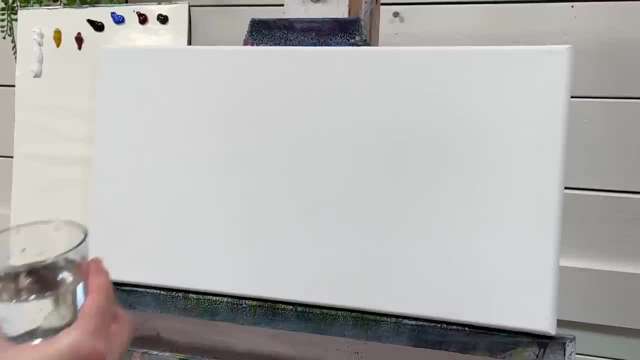 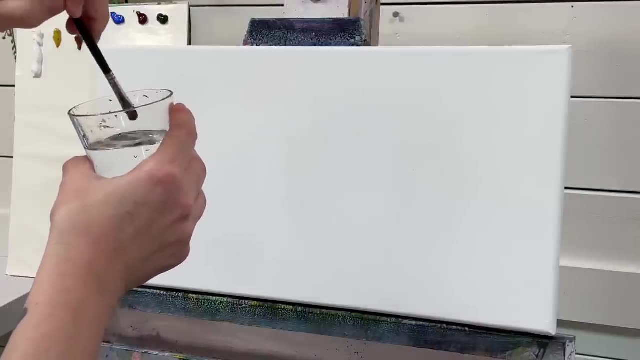 I've got a little cup of water here to show you how much water I'm using, And we're just going to break it down into simple shapes and colors. today, I'm just going to add a little bit of water to my brush And then the first color I'm going to take is a little bit of black. 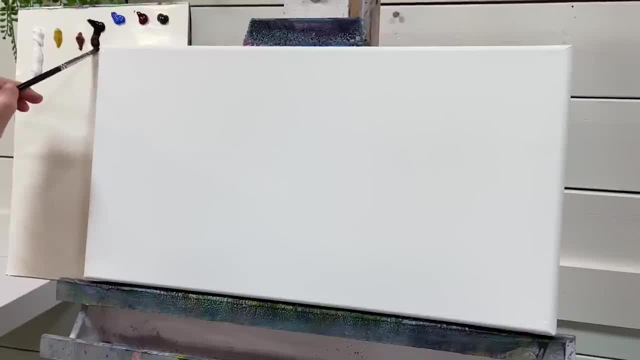 So I'm just going to add black first, Little Little bit on the end of my brush, So you don't need too much paint. Biggest mistake new painters make is overloading their brush, And so we're just going to start with lines like this: 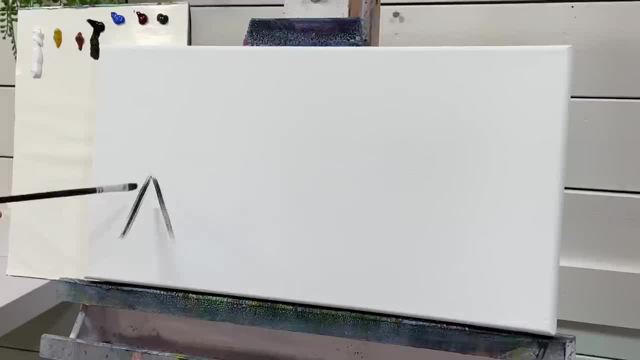 Just make a simple peak like that, or the starting of a triangle, but it's not going to complete right down here. So then we're going to start to make them a little thicker. This is where I'm going to take a little bit more water. 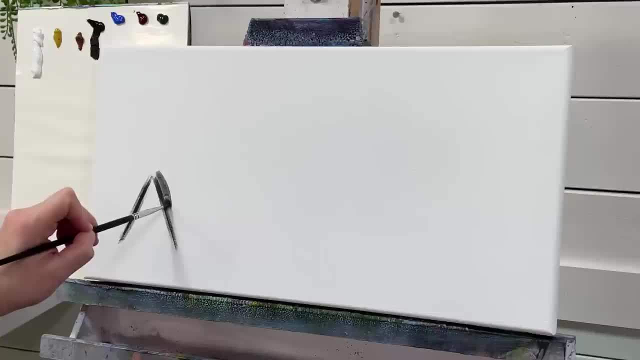 And the thigh is bigger than the knee, So we'll just add a little bump there and then the calf down to the ankle gets narrower. Let's take a little bit more paint now, Go over that, And then we're going to work on this one. 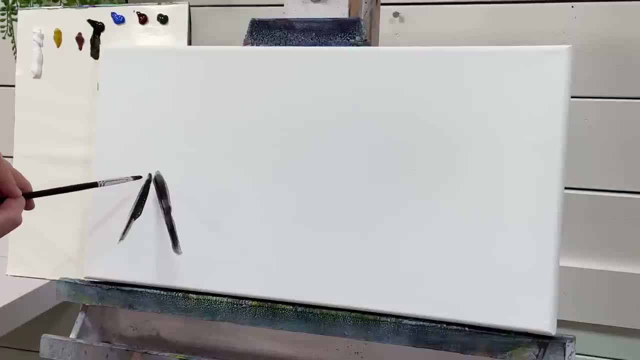 So this one's going to start to bend. We've got the knee right In there by the knee and then we're going to pull it back just a little bit for that calf. Just pop that out a little bit, bring this in around the bottom area and make this start to come up straighter. 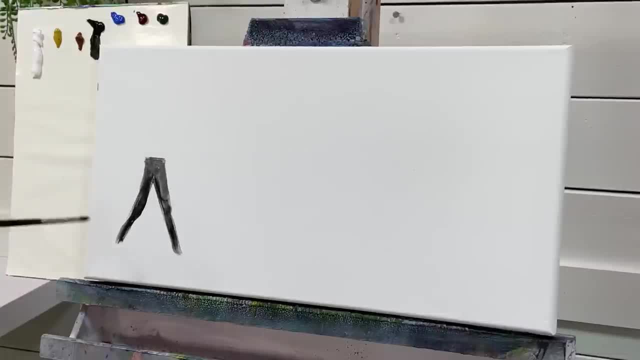 And then we're just going to pull a line, a little line, to connect them right like that. Now, if they've got baggy pants, You might want to make it a little bit wider for the bottom of the leg of the pants. 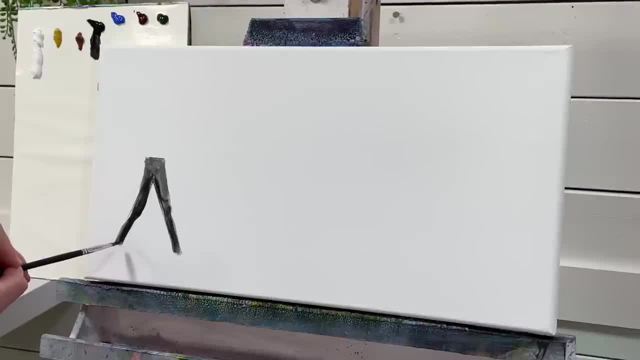 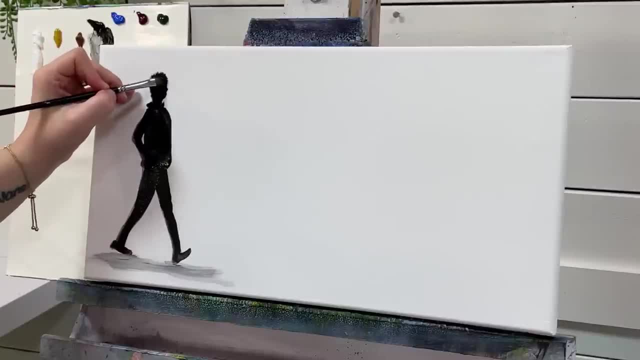 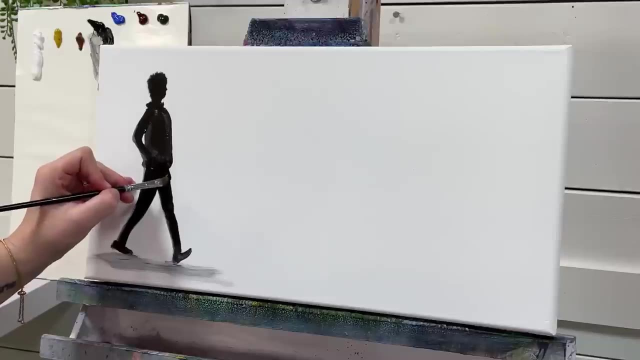 of the brush, a little bit like that, and they've got a basic figure walking again. just go back and make it a little bigger, wider, wherever you want, depending on who you're painting. so we're just going to. i'm going to demonstrate them in black silhouette first, and 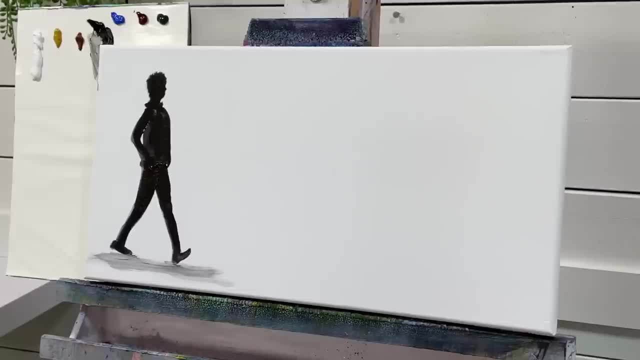 then we're going to come in after it dries and i'll show you how to add color to them. and now take a little bit of black again, again, not too much paint, and we'll add the legs. here i'm going to paint a lady now. 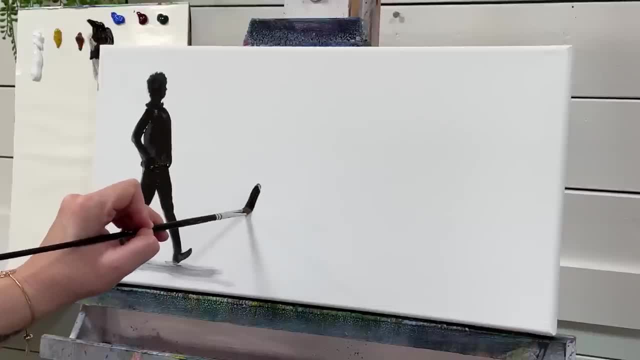 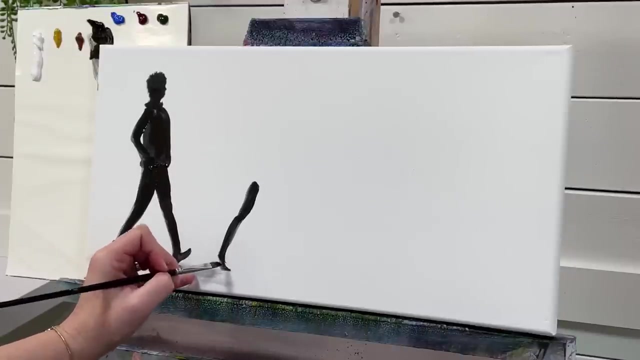 her thigh knee. so we're going to just pop it out a little bit and then bring it back in and then her calf goes. the calf goes out that way and then just bring it down into a point and then flat for her shoe, just twist over with the end of the foot. 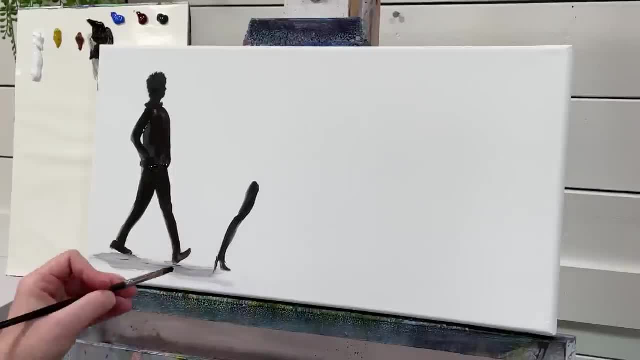 fill filbert brush and add the heel that pops out just a little bit. then we can add a shadow at the base. i'll take a little bit of water again thin that paint out. okay, then we're going to add just a little scoop here for her dress and then start her next leg. 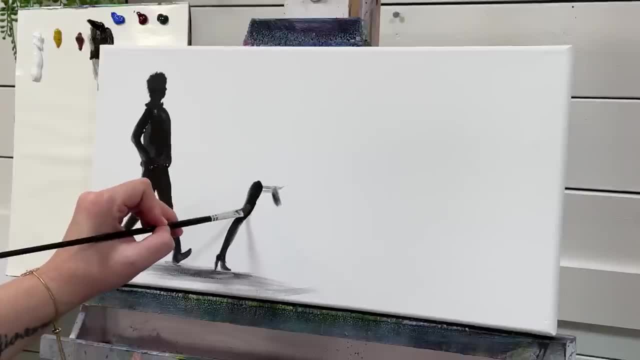 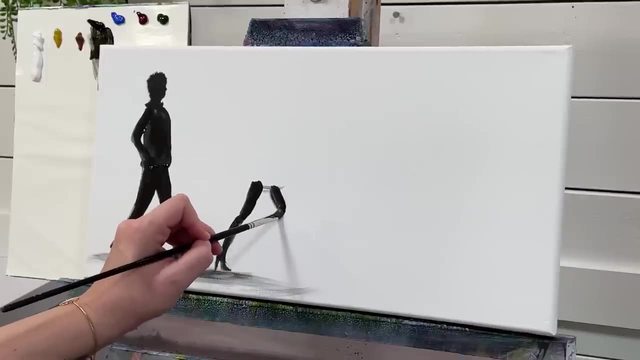 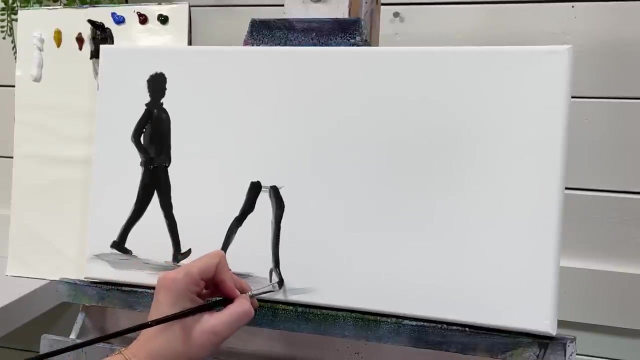 make this a little bit thicker here and her knee is going to be right here, okay. so a little line there, the knee, bring it down, and then just a little rug pop her the heel out right there, just twist and turn over on a slant and then flat again. 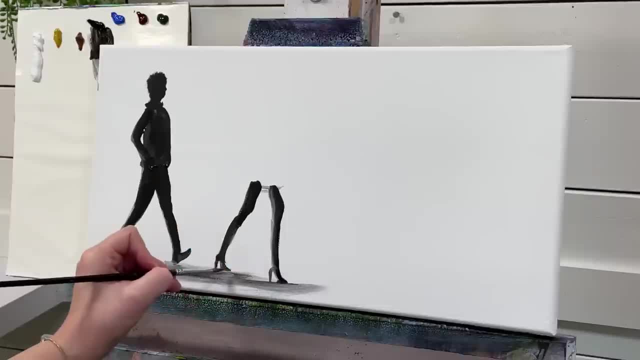 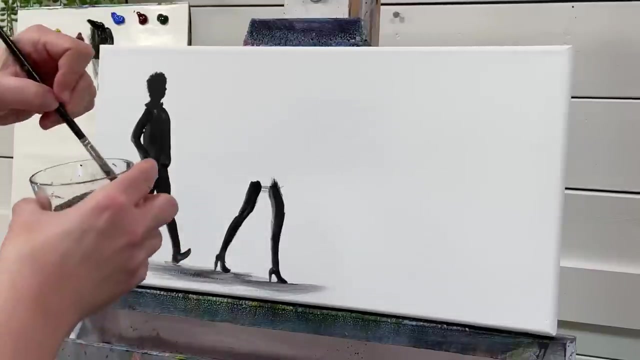 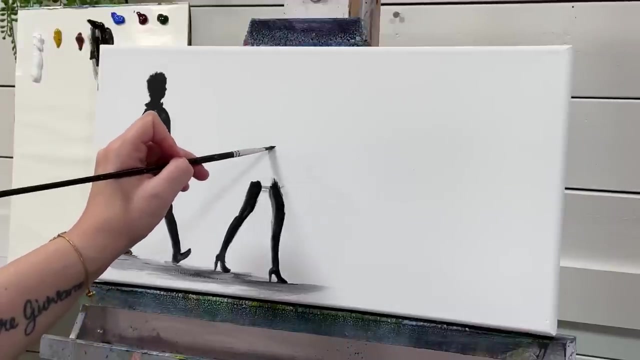 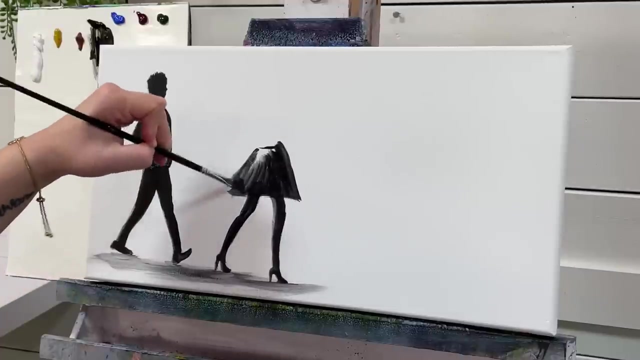 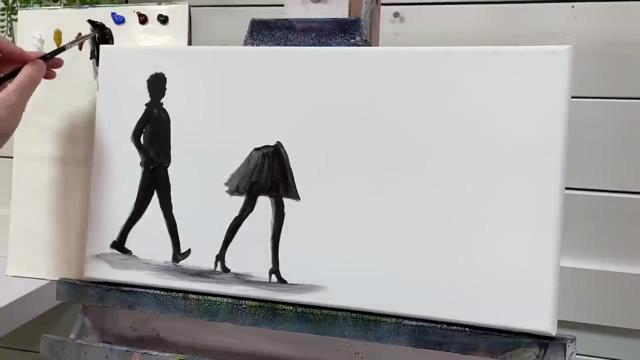 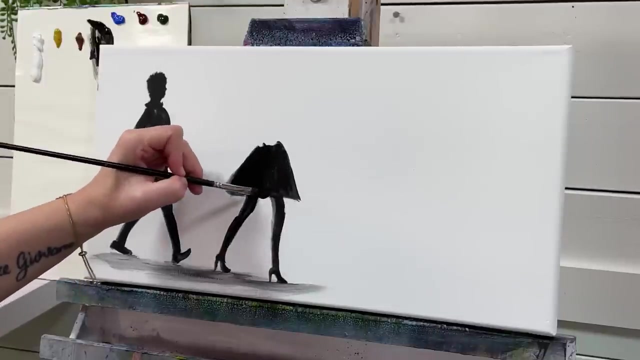 oh yeah, okay, now we'll add her dress or skirt. we're going to start about an inch up from the legs. we're going to add a little line right here and we're just going to pull across and paint it in. we'll bring that material- her skirt or dress- over the legs here in the front a little bit more. 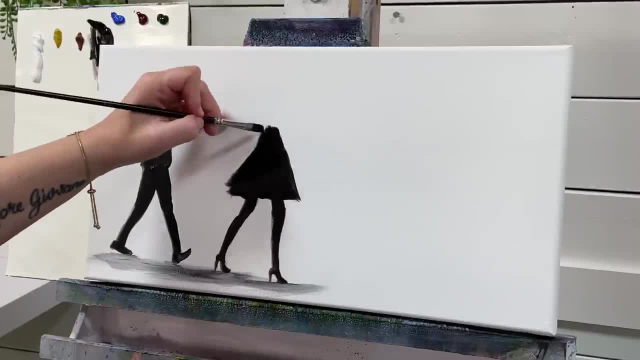 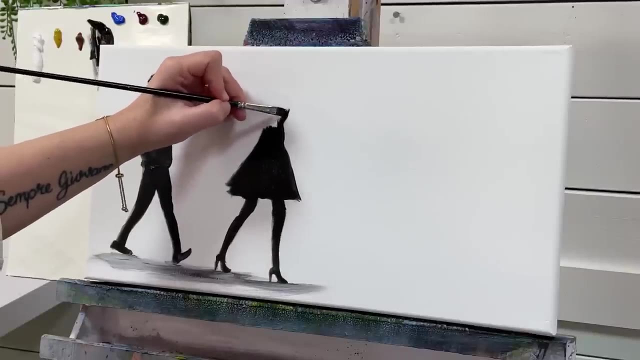 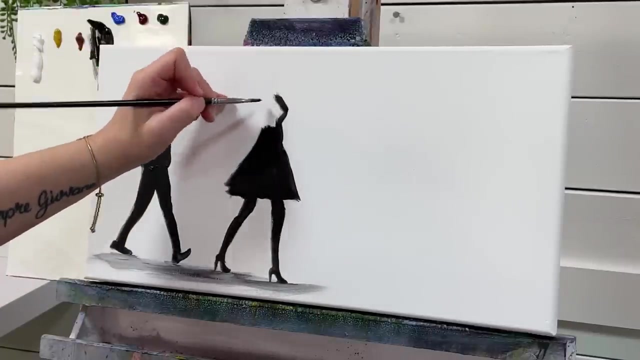 and then we're going to go and bring it up, keep a little bit of a slant right here and then we'll add a little bit of a roundness here and then bring out her chest breast area so to a point in and then a little bit roundish there. 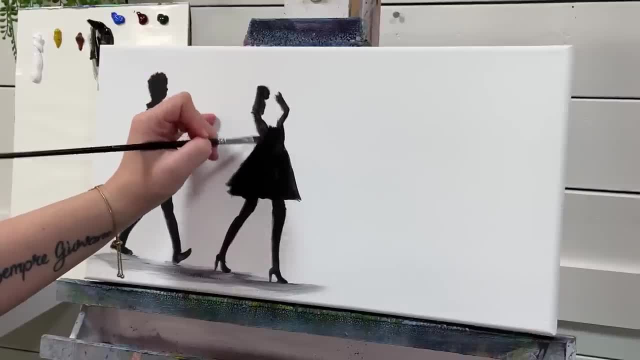 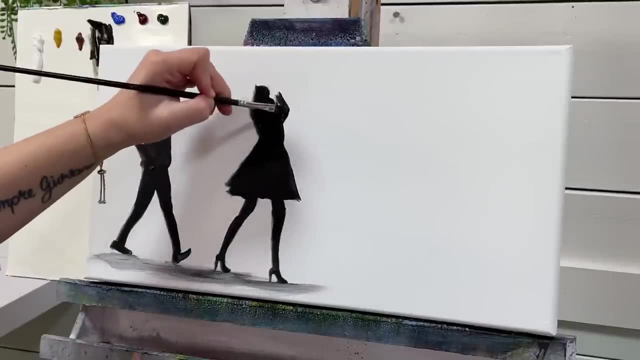 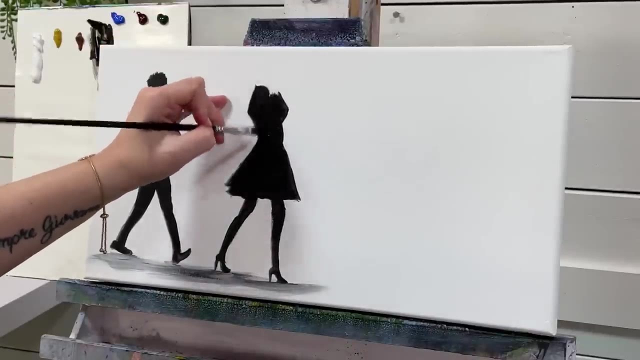 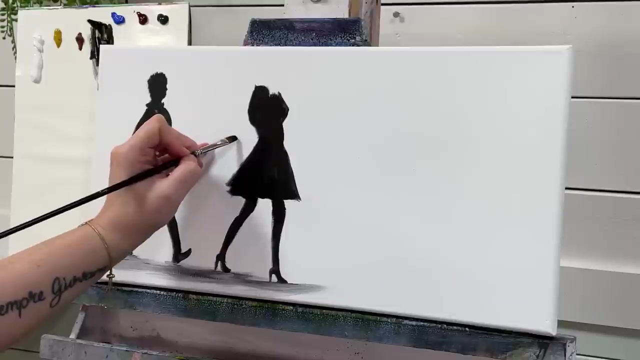 and then we'll add an elbow that comes down here, her arm, and then we'll paint this in. then i'm going to give her a little purse to wear. i'm going to just add a little oval here on a slant, just a simple little oval. you can make your square if you want a rectangle. 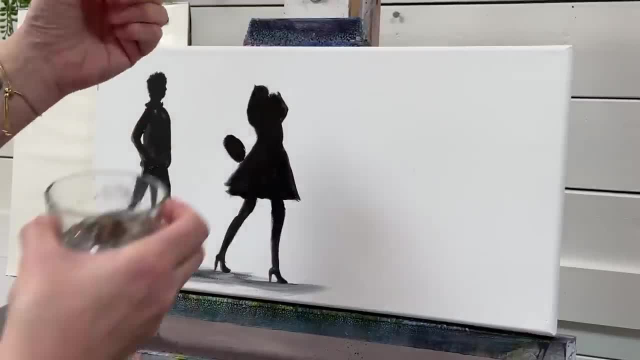 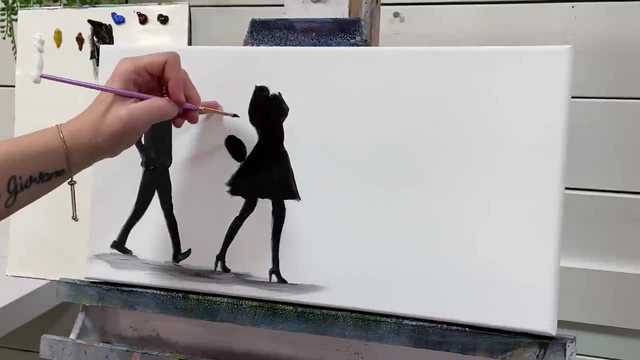 i'll just set that aside for a moment and we'll take our round brush so it's easier to make finer lines with a round brush or a liner brush, and we'll add two lines that come down there so it looks like she's carrying a purse. 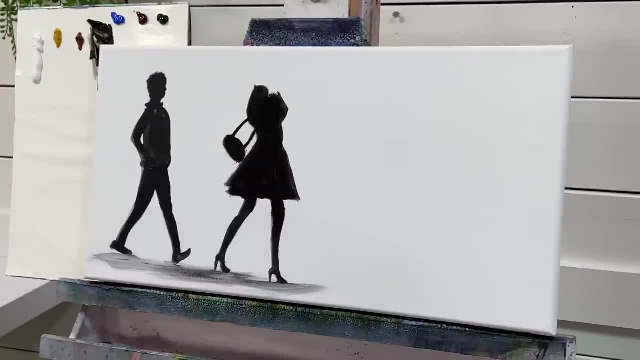 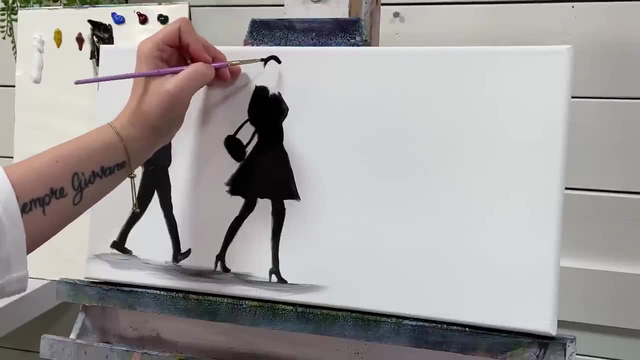 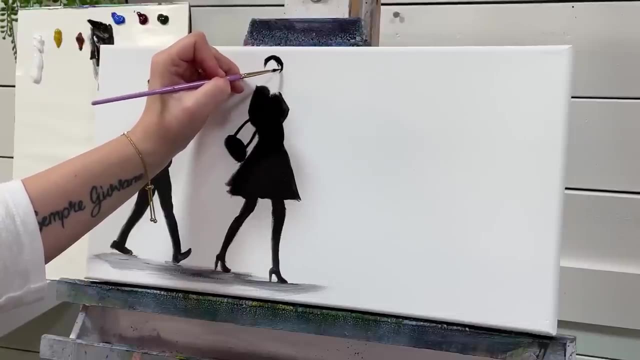 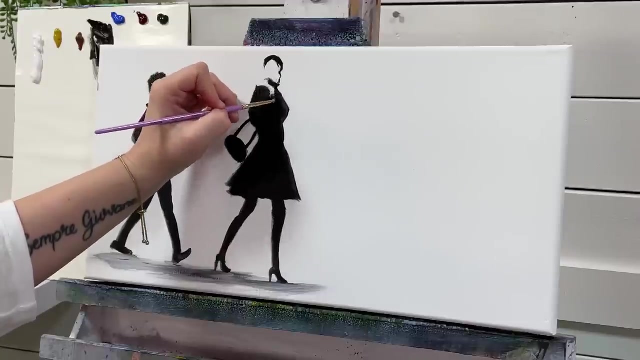 and then i'm just going to continue using this brush. for now. we'll add her skirt, We'll add her head, we'll add half a circle right here. bring some bangs out, pull it in for her eye area and then her nose. a little chin, just a few little bumps there, and then just 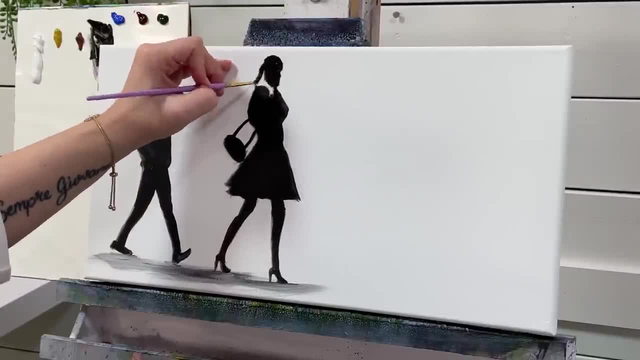 paint it in. I'm going to add some hair. I'm going to take a little bit of water on my brush, thin the black out and again we'll go over the top of the head there and we'll make her hair kind of flowing and paint the same silhouette. 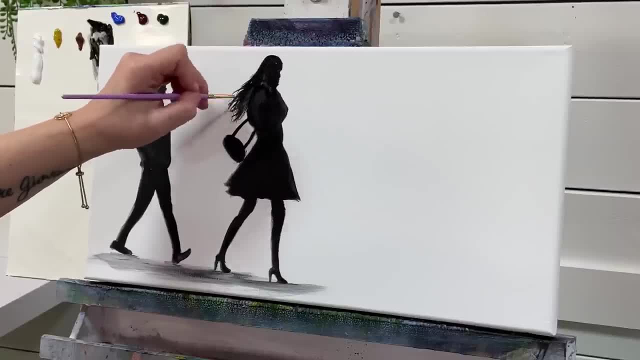 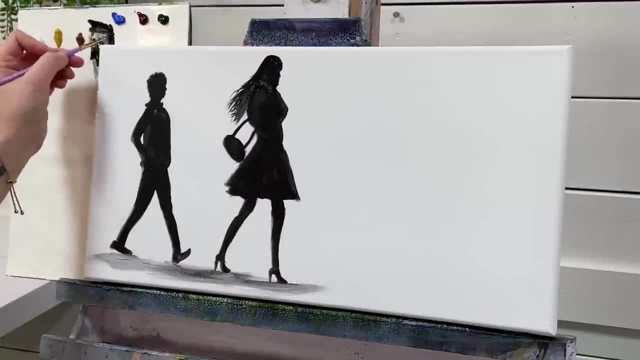 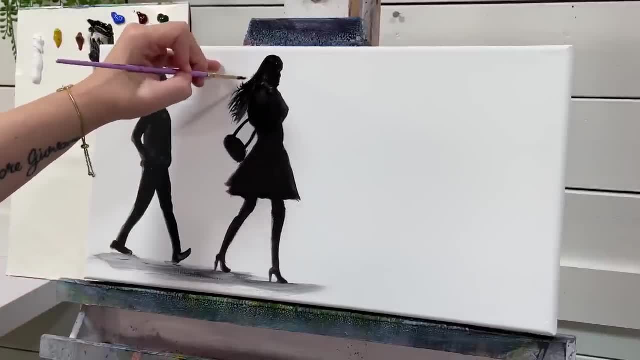 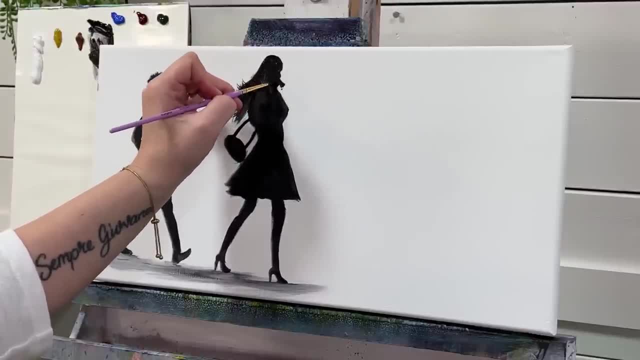 Maybe she's got her hand and her phone over here on this side and she's on her phone, so we'll just add a little rectangle or square here coming out from her jaw and chin area, and then we'll add her wrist here. 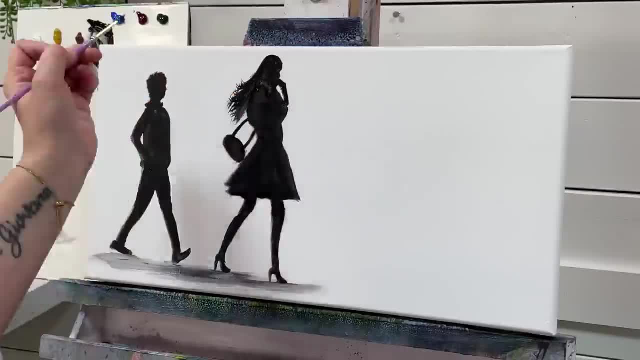 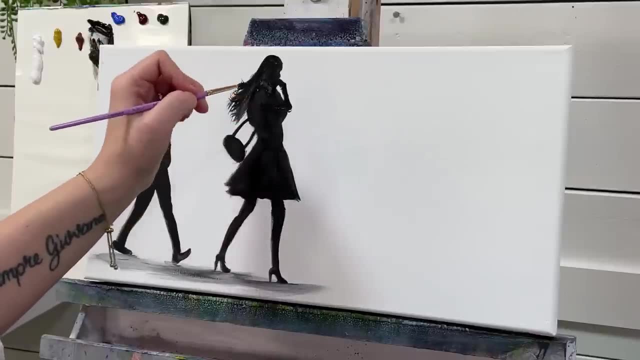 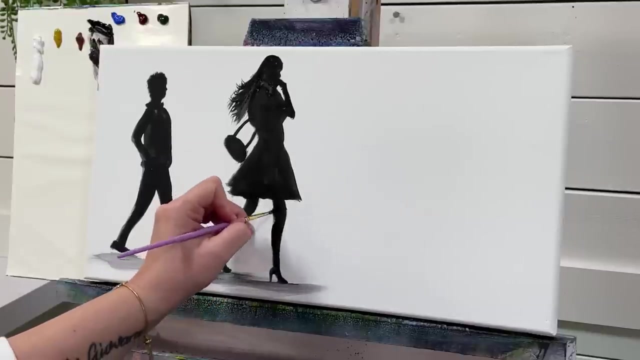 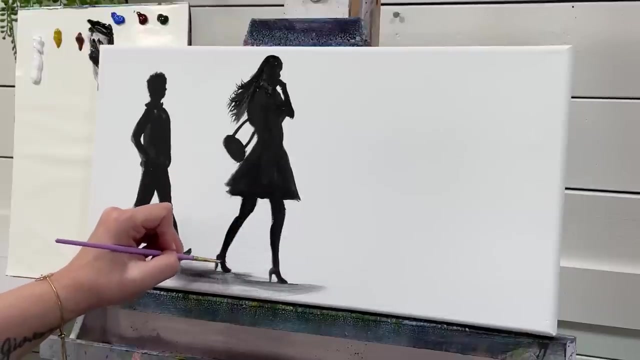 And this, of course, is just on the other side- And her elbow. Bring it down a little lower, a little pointy, and back in. I'm going to make her calf come out a little bit more here. Let's go into our black again. 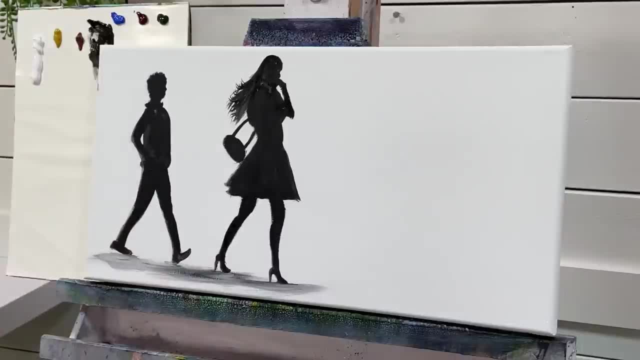 Okay, just a little bit of paint on there. It goes a long way. And we're going to start right about here. the waist area, Start with a waistline for a line just to go by for the leg. And then we're going to start right about here, the waist area, Start with a waistline for a line just to go by for the leg. 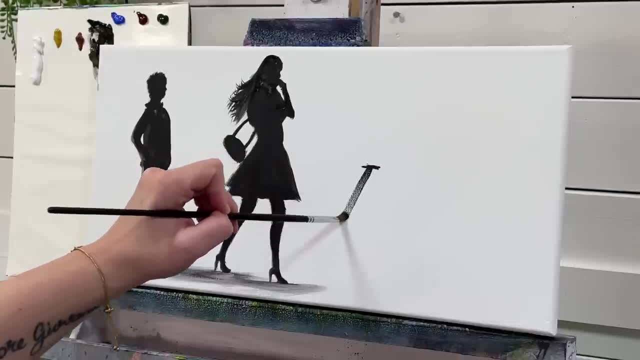 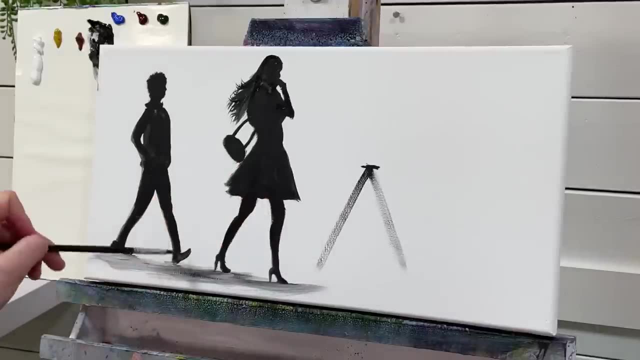 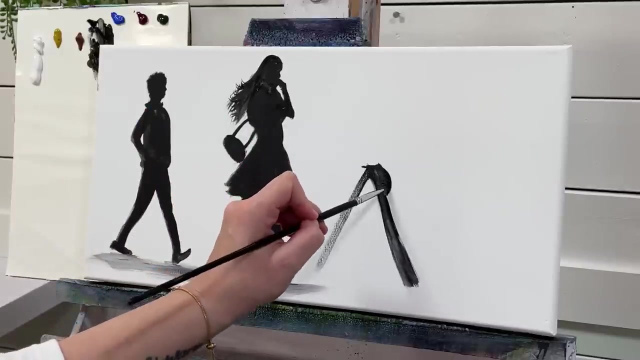 And we're going to add that sort of line that we started with the peak. A little bit more water on my brush And we'll have this person wearing wide pants. We'll round out their facing this way. We'll round out their bottom. 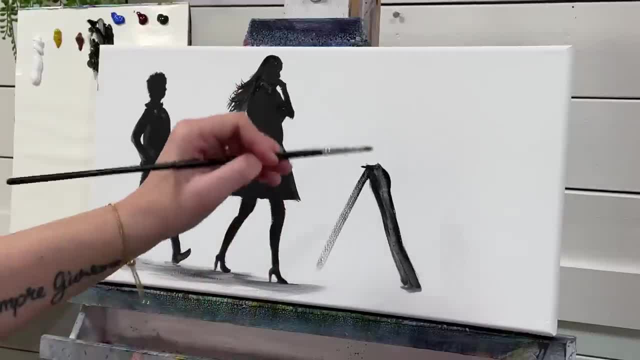 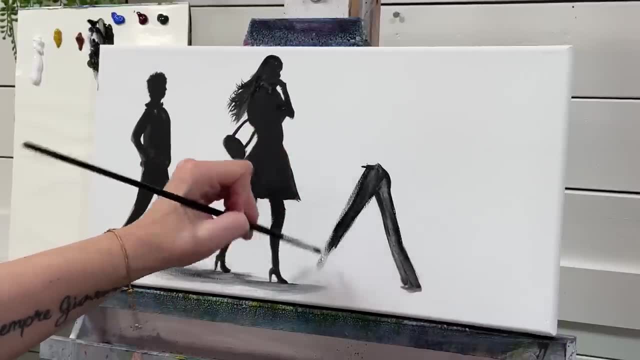 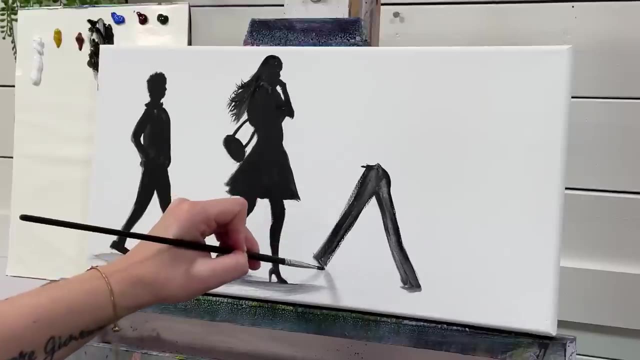 And give them some wider pant legs. Okay, and then we'll widen it this way: This leg here is in the front And then on an angle, because that's how we want to make her foot up in the air a little bit mid-step. 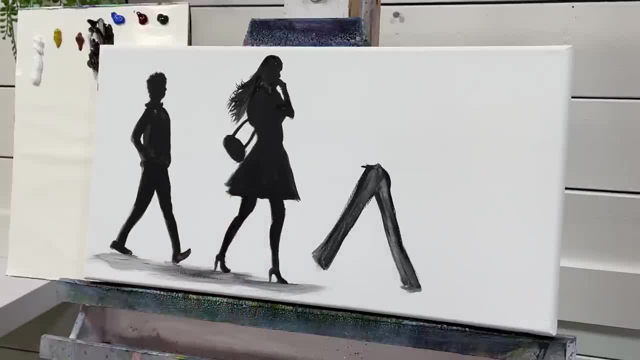 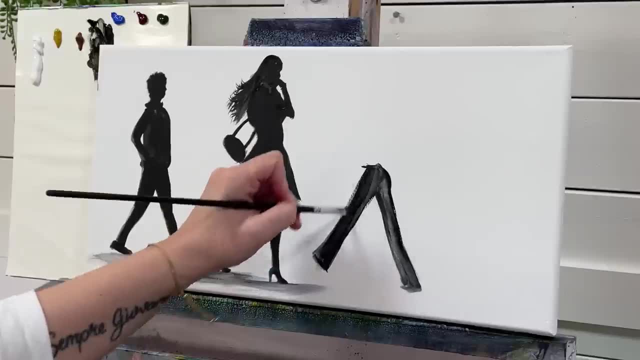 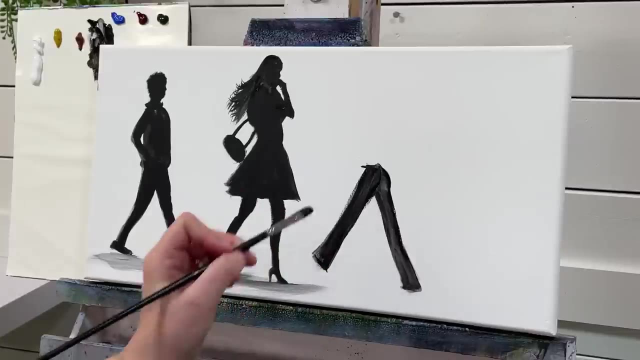 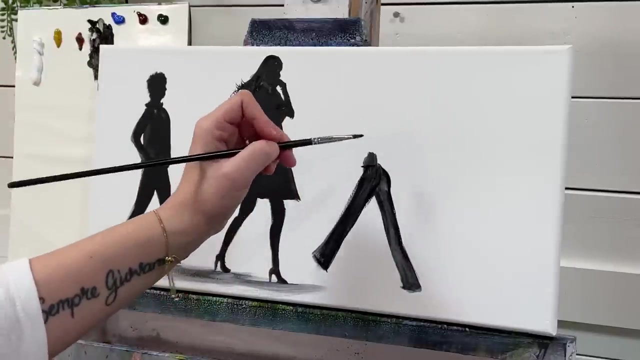 So I'm going to smooth that out a little bit. I'm going to add a little bit more black here. Then we're going to work on the waist. We'll do the feet or shoes in a moment. We're going to gently round out the bottom part. Make sure that your toes are in the middle on that side of your shoe, Okay. so we're going to make sure that the top and bottom are in the right spot. We're going to turn that over, Okay, and then we're going to round out the bottom part. We're going to do that again, but I'm going to finish up the top. Okay, so now it's nice and smooth, but I think it's hair. We're going to do the center a little bit later. We're going to speed it up a little bit. 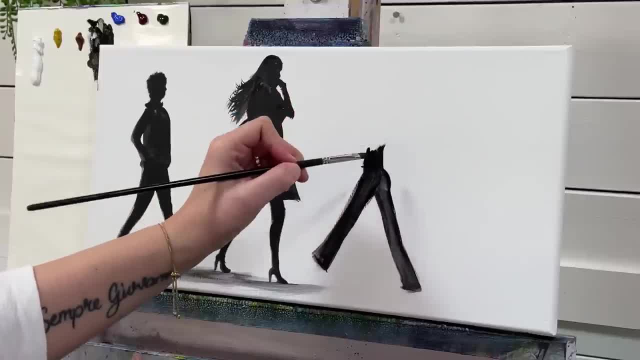 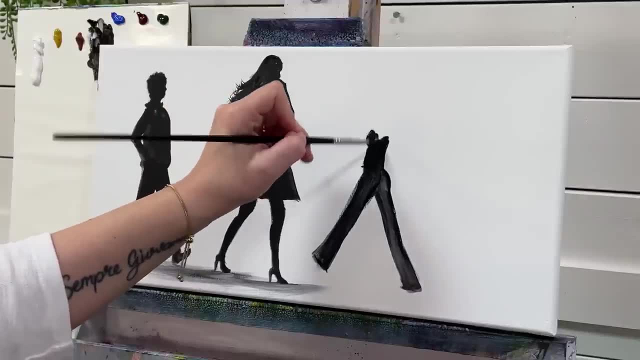 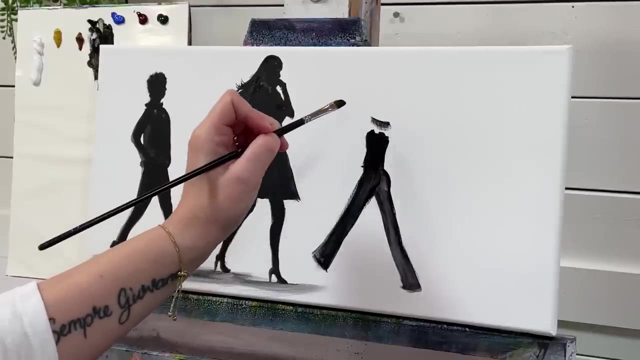 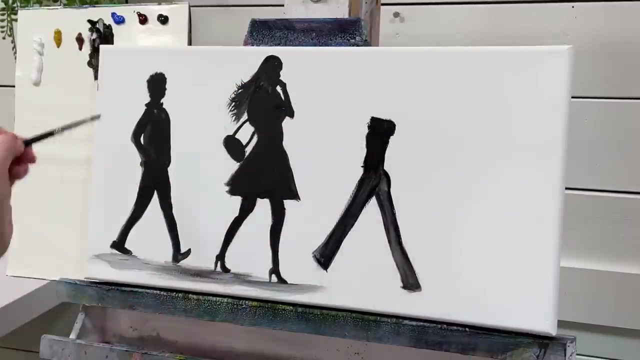 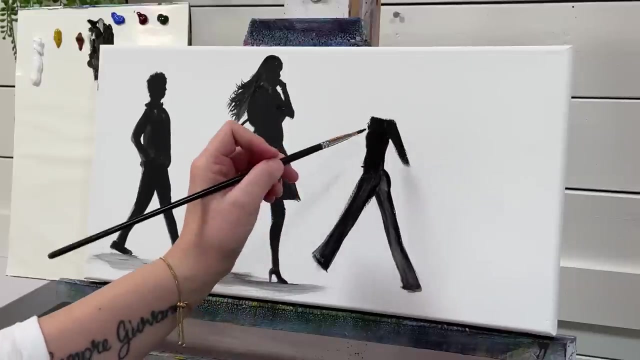 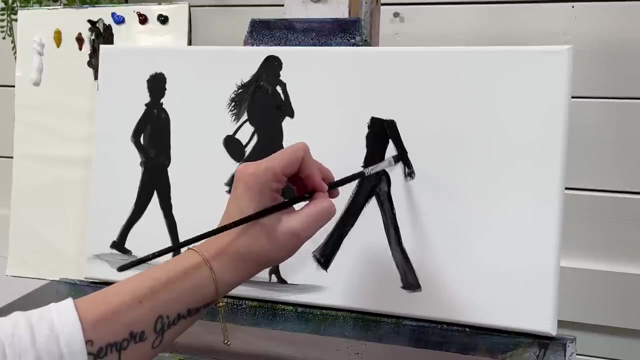 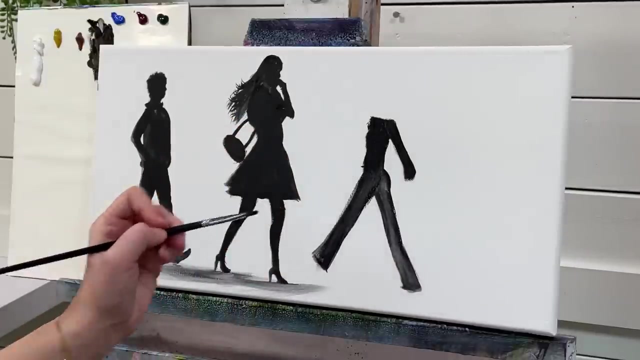 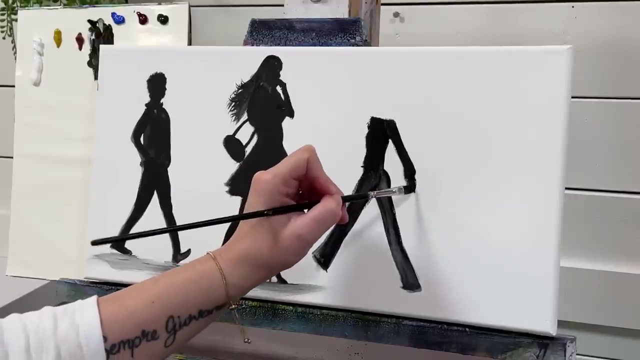 the waist, bring the back, scoop and slant over slightly. maybe add just a little bump for the chest area and then shoulders, bring that up, paint it in. okay, her shoulder elbow would be right about there- and then we'll give her kind of a flouncy cuff and then we'll have her holding a bag. now let's just make. 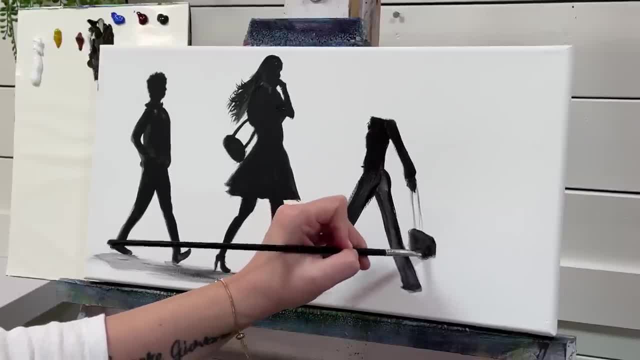 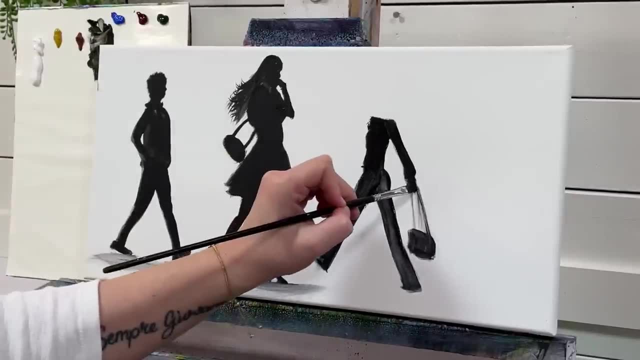 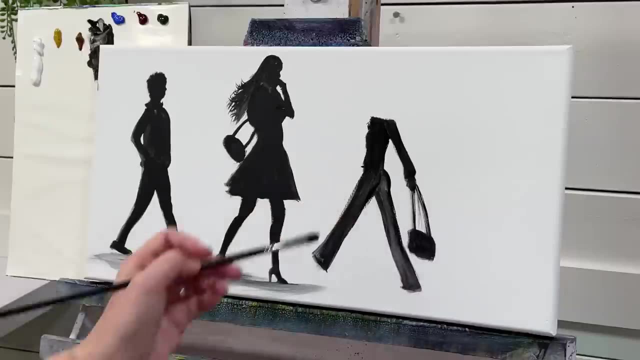 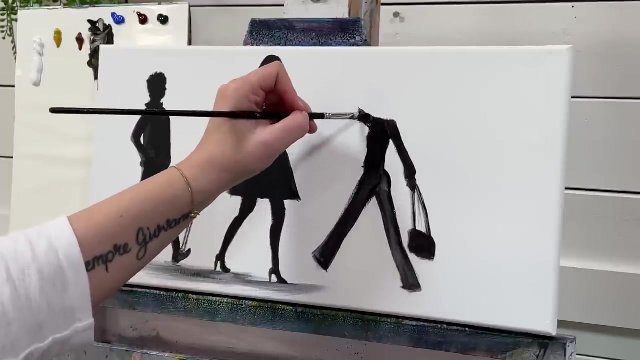 this one more of a rectangle, so you can do this with your round brush- it's whatever you feel comfortable with- or using the filbert, okay, and then we're gonna have her other arm come up here because she's gonna be holding her hat. so right about here is it will be the elbow. we're gonna stop there. 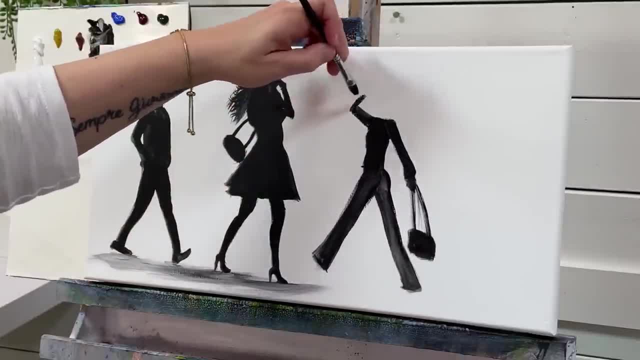 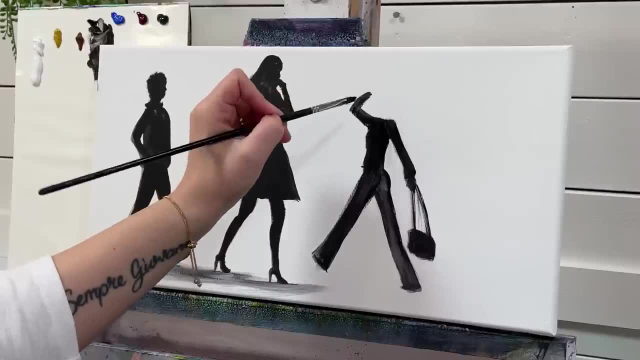 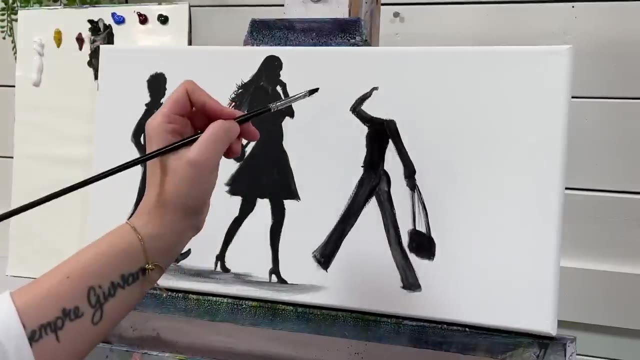 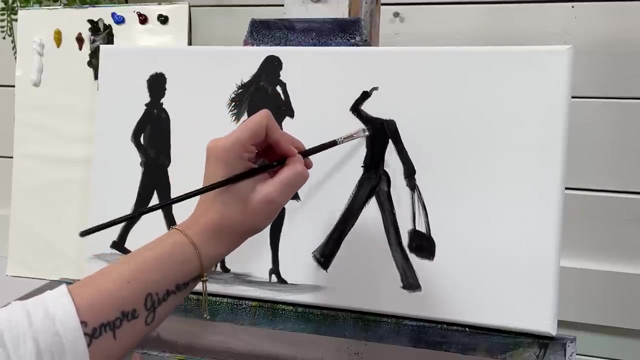 on an angle and then we're gonna have her wrist area here get narrower, add a little curve like that where she's gonna be holding her hat, and just a little bit more handled there, and then you can go ahead and let the shoulder go out really slowly. I think this is going to go really nice. this one right here is going to look like a bun, and then what I'm gonna do is take this bit and open this big, ardent ep impostor and pull this off of the nappy anymore. there's not going to fit it in any, any opinion. click that button and then let's fell into the mat and we're going to practicing this around the neckoupe. so I'm just going toEND those. actually, I do want to point out the mean head cut and spreading this, because the client might want to learn to look at the Philosophy wisdom, if you'd like. 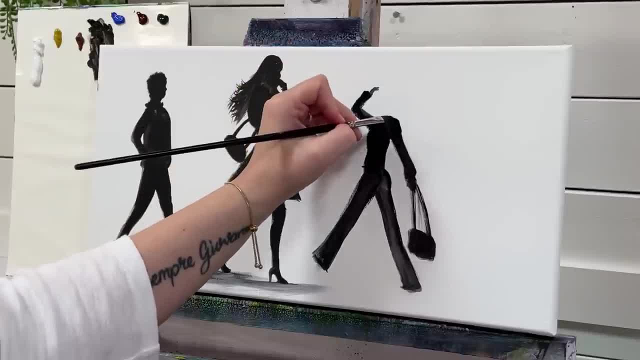 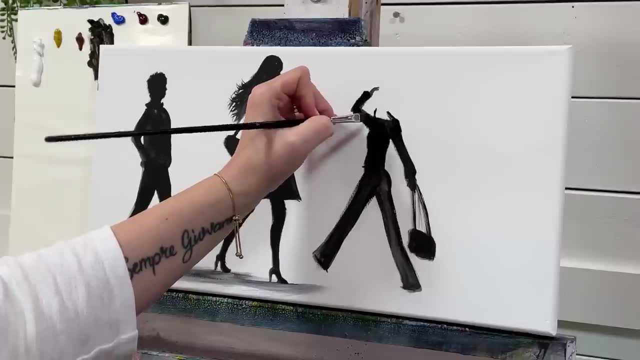 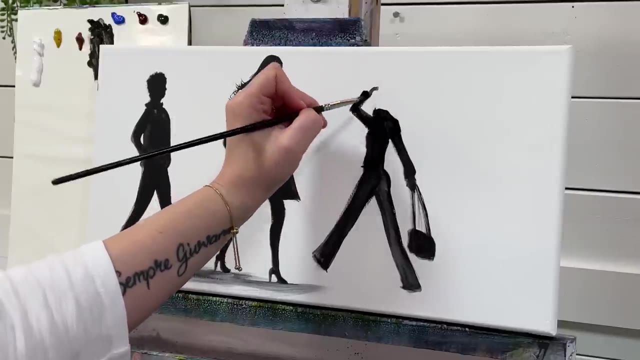 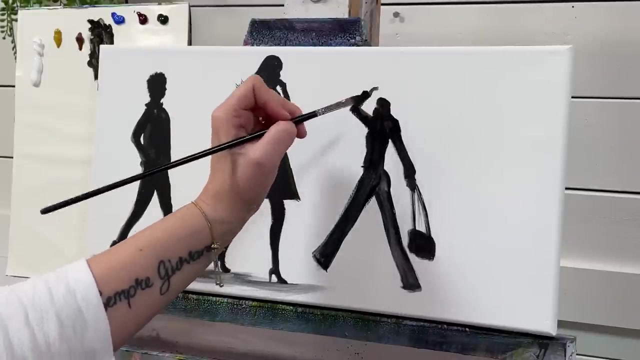 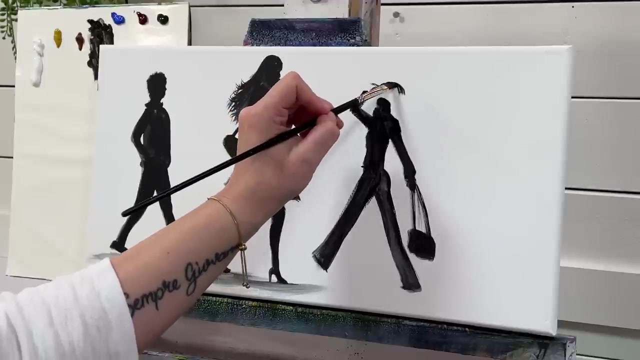 to my brush, gently pull on a slant this way, then we're going to pull straight up here. we'll paint that in, bring it up a little higher here, but keep this slant, and then we're going to add the top of the hat, rounded. a little round part to the hat and then another. 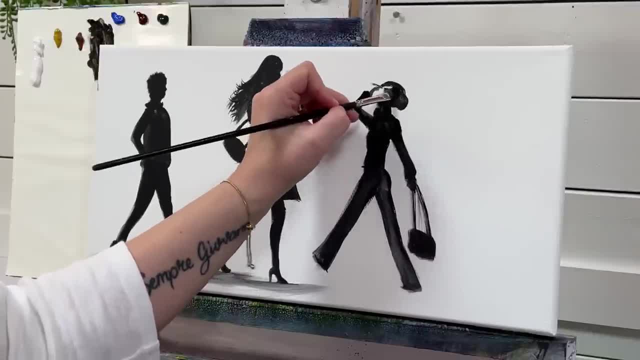 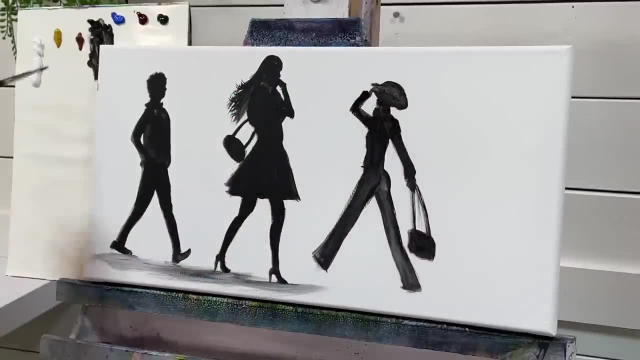 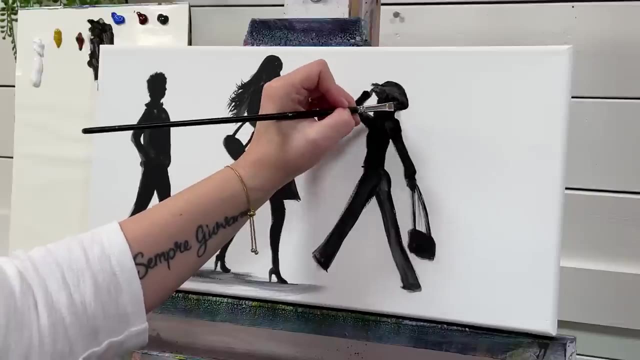 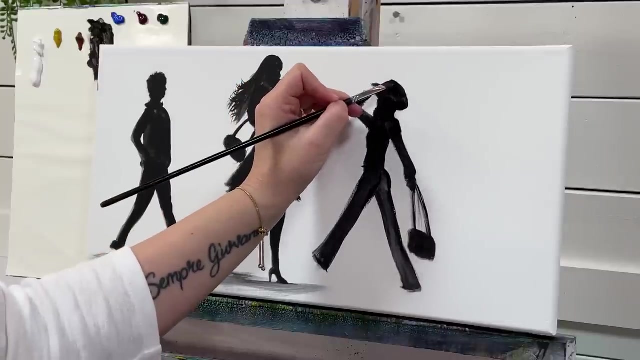 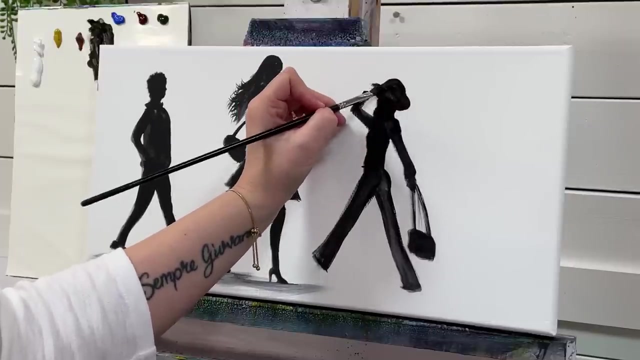 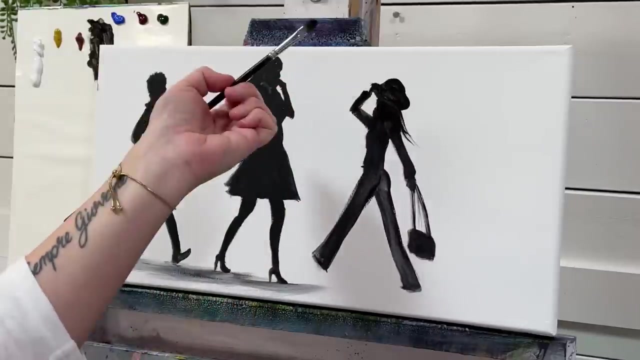 one that comes out just to the shoulder. let me pop this up just a little higher right there, and then I'm going to give her a little bit of hair too, because I think that would be kind of pretty, and show you how to do it with the filbert brush here. 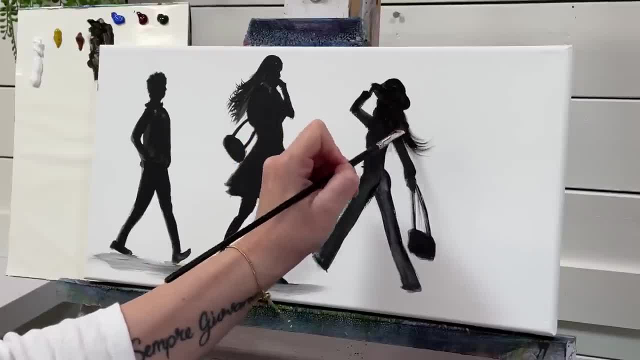 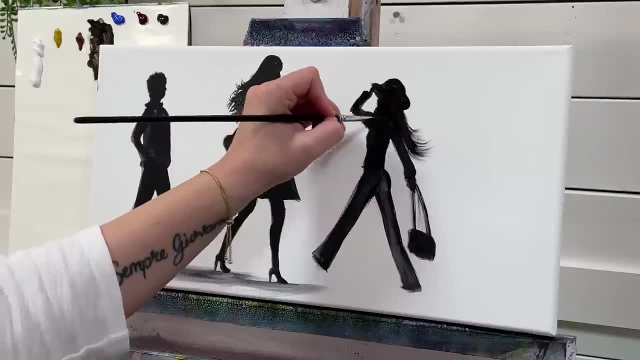 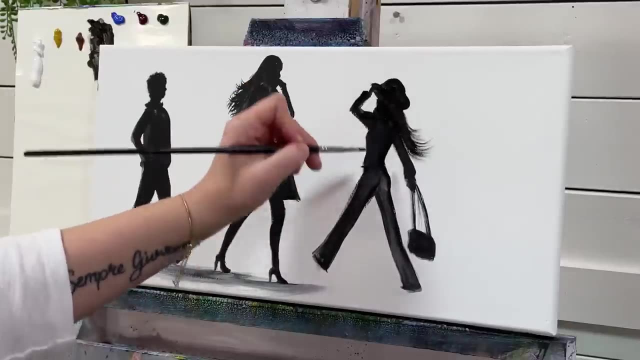 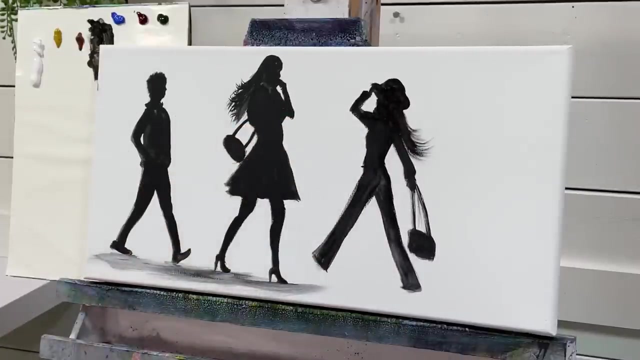 add a little curve and scoop and flick. okay, so now switch over to the brown brush so we can paint her shoes. a little water, a little bit of black, and we're just going to start inside, about the middle of the pant leg. gently scoop a little bit and then come down, scoop. 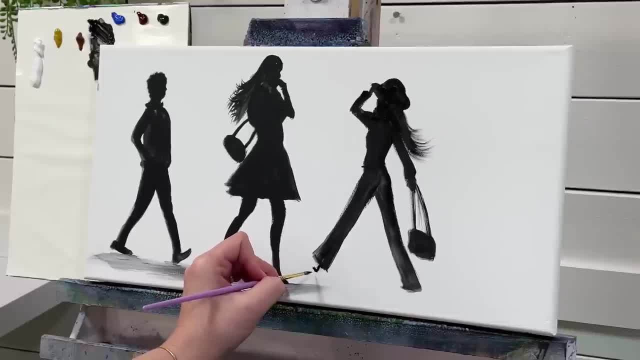 almost like an S shape right here. then bring it up a little bit and then up again, so S, and then scoop in, and then up on a slant and scoop okay, and then this one- we're going to start back a little farther heel, so just scoop out, pop that out half circle. 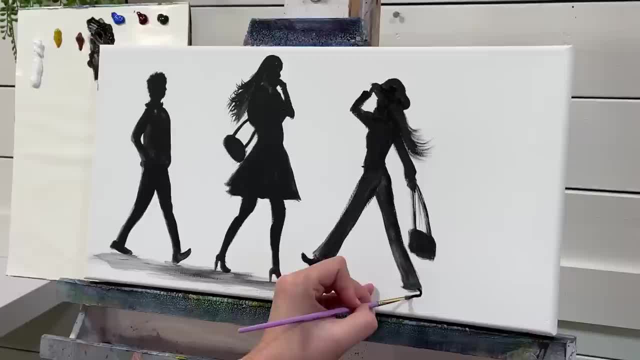 okay. and then this one: we're going to start back a little farther heel, so just scoop out, pop that out half circle, okay. and then this one: we're going to start back a little farther heel, so just scoop out, pop that out half circle, then on a little slight angle, and then pull it back over. 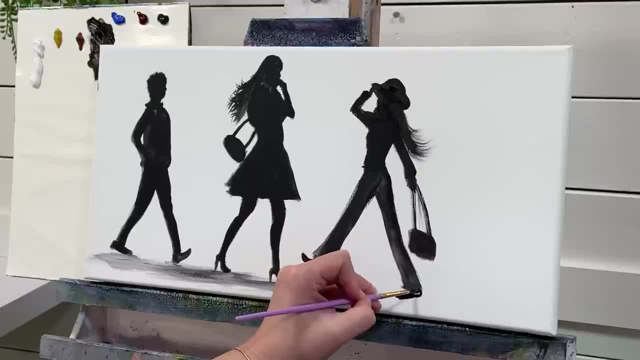 then on a little slight angle and then pull it back over, then on a little slight angle and then pull it back over. this kind of looks more like she's this kind of looks more like she's this kind of looks more like she's barefoot, and you can change it by adding. 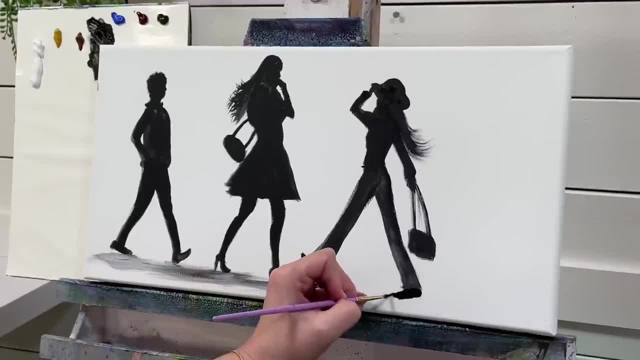 barefoot, and you can change it by adding barefoot. and you can change it by adding a little heel, like we did here, and a a little heel, like we did here, and a a little heel, like we did here, and a little scoop, little scoop, little scoop, or just adding a wedge heel. 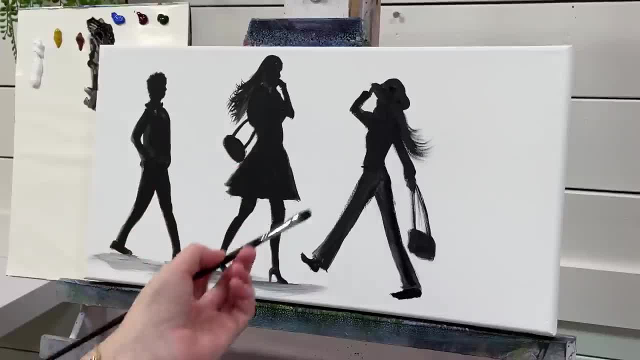 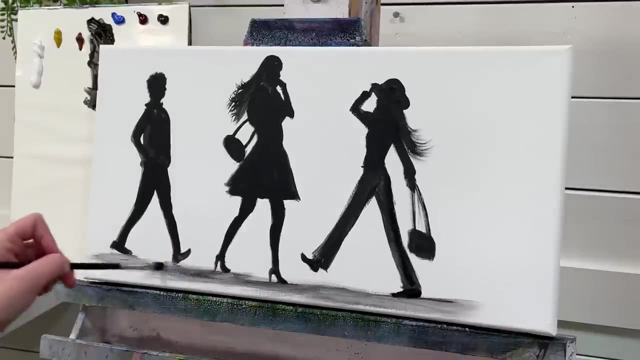 a little bit of a little bit of a little bit of water down, transparent black. okay, i think i've got room for one more. okay, i think i've got room for one more. okay, i think i've got room for one more here. so i'm going to add a little bit. 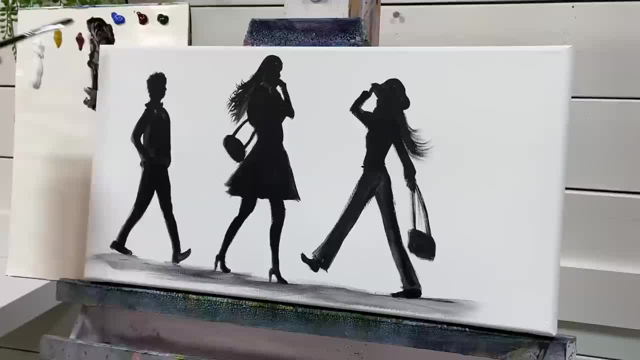 here. so i'm going to add a little bit here. so i'm going to add a little bit of water to my brush. again of water to my brush. again of water to my brush. again some more black. we're going to start with the top this. we're going to start with the top this. 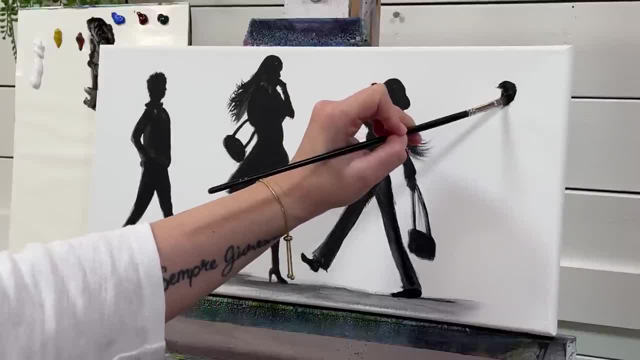 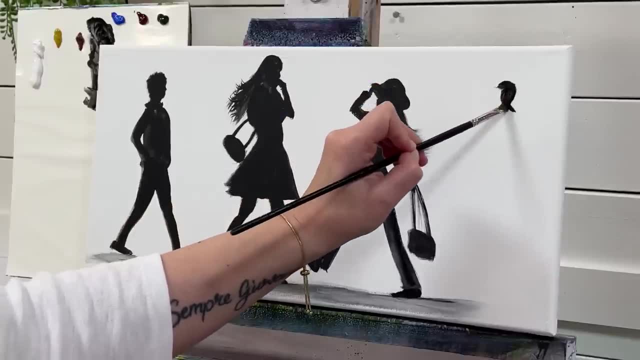 we're going to start with the top this time. time time we'll add roundness there, we'll add roundness there, we'll add roundness there. so half a circle there, so half a circle there, so half a circle there. then then, then bring it out. 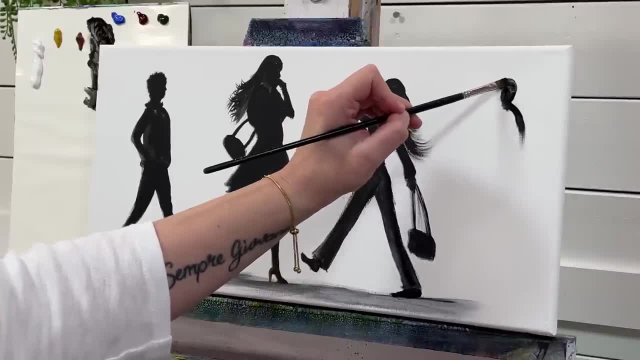 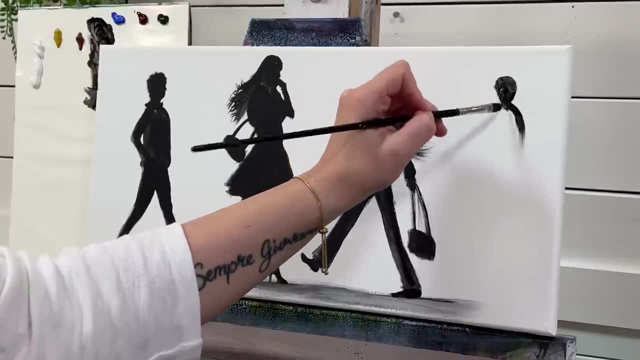 bring it out, bring it out down, down, down. we'll bring the height of this up a. we'll bring the height of this up a. we'll bring the height of this up a little bit more. and then straight down here, and then straight down here, and then straight down here on an angle. 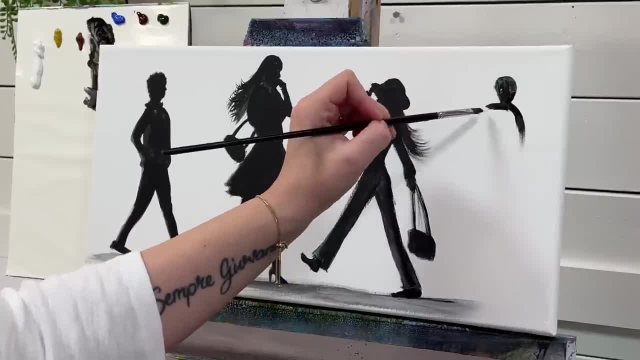 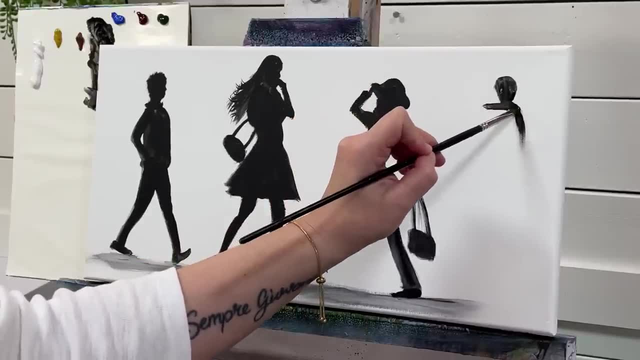 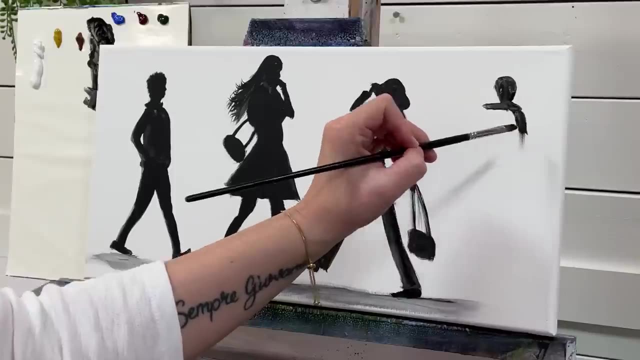 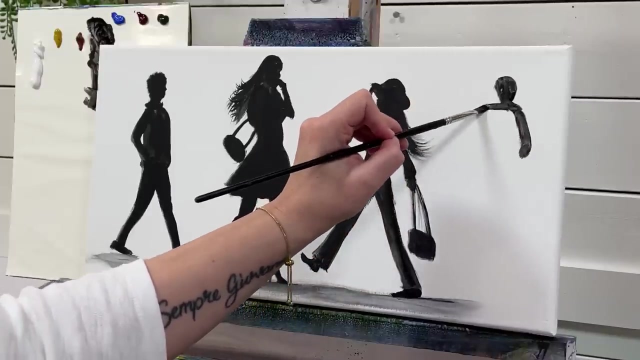 on an angle, on an angle. bring it out a line here a little, a little, a little: collar, collar, collar, sticking out, sticking out, sticking out. bring the shoulder out a little bit. bring the shoulder out a little bit. bring the shoulder out a little bit more, then we're going to pull in. 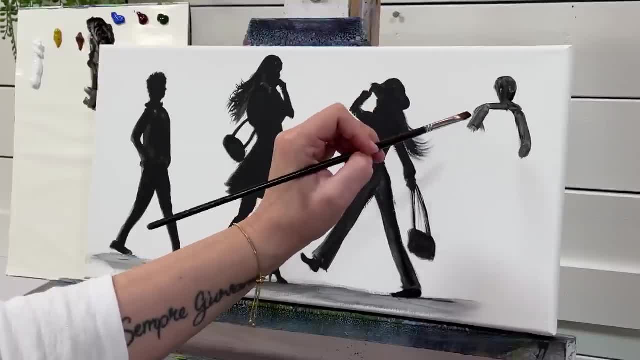 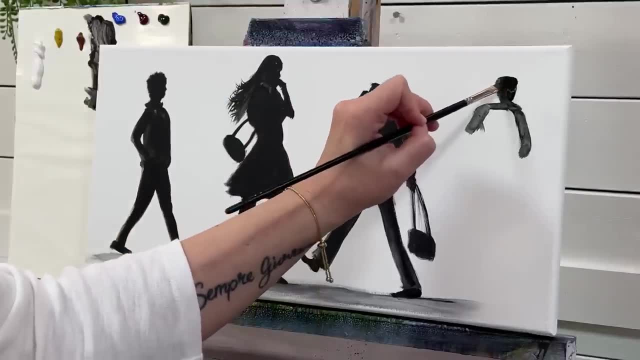 then we're going to pull in, then we're going to pull in this one, this one, this one, we're going to bring down, we're going to bring down, we're going to bring down on an angle, on an angle, on an angle. grab a little bit more black here. 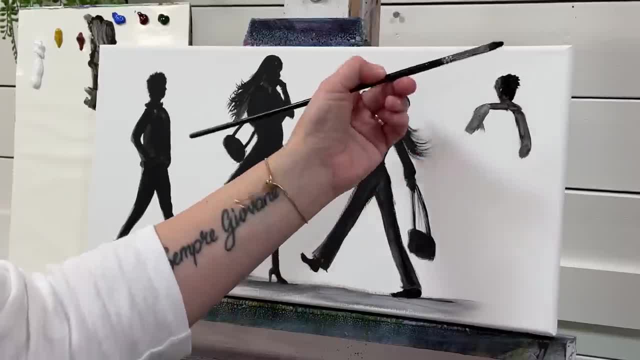 tap in a little bit of hair, just turning tap in a little bit of hair, just turning tap in a little bit of hair, just turning my brush on the side to use the end. like my brush on the side to use the end, like my brush on the side, to use the end like this. 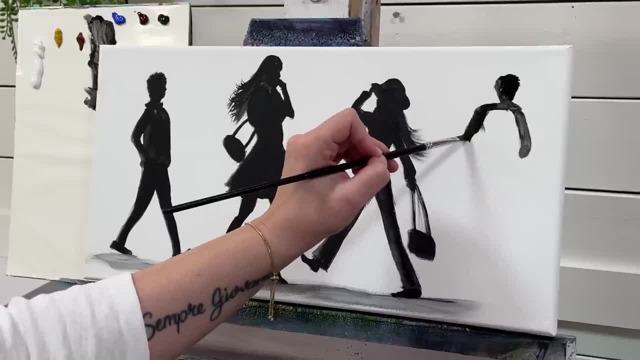 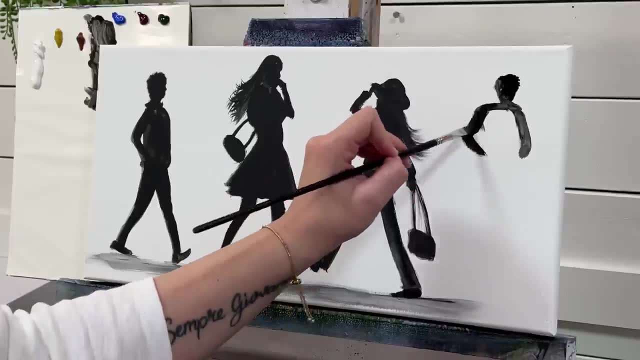 straight shoulder on an angle. bring the straight shoulder on an angle. bring the straight shoulder on an angle. bring the elbow out here, elbow out here, elbow out here, and then a little bit narrower there, and then a little bit narrower there. then we're going to leave a little. 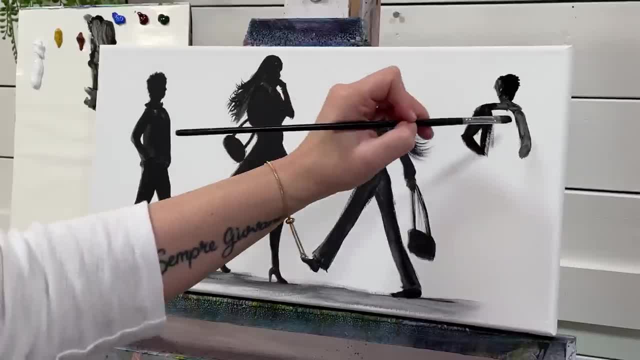 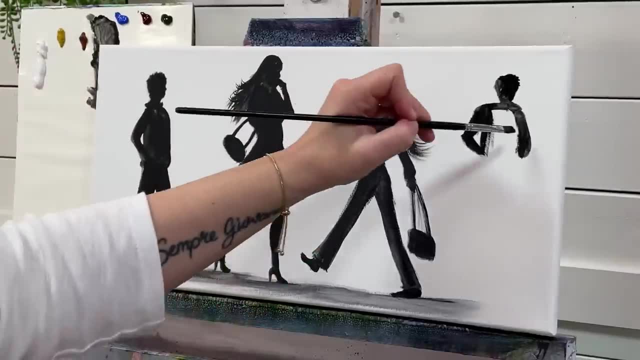 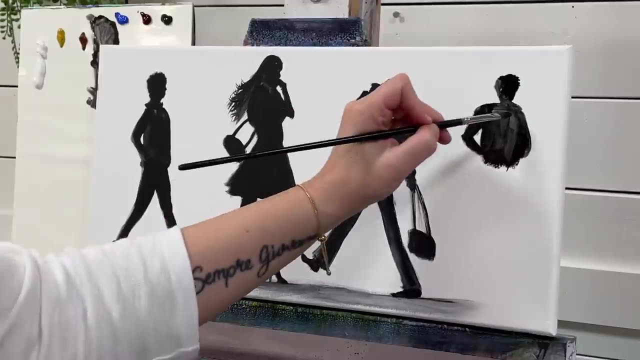 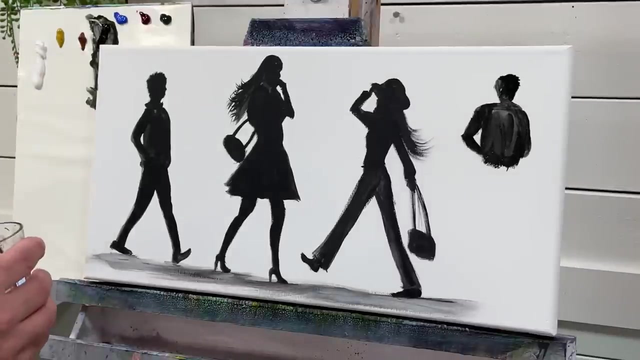 then we're going to leave a little. then we're going to leave a little triangle, triangle, triangle in the middle, there, in the middle, there, in the middle there. a little bit of water again, a little bit of water again, a little bit of water again. i don't want my paint dripping, i just 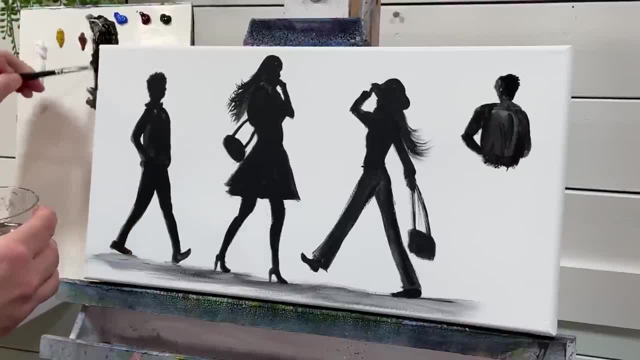 i don't want my paint dripping. i just i don't want my paint dripping, i just want to add a bit of water. so want to add a bit of water. so want to add a bit of water so my paint stays nice and wet and a little. 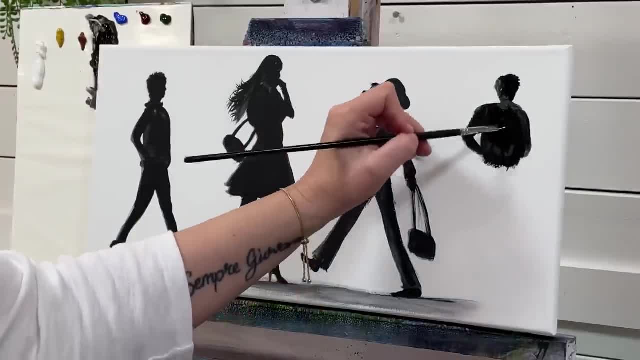 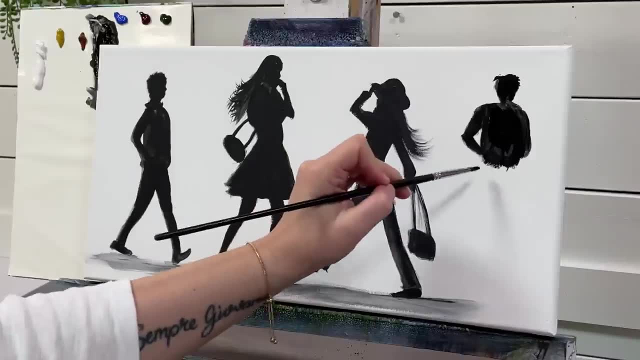 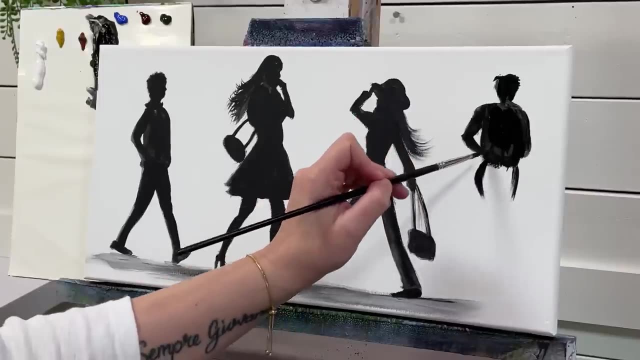 my paint stays nice and wet and a little. my paint stays nice and wet and a little bit more fluid, okay, and then we're going to come out. okay, and then we're going to come out. okay, and then we're going to come out here a little bit. 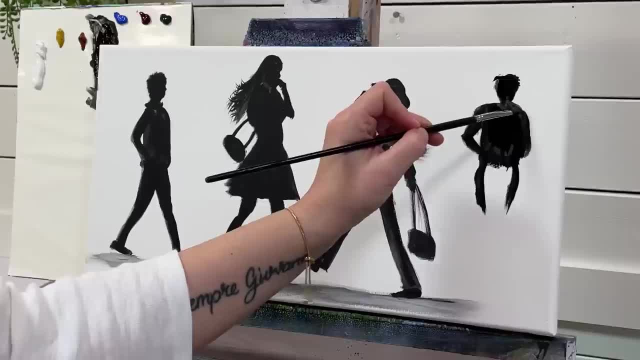 here a little bit, here a little bit. pull it in like this, pull it in like this, pull it in like this. so you've got a, let's look at it into. so you've got a, let's look at it into. so you've got a, let's look at it into shape, as it would be as a shape. 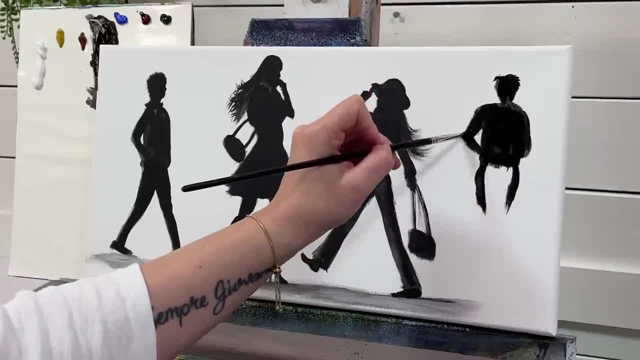 shape as it would be as a shape. shape as it would be as a shape. rectangle here, rectangle here, rectangle here, wider here, wider here, wider here, turn narrow. we've got a turn narrow. we've got a turn narrow. we've got a little triangle in there, little triangle in there. 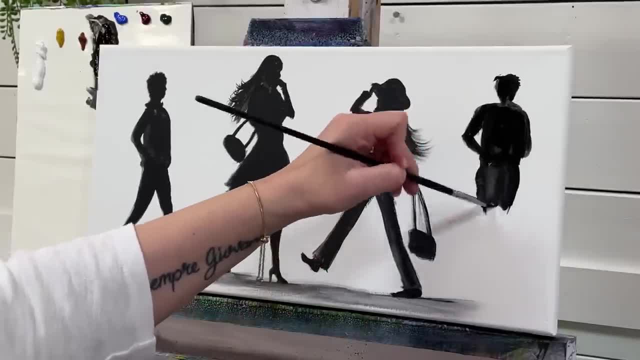 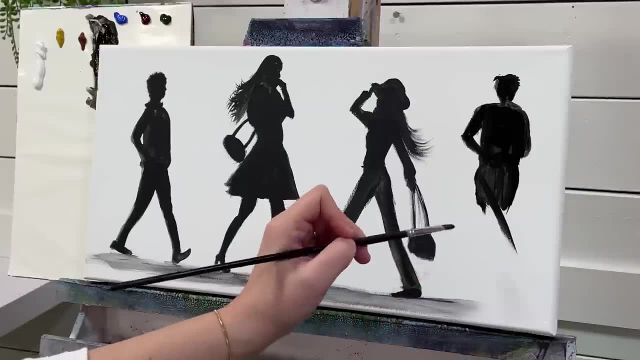 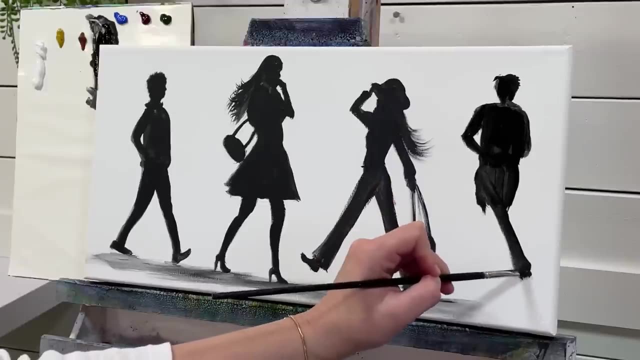 little triangle in there, and and, and we're going to paint this, we're going to paint this, we're going to paint this in, and then we're going to pull over, and then we're going to pull over, and then we're going to pull over- make the pant leg. 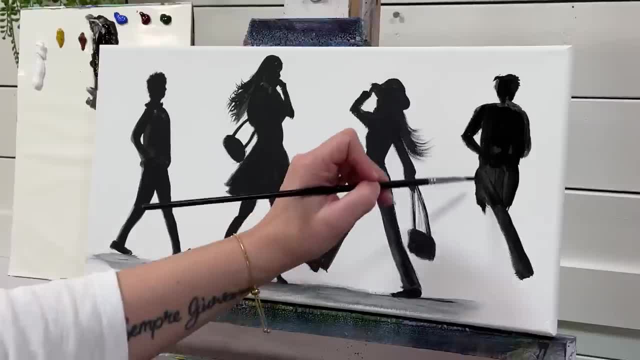 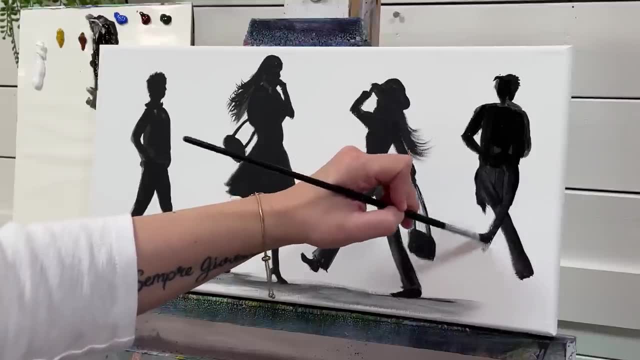 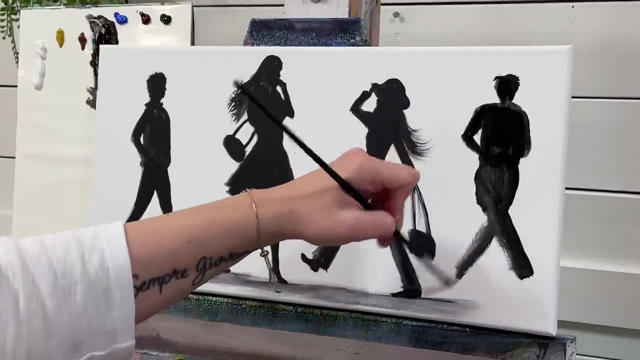 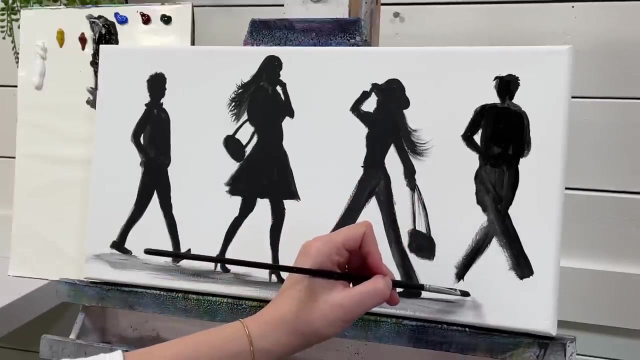 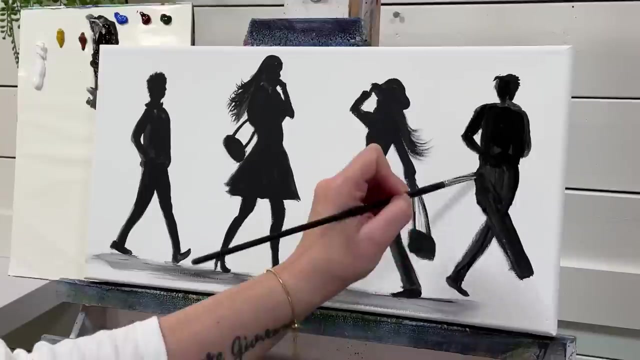 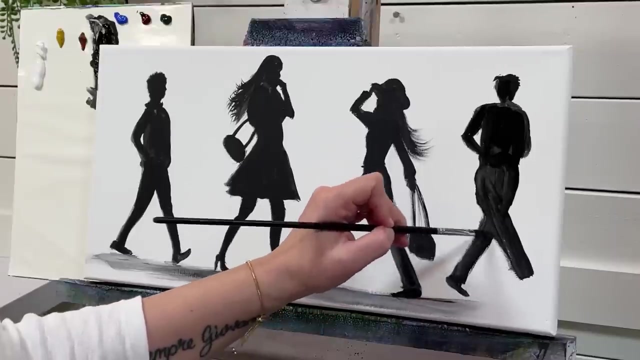 make the pant leg, make the pant leg wider right here, then we're going to pull this way, point, point, point, point point. for the end of the shoe, the front of the. for the end of the shoe, the front of the. for the end of the shoe, the front of the shoe, scoop up. 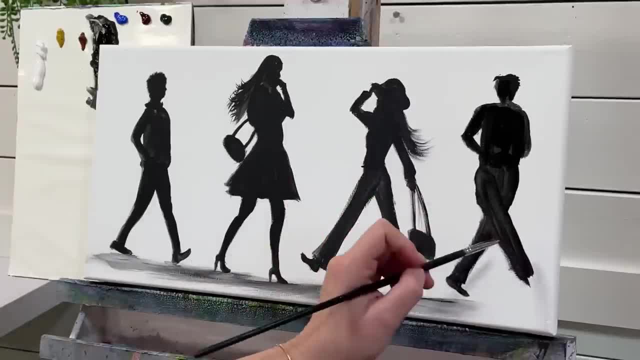 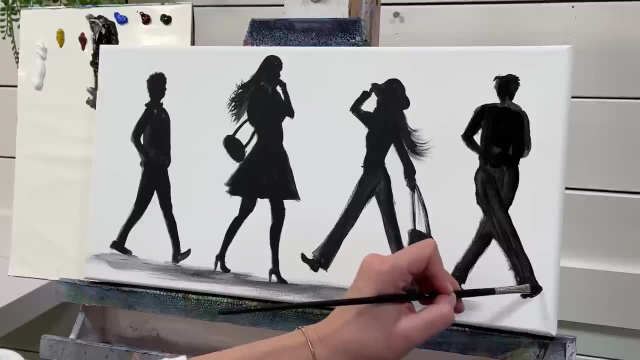 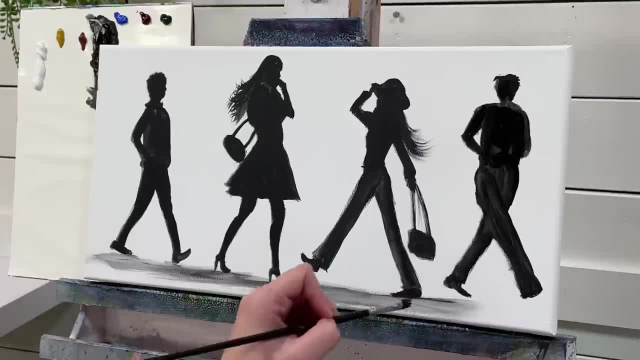 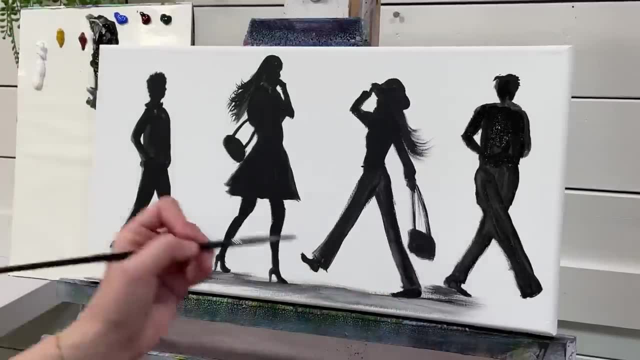 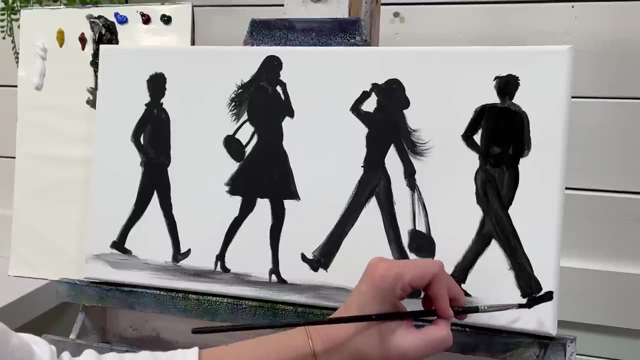 i'm going to give him a little bit more. i'm going to give him a little bit more of a heel here on his, of a heel here on his, of a heel here on his back- shoe there, back, shoe there, back, shoe there, and then pull across. 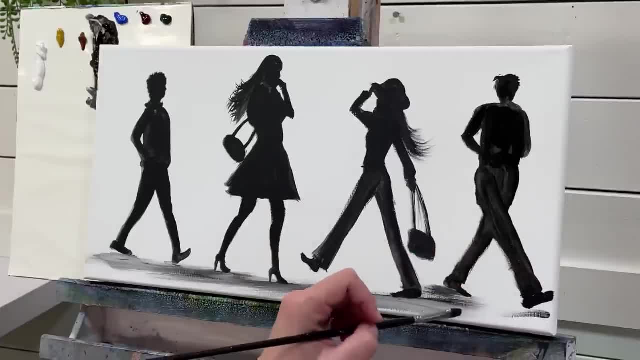 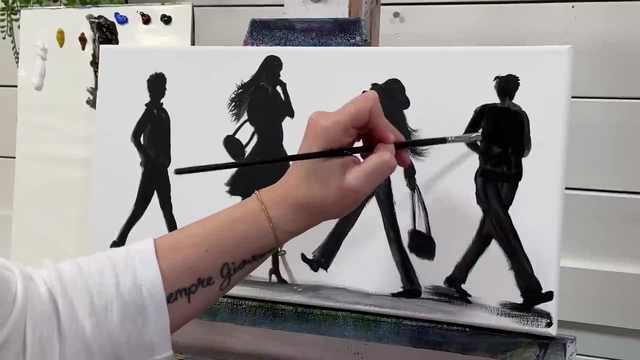 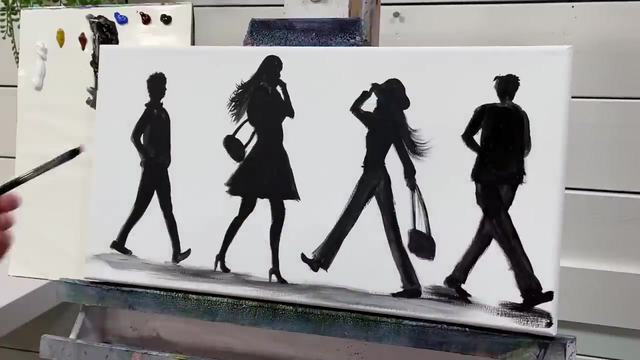 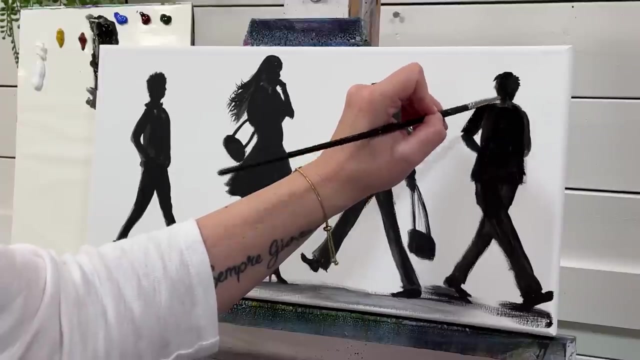 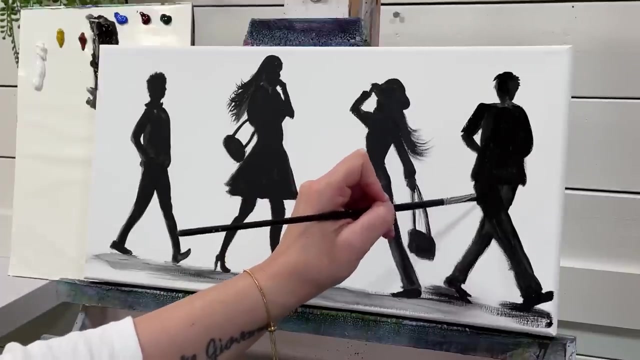 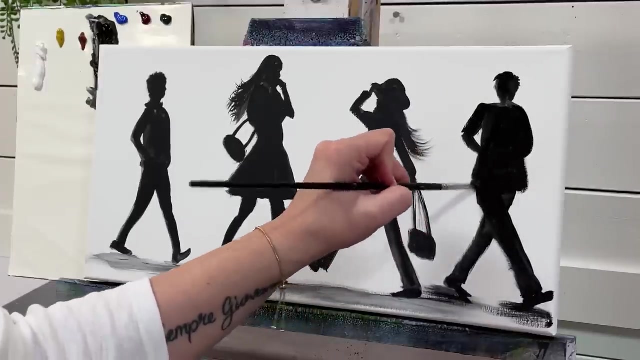 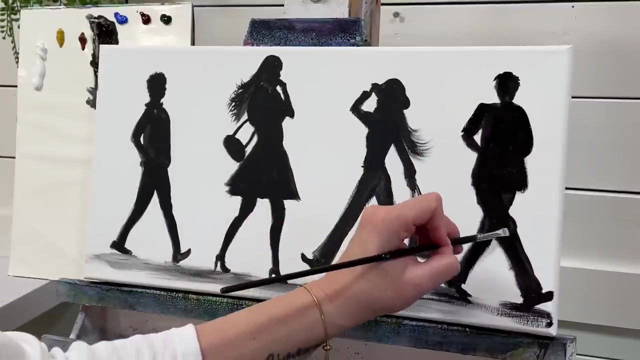 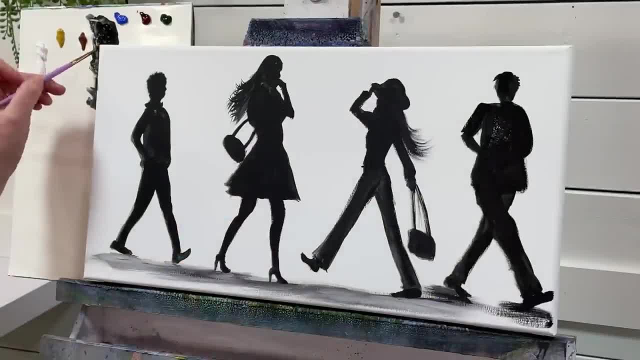 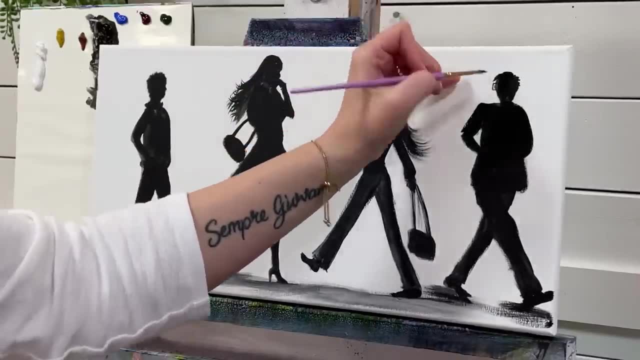 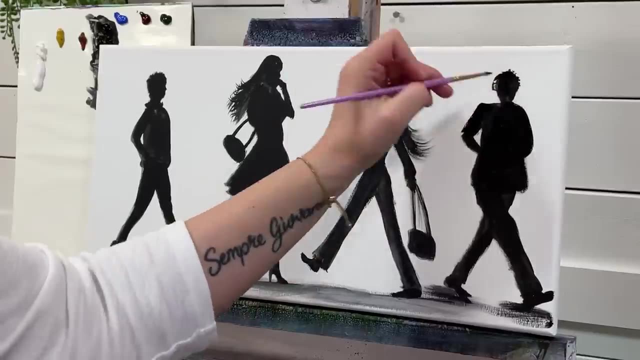 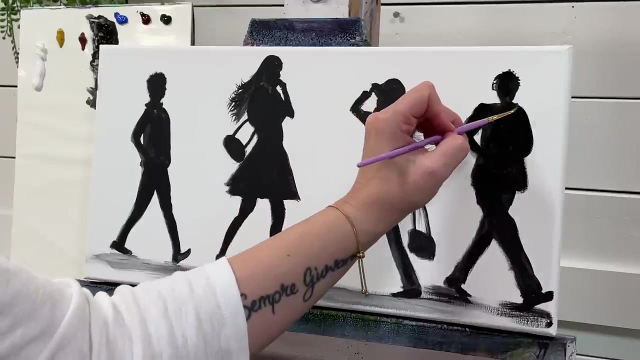 now i'm going to bring his coat down. i'm going to take my round brush a. i'm going to take my round brush a. i'm going to take my round brush a little bit of black. i'll add indication of indication of indication of some glasses here that he's wearing. 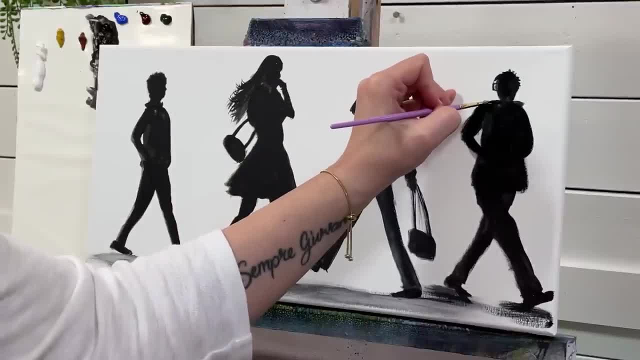 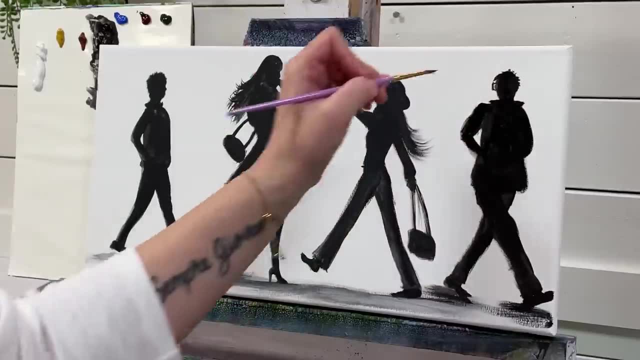 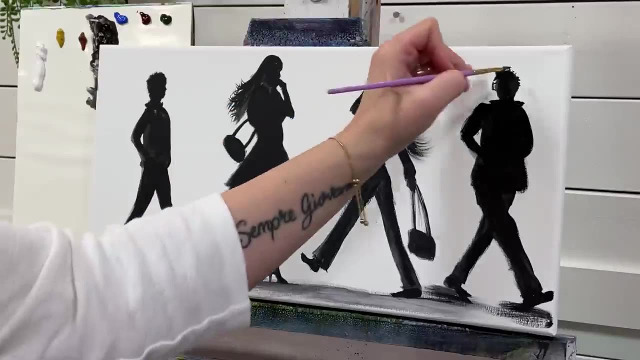 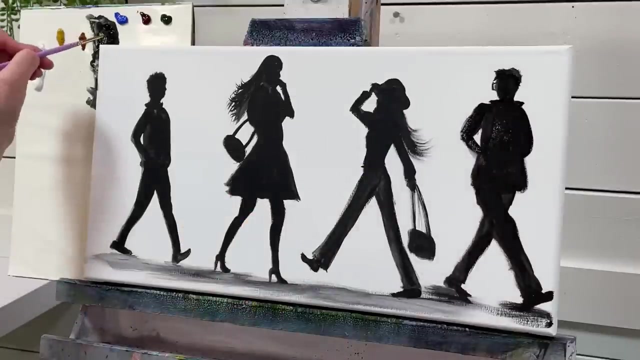 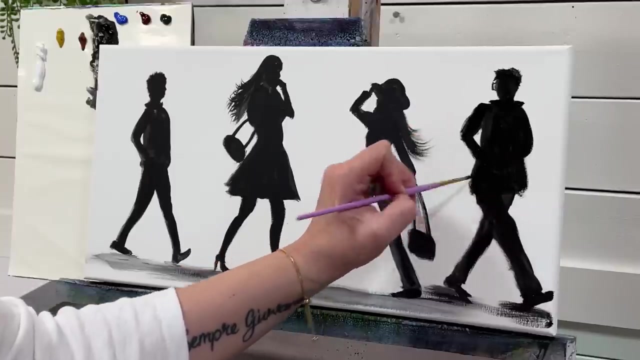 a little, a little. a little collar back there again, a little collar back there again. just bring it on into a little point. just bring it on into a little point. just bring it on into a little point. and a point there and a point there again. just bring it on into a little point there. 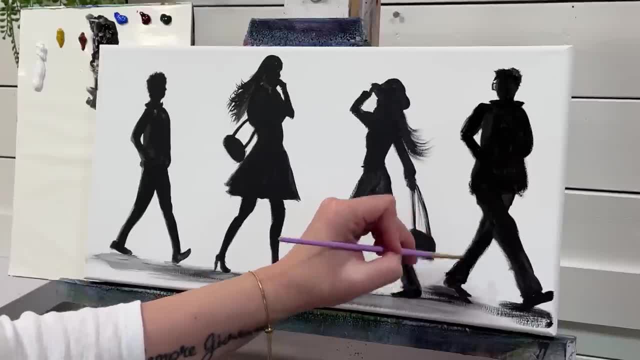 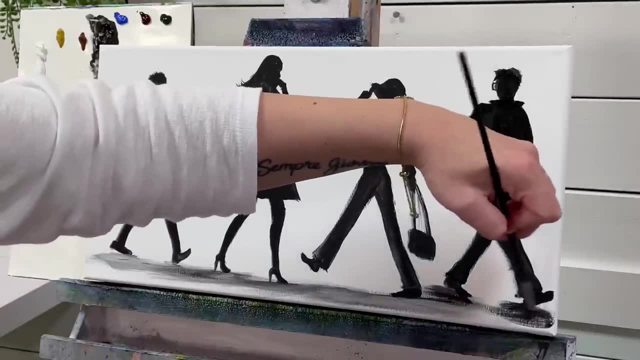 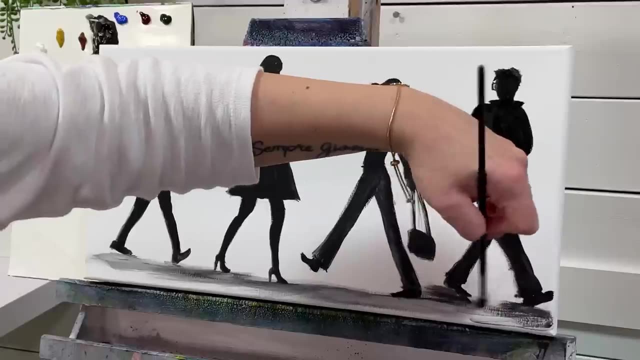 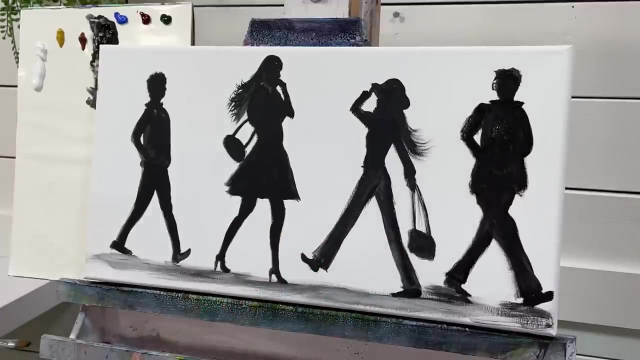 and a point there again. just bring it on into a little point there. and a point there again. just bring it on into a little point there. i'm just going to soften, i'm just going to soften, i'm just going to soften these shadows a little bit down here. okay, so i'm going to use my filbert. okay, so i'm going to use my filbert. okay, so i'm going to use my filbert, brush, brush, brush, and i'm going to take a little bit, and i'm going to take a little bit. 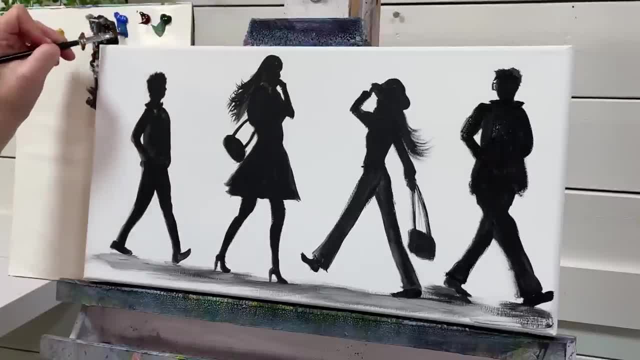 and i'm going to take a little bit of blue, a little bit of white and a of blue, a little bit of white and a of blue, a little bit of white and a little bit of sap green, little bit of sap green, little bit of sap green. and i'll just add this: 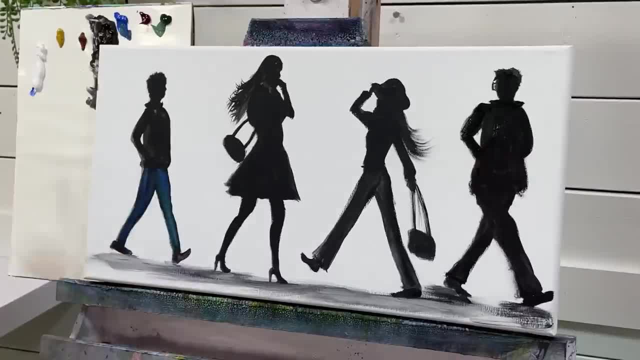 here over the pants, so you can just have here over the pants, so you can just have here over the pants. so you can just have like a simple, like a simple, like a simple jean or pant and then just add a little jean or pant and then just add a little. 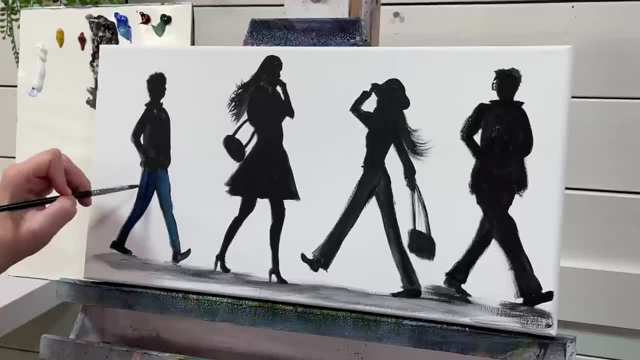 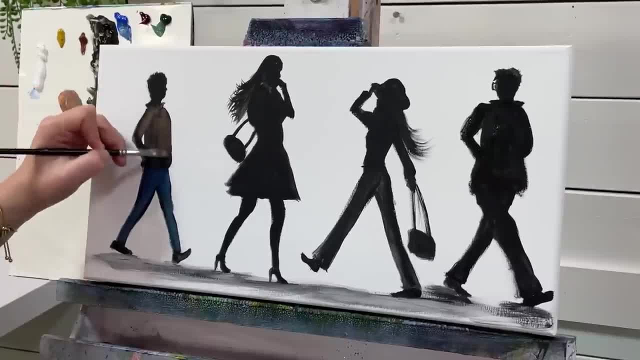 and give them sort of a tan colored and give them sort of a tan colored coat. try to not make it solid everywhere. so try to not make it solid everywhere. so try to not make it solid everywhere, so that you are left with some, that you are left with some. 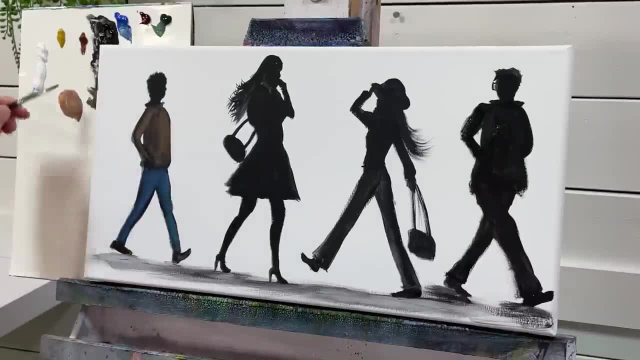 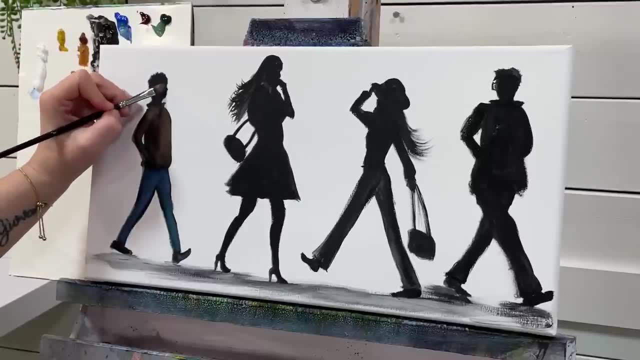 that you are left with some shadows, and i'm going to take a little bit of and i'm going to take a little bit of, and i'm going to take a little bit of yellow ochre burnt sienna, yellow ochre burnt sienna, yellow ochre burnt sienna, and just 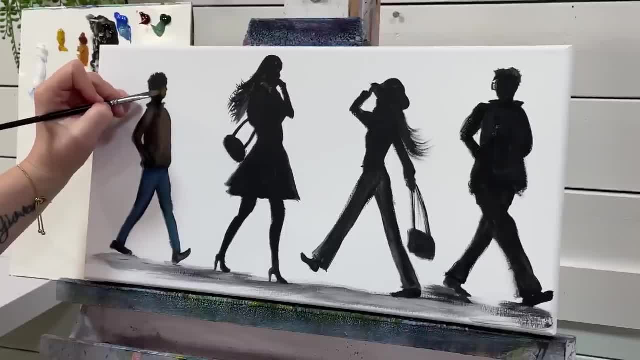 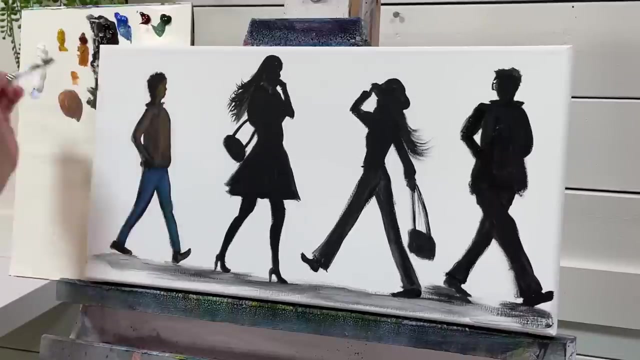 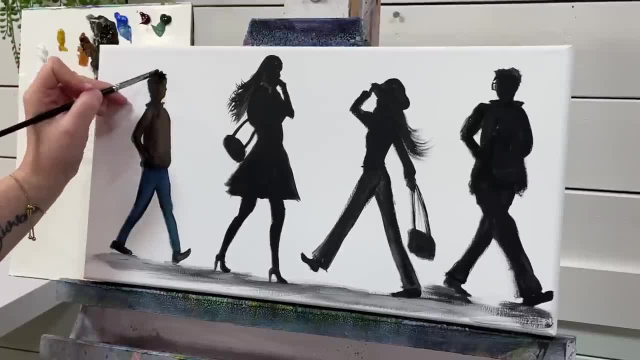 and then a little bit of black burnt, and then a little bit of black burnt. sienna, sienna, sienna, you could leave the hair dark, or you, you could leave the hair dark, or you, you could leave the hair dark, or you could add a little bit of. 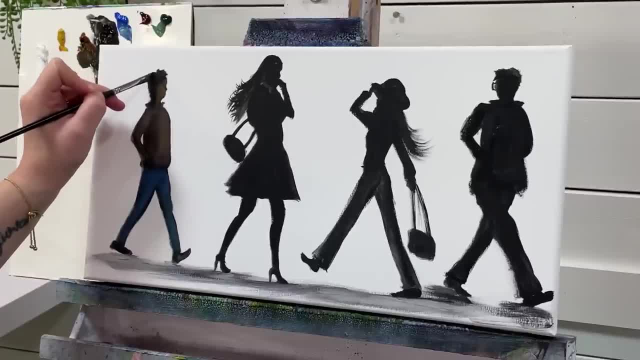 ground to it, or blonde if you wanted. grab a little bit more, grab a little bit more, grab a little bit more. yellow ochre, yellow ochre, yellow ochre. i'm not trying to paint, i'm not trying to paint, i'm not trying to paint the features we're just adding. 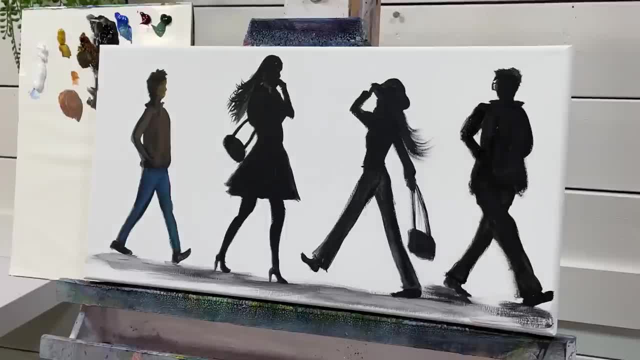 the features. we're just adding the features. we're just adding little suggestions, of little suggestions, of little suggestions of colors for skin here. colors for skin here. colors for skin here: okay, so let's add um some red maybe. okay, so let's add um some red maybe. 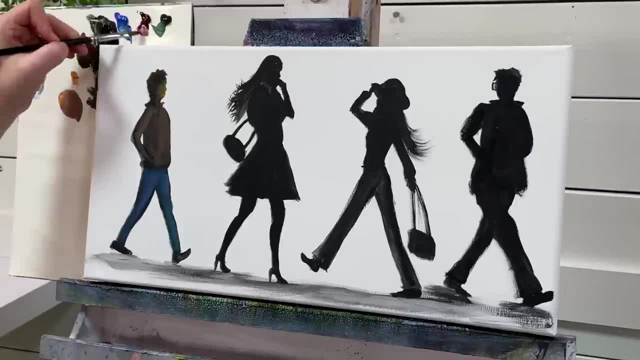 okay. so let's add, um, some red, maybe for her dress, for her dress, for her dress, a little bit of white, a little bit of a little bit of white. a little bit of a little bit of white, a little bit of yellow ochre, yellow ochre. 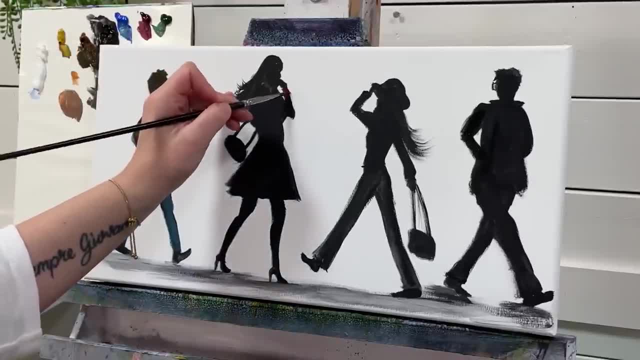 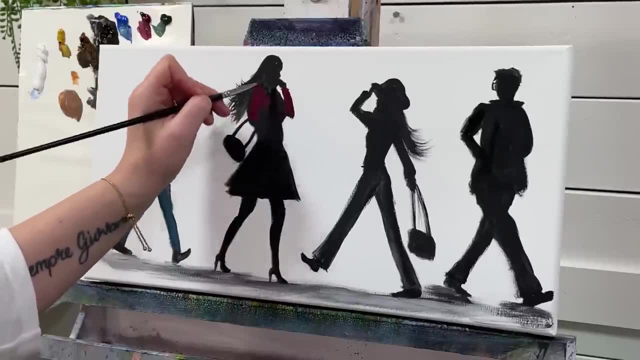 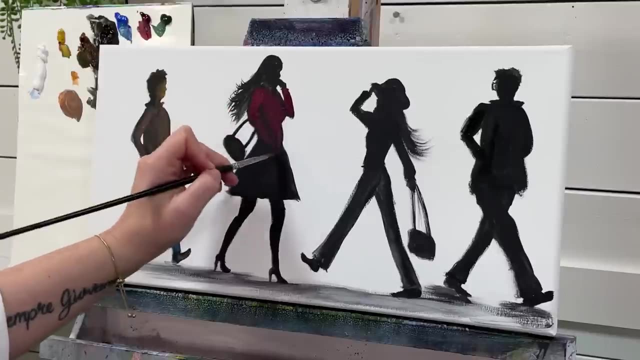 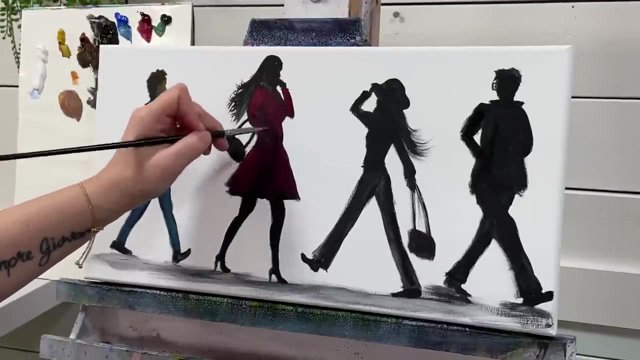 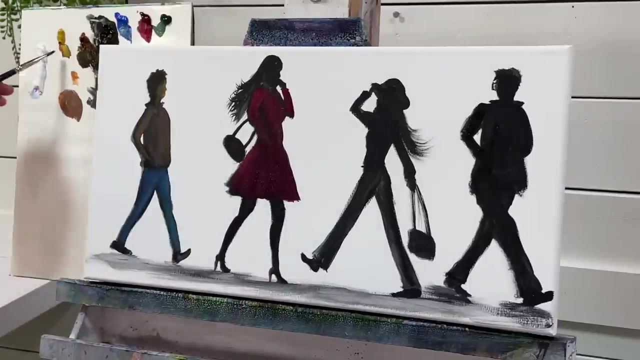 yellow ochre. we can tone it a bit, and we can tone it a bit, and we can tone it a bit and start with start with. start with her cuff here, her cuff here, her cuff here. so you just keep it simple. so you just keep it simple. 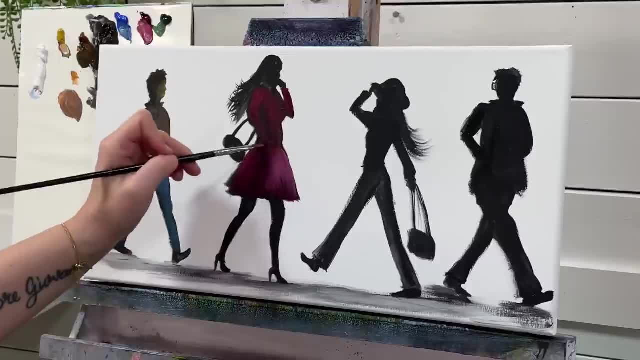 so you just keep it simple, and then a little bit of a, and then a little bit of a, and then a little bit of a. white and yellow ochre in there. white and yellow ochre in there. white and yellow ochre in there, along with the red. 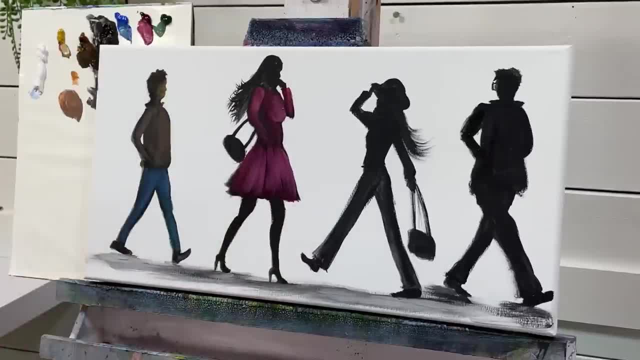 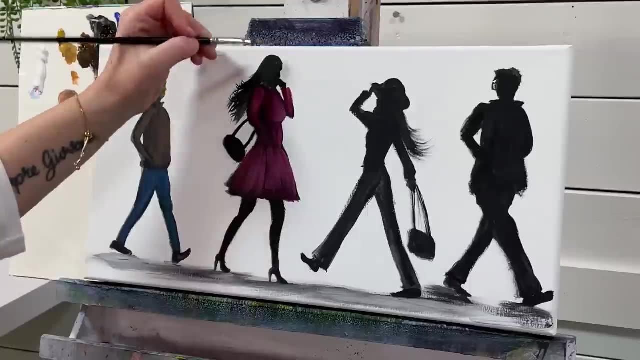 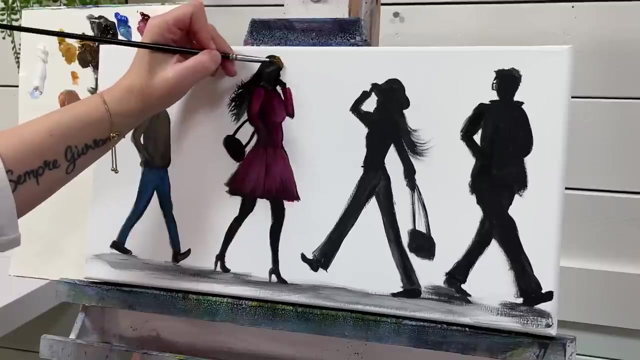 the red, the red. you can use any red you want. and let's uh add some yellow ochre. and let's uh add some yellow ochre. and let's uh add some yellow ochre- burnt sienna to her hair and start at the top here. start at the top here. 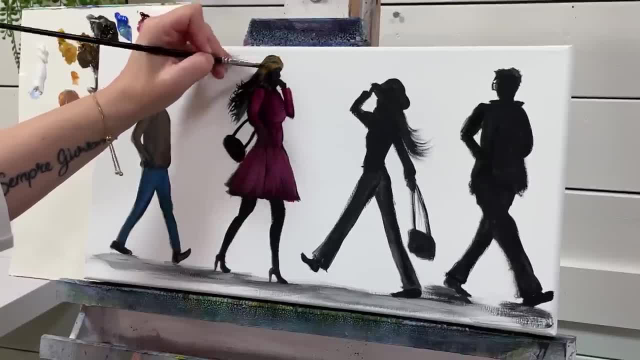 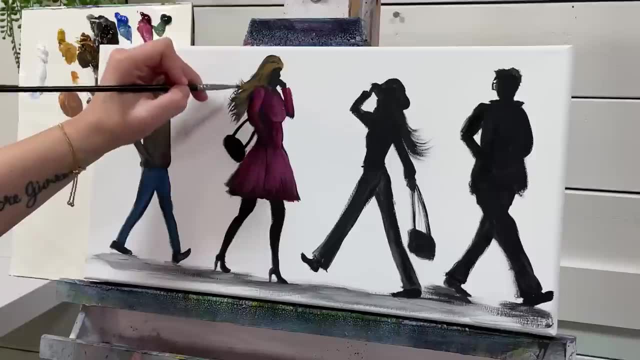 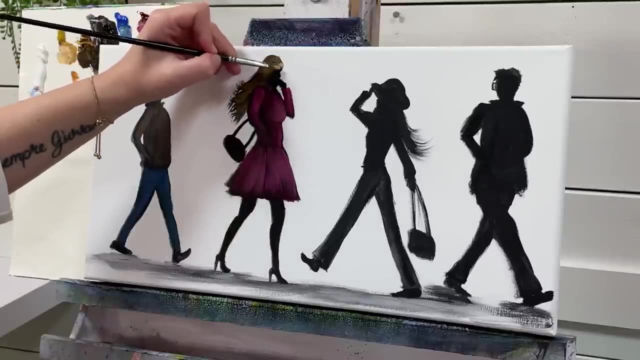 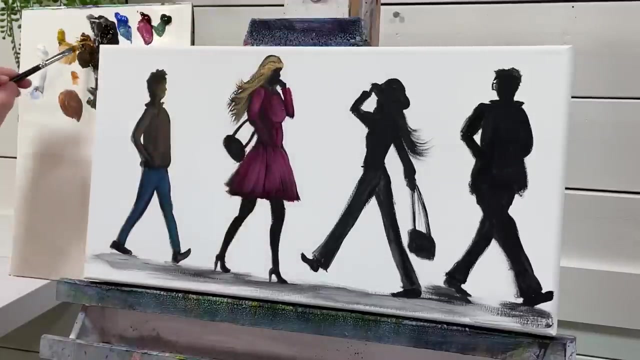 start at the top here, pull and sweep over and add a little bit of white to create that movement, just kind of to create that movement. just kind of to create that movement, just kind of sweep, sweep, sweep. we'll add a little bit of burnt sienna in. 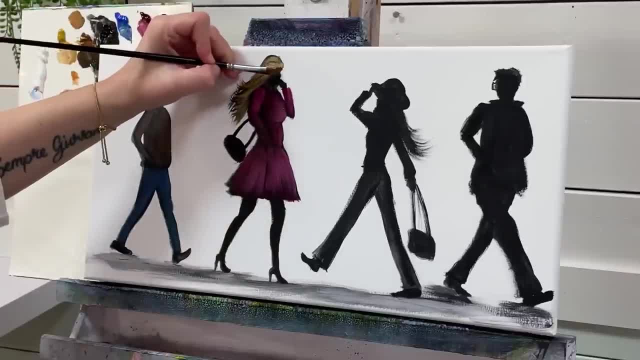 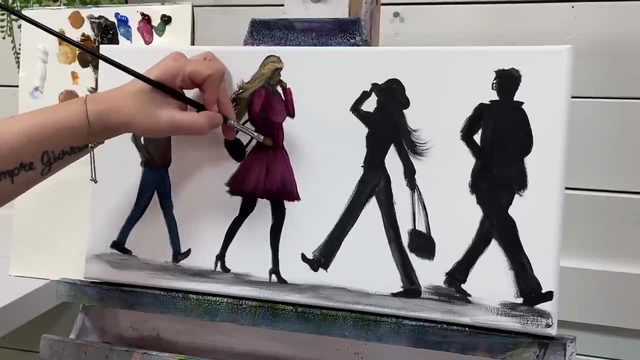 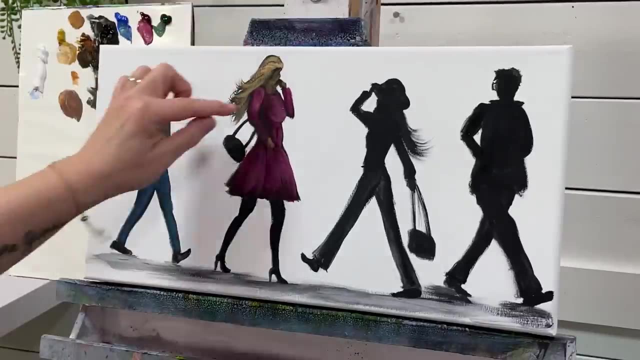 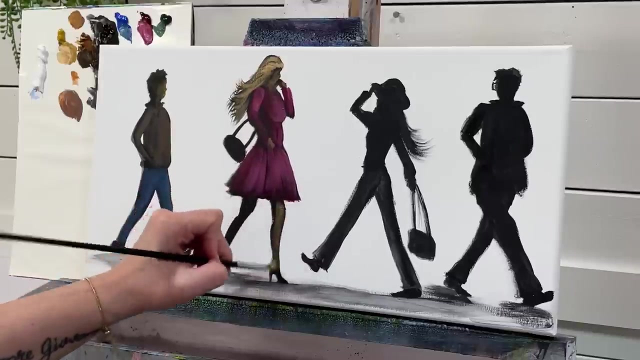 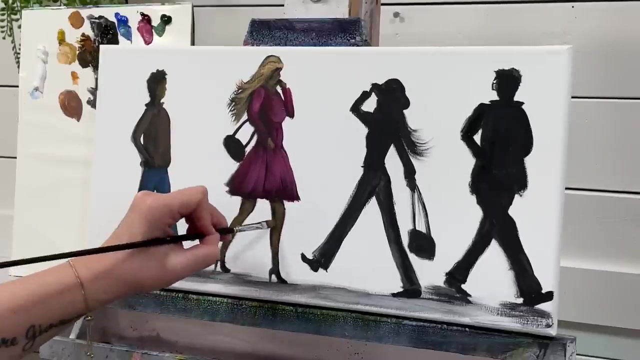 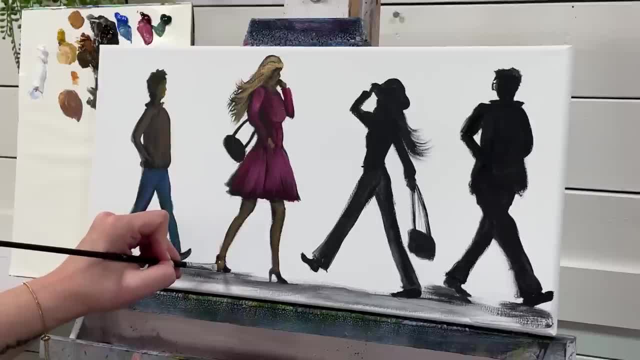 keep it darker right under the dress, or keep it darker right under the dress or the skirt and then bring it down just a little bit. and then bring it down just a little bit, and then bring it down just a little bit for, for, for the top, on the top of the shoes. 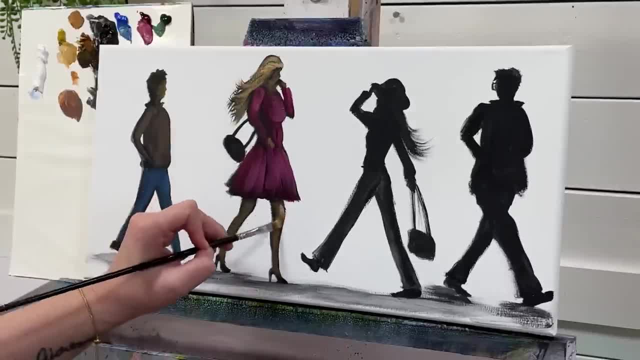 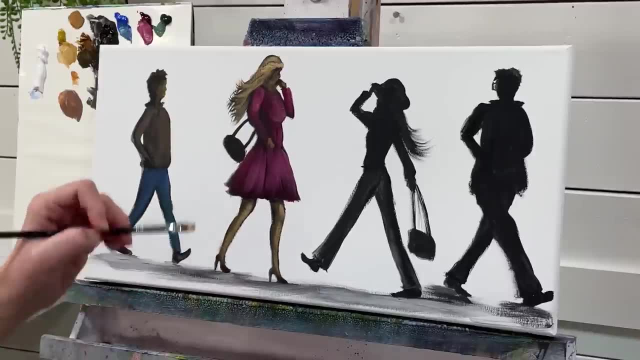 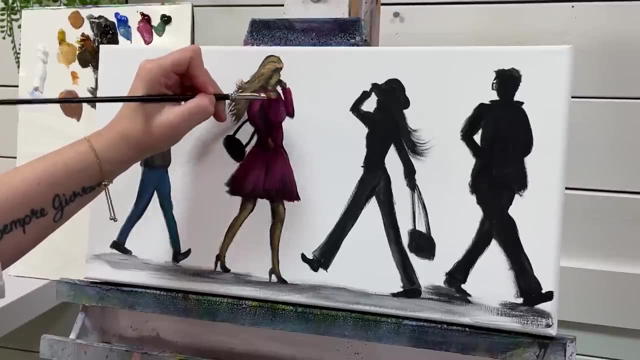 and then add just a little bit more of, and then add just a little bit more of, and then add just a little bit more of the yellow ochre, the yellow ochre, the yellow ochre. okay, let's go over here and let's add. okay, let's go over here and let's add. 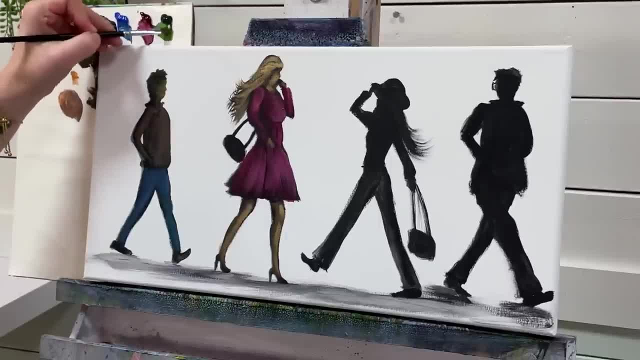 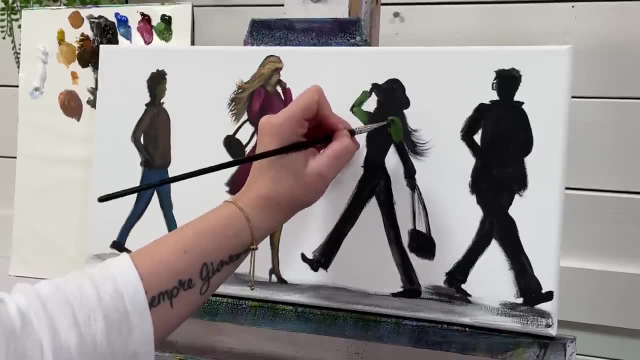 okay, let's go over here and let's add some green, a little bit of white, some green a little bit of white, some green a little bit of white. so black or white is up to you, it's up to you. so black or white is up to you, it's up to you. so black or gray scale is a really great. 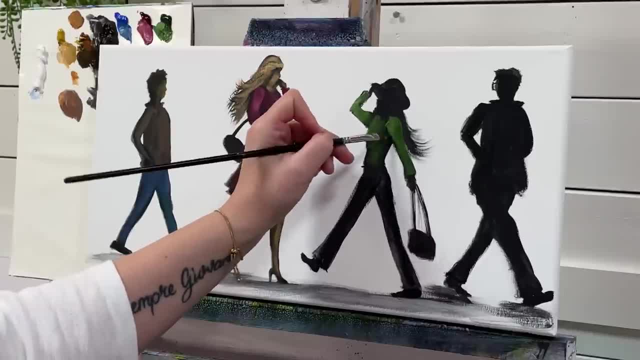 so black or gray scale is a really great. so black or gray scale is a really great. base coat, base coat, base coat. i'm leaving a little darker in between. i'm leaving a little darker in between. i'm leaving a little darker in between her, her, her arm there and her waist. bring it out. 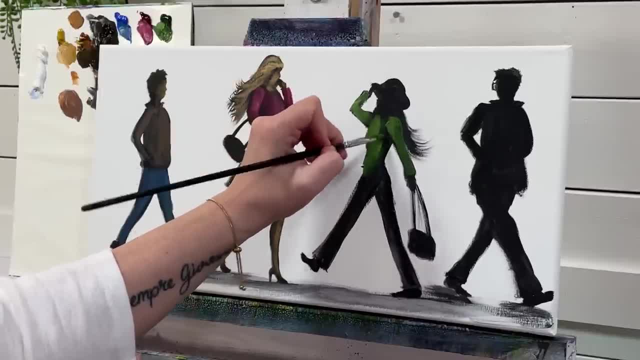 arm there and her waist bring it out. arm there and her waist bring it out here. so it's going to be here. so it's going to be here, so it's going to be a little brighter right here and then a little brighter right here and then. 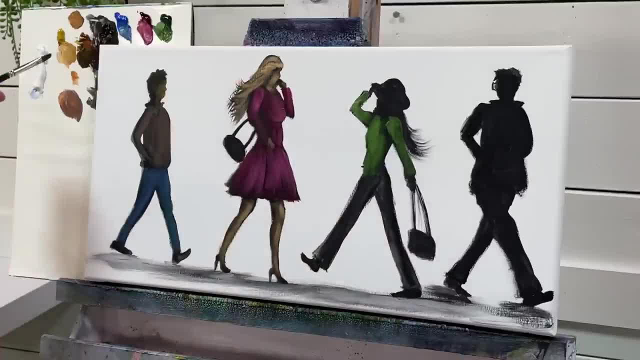 a little brighter right here and then more in shadow there. i think i want to keep her pants black. i think i want to keep her pants black. i think i want to keep her pants black. though i'm just going to go over with, though i'm just going to go over with. 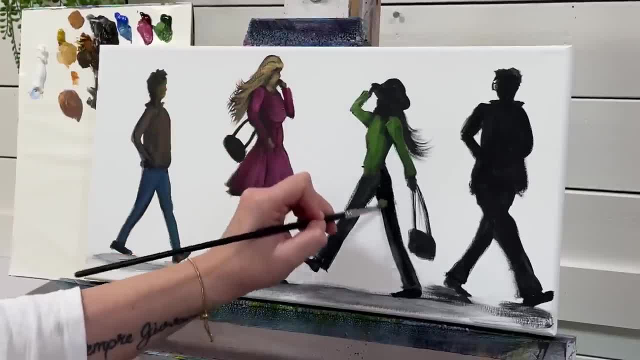 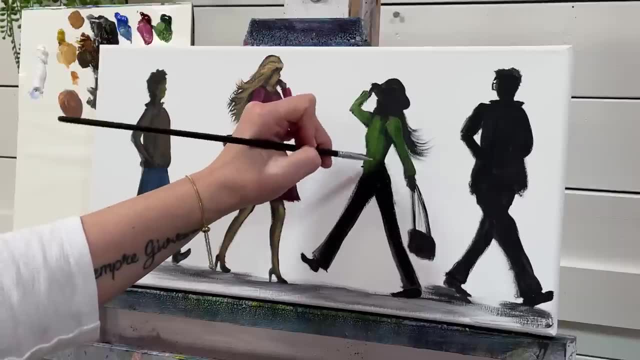 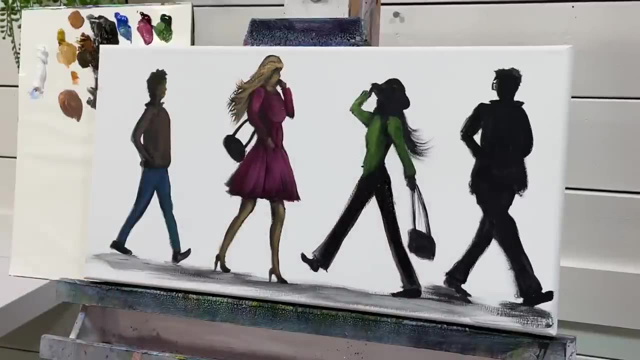 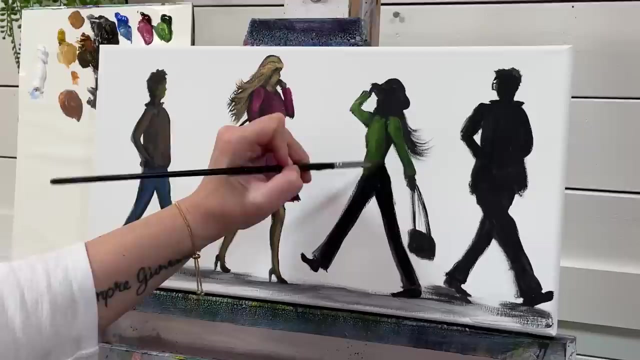 though i'm just going to go over with extra black. rinse my brush out periodically here. rinse my brush out periodically here. rinse my brush out periodically here just to make sure it's nice and clean. those paint colors aren't nice and clean. those paint colors aren't. 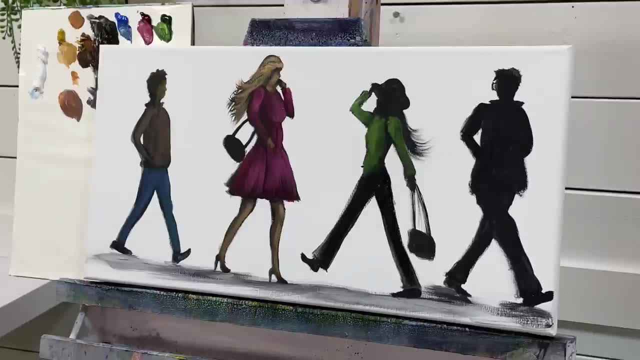 nice and clean. those paint colors aren't building up in my brush. building up in my brush. building up in my brush: okay, let's just add a little bit of. okay, let's just add a little bit of. okay, let's just add a little bit of white and yellow ochre. 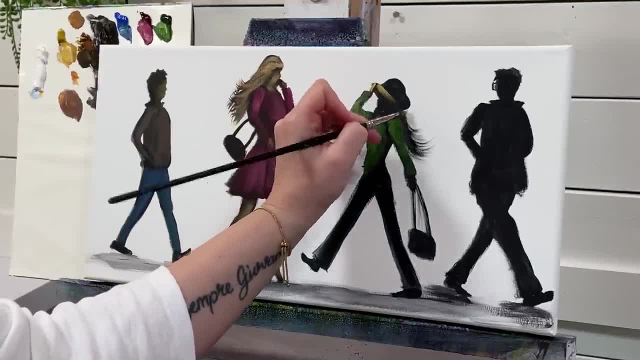 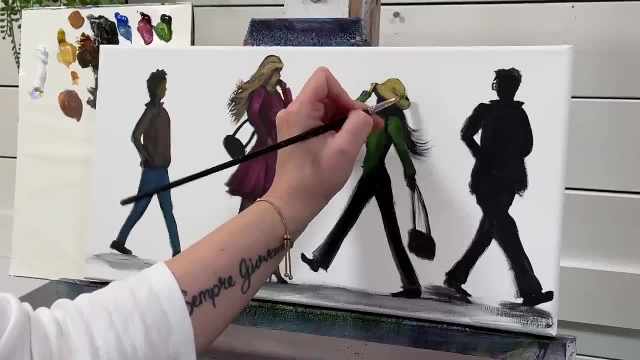 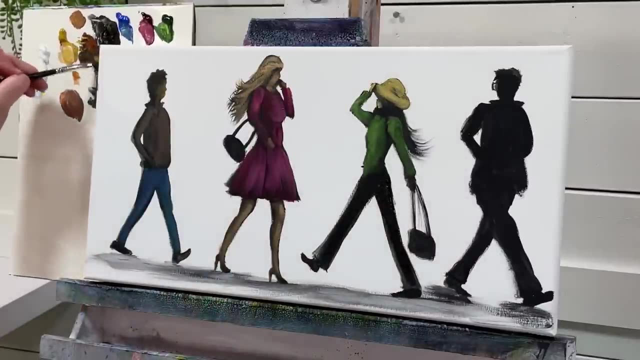 white and yellow ochre- white and yellow ochre- to our hand, grabbing her hat there. and then we can take some burnt sienna, and then we can take some burnt sienna, and then we can take some burnt sienna, and we'll have her hair, and we'll have her hair. 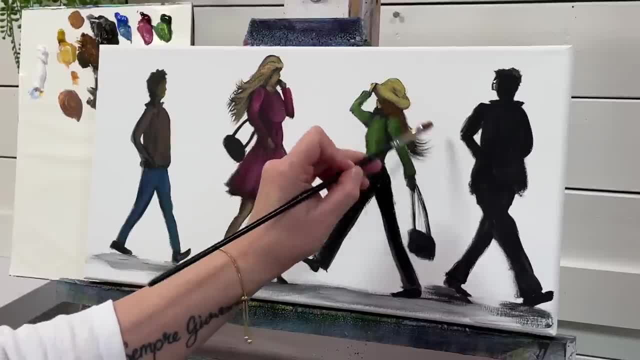 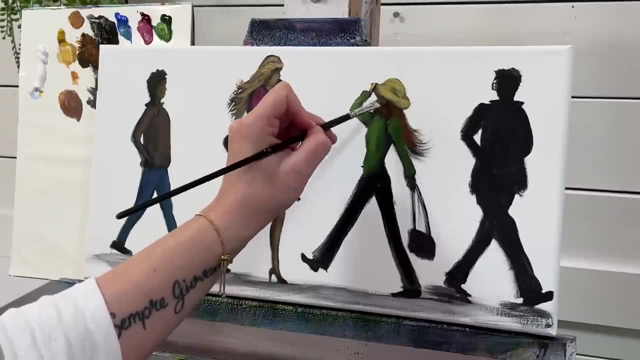 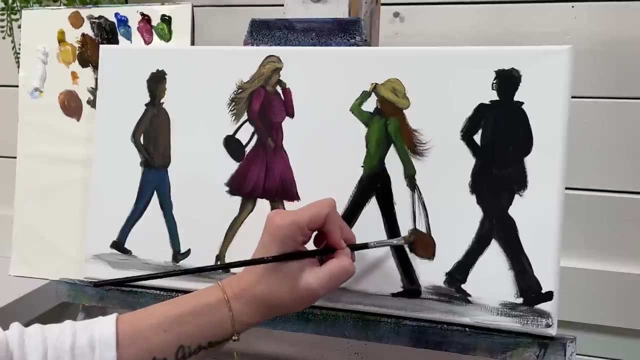 and we'll have her hair coming down, coming down, coming down over her shoulder, and let's give her a brown brown leather bag here, and let's give her a brown brown leather bag here, and let's give her a brown brown leather bag here. so a little bit of burnt sienna. 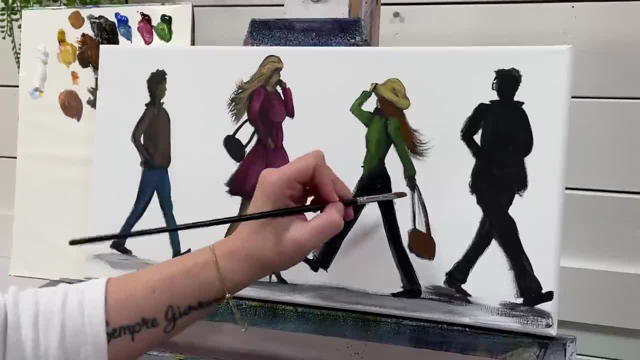 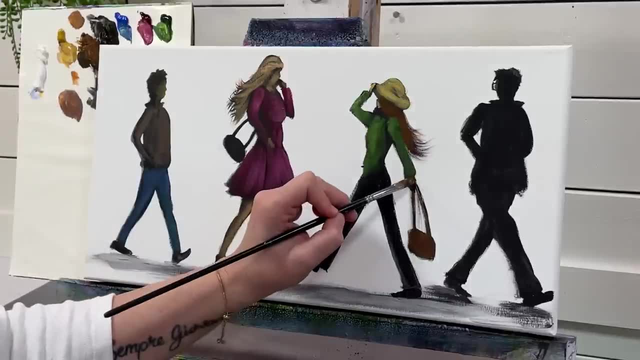 so a little bit of burnt sienna. so a little bit of burnt sienna again, and just a little bit here again and just a little bit here again, and just a little bit here on the handles, and then a little on the handles and then a little. 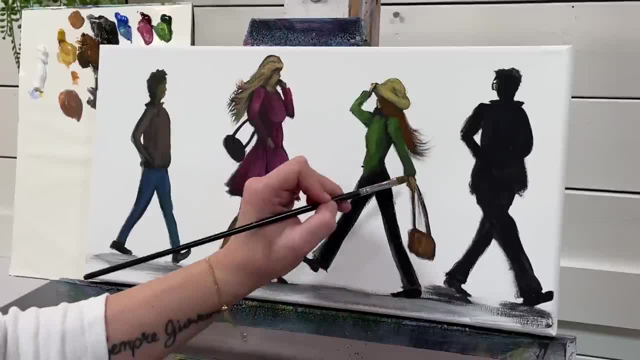 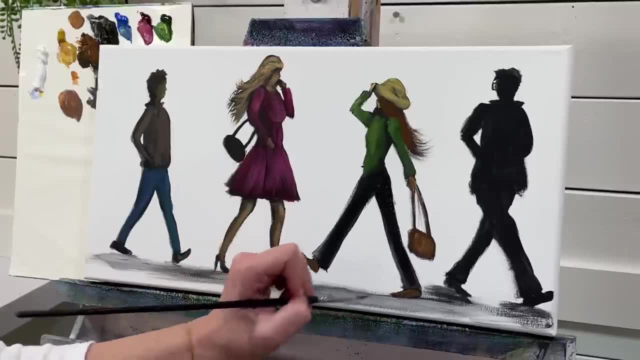 on the handles and then a little dab of yellow ochre, dab of yellow ochre, dab of yellow ochre for her hand there. and we could add this to her feet as well. i don't. and we could add this to her feet as well. i don't. 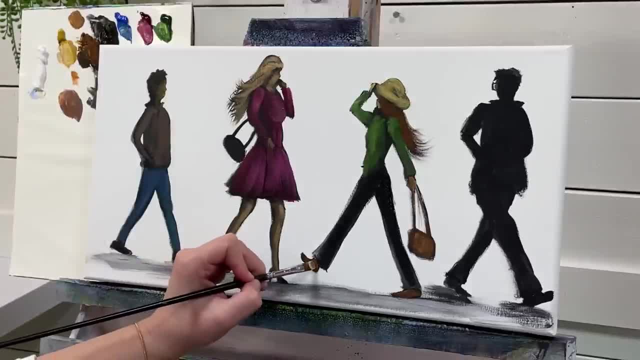 and we could add this to her feet as well. i don't think she's wearing shoes. think she's wearing shoes. think she's wearing shoes, it's kind of something. it's kind of something. it's kind of something interesting to add if you were wanting. interesting to add, if you were wanting. 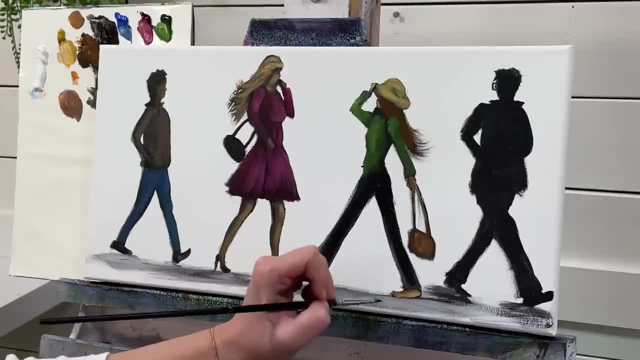 interesting to add if you were wanting to paint, to paint, to paint a figure like walking on a path or a. a figure like walking on a path or a. a figure like walking on a path or a field and like just a more field and like just a more. 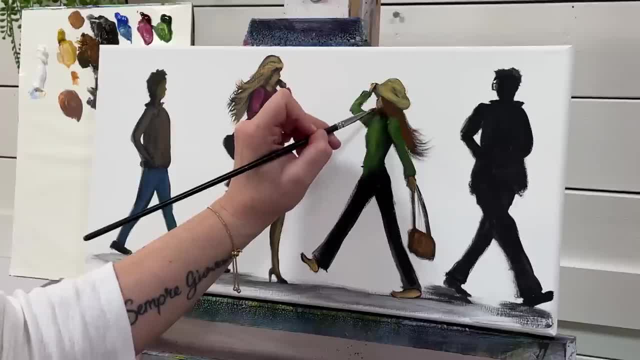 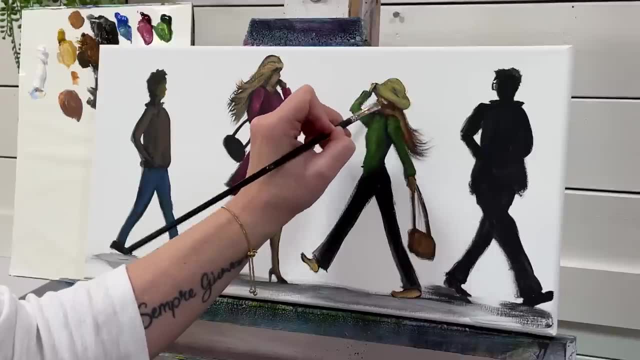 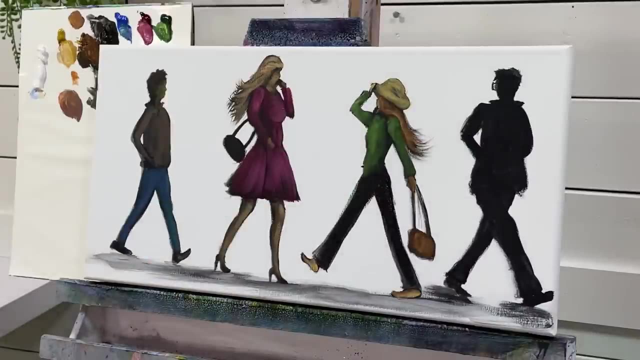 field and like just a more natural setting. so i think it's you're learning a lot. so i think it's you're learning a lot. so i think it's you're learning a lot today about figure painting and how you today about figure painting and how you. 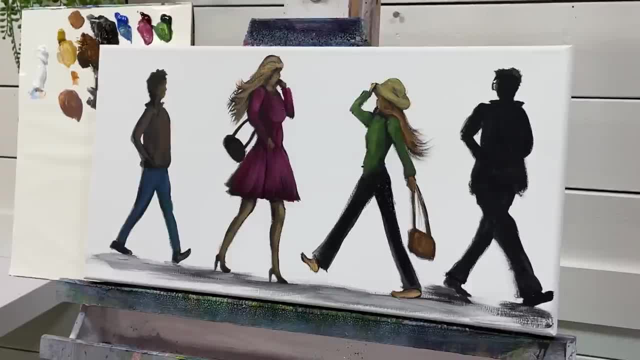 today about figure painting and how you don't have to have, don't have to have, don't have to have all the details of their limbs, all the details of their limbs, all the details of their limbs: fingers, toes, fingers, toes, fingers, toes, um, um, um, and and. 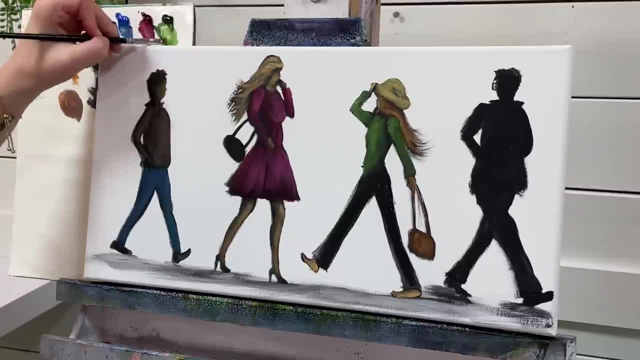 and their faces, their faces, their faces, to be able to paint them and add them, to be able to paint them and add them, to be able to paint them and add them. and this is just like for beginners, right? and this is just like for beginners, right? and this is just like for beginners, right. maybe you want to. 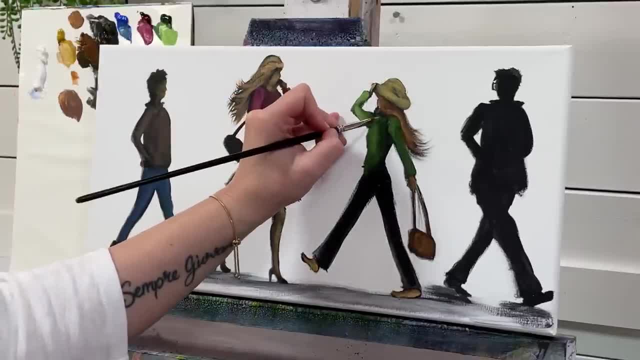 maybe you want to. maybe you want to add a little bit of extra white to the. add a little bit of extra white to the. add a little bit of extra white to the green here. maybe you want to add green here. maybe you want to add green here. maybe you want to add all those details and some of your. 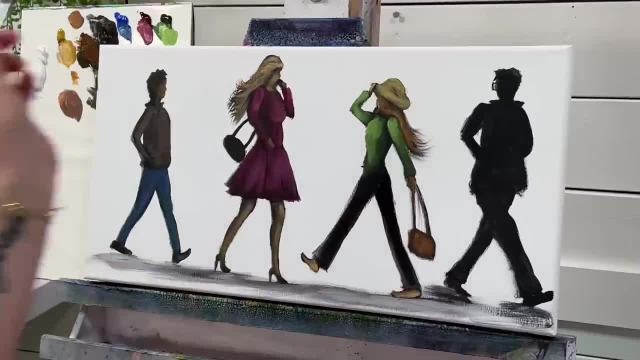 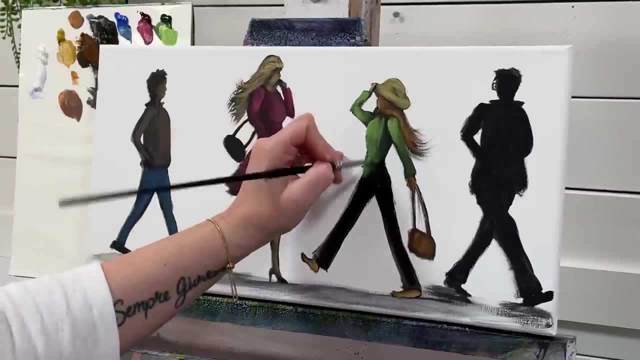 all those details and some of your, all those details and some of your paintings, and you definitely can but this paintings and you definitely can but this paintings and you definitely can, but this tutorial is just meant to be for tutorial is just meant to be for tutorial is just meant to be for um beginners. 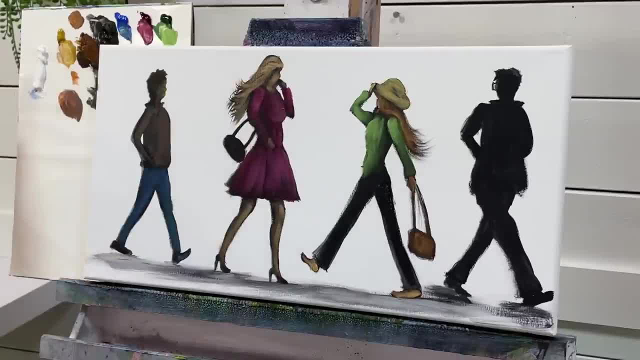 okay, let's work on um this guy over here. okay, let's work on um this guy over here. okay, let's work on um this guy over here. so i'm gonna give him, so i'm gonna give him, so i'm gonna give him. let's make some purple, we'll mix it up. 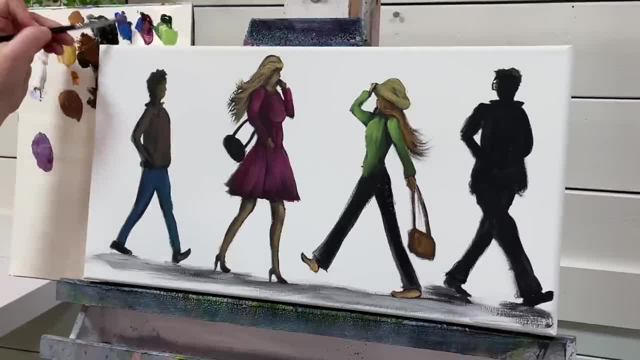 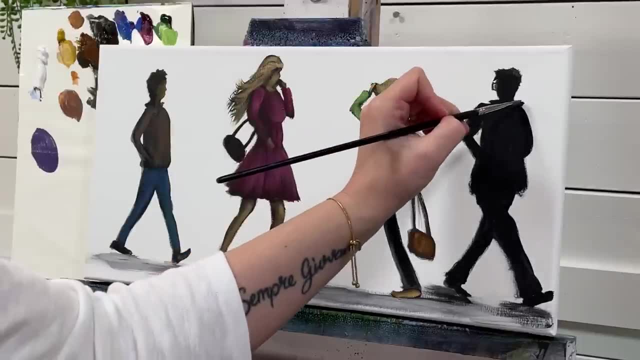 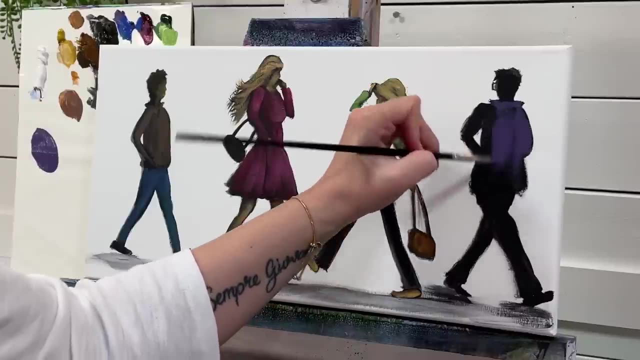 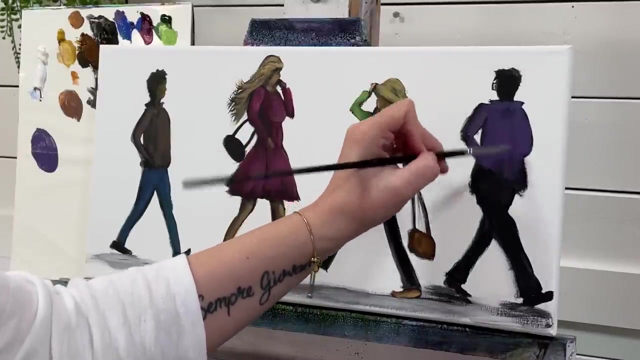 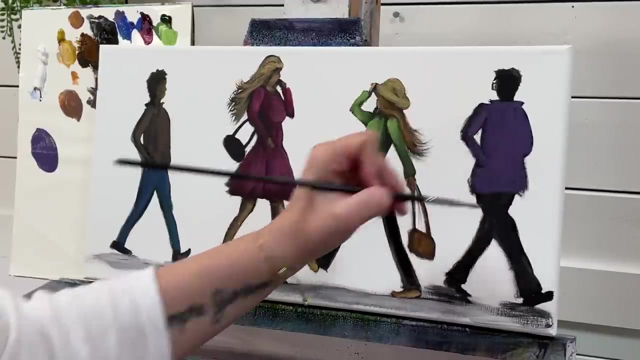 let's make some purple, we'll mix it up. let's make some purple, we'll mix it up over here. a little bit of white crimson and the blue, we'll make more of a purple jacket. white crimson and the blue: we'll make more of a purple jacket. 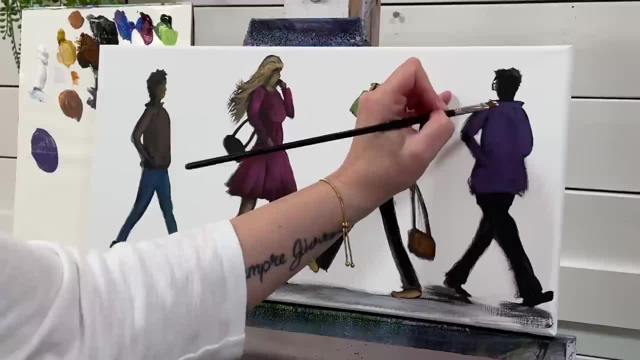 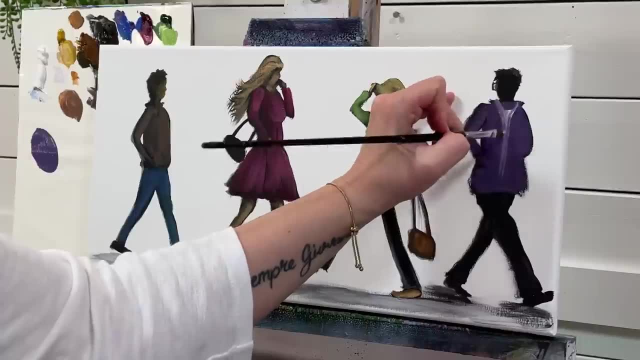 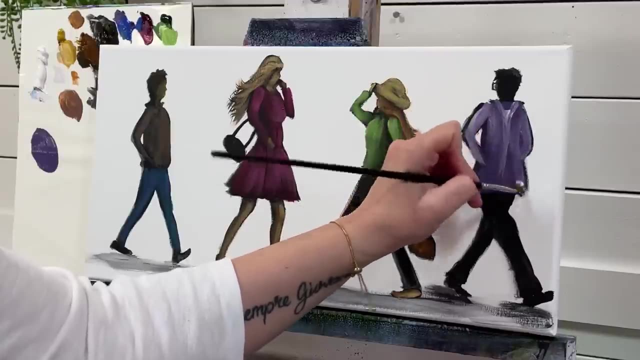 then i'm going to come down in the front, then i'm going to come down in the front, then i'm going to come down in the front with a little bit of white, with a little bit of white, with a little bit of white. take a little bit of burnt sienna yellow. 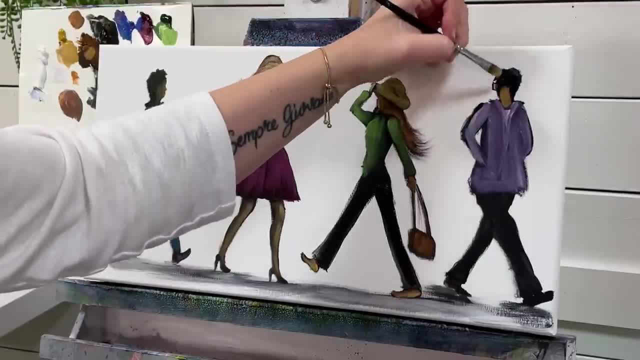 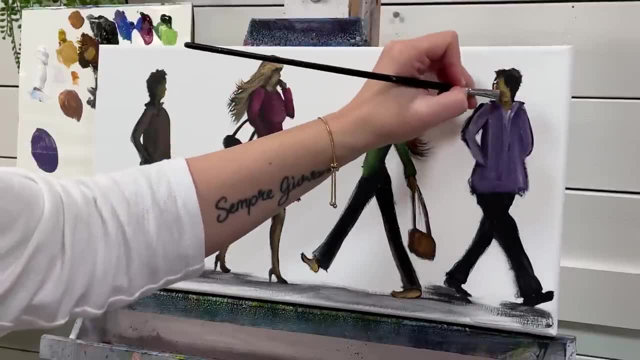 take a little bit of burnt sienna yellow. take a little bit of burnt sienna yellow, ochre, ochre, ochre and white. so this is the front, but he's turning. so this is the front, but he's turning. so this is the front, but he's turning his head. 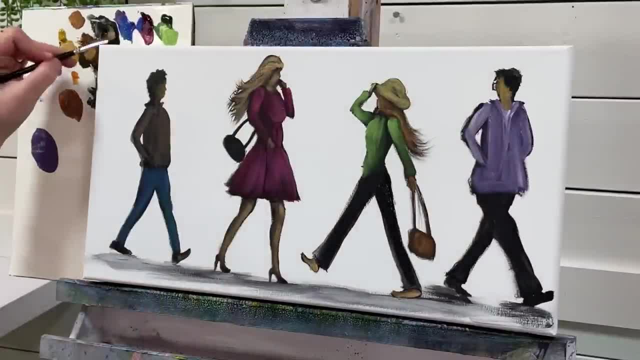 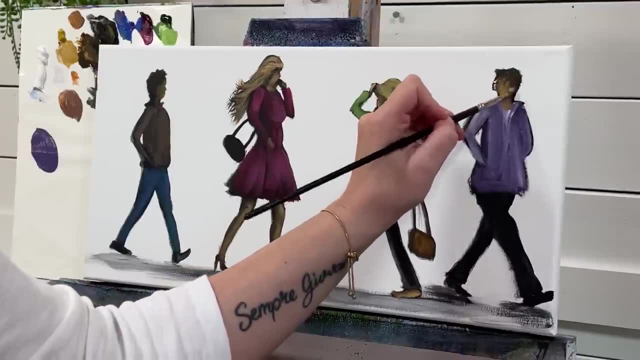 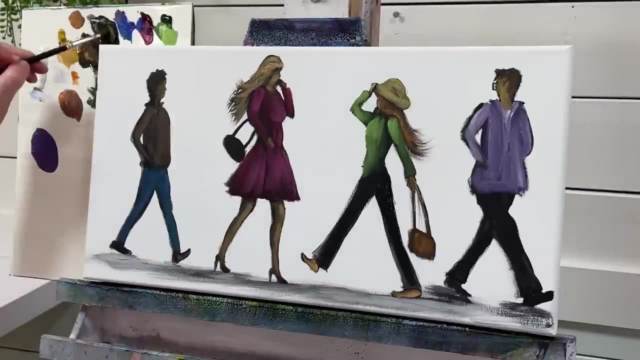 his head, his head to look at something. maybe that girl to look at something. maybe that girl to look at something, maybe that girl. so i'm going to add a little bit of, so i'm going to add a little bit of, so i'm going to add a little bit of black to. 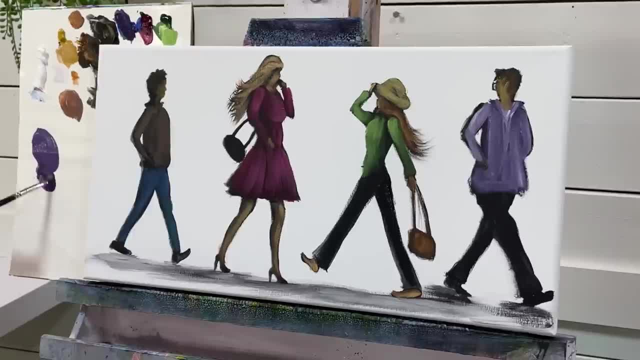 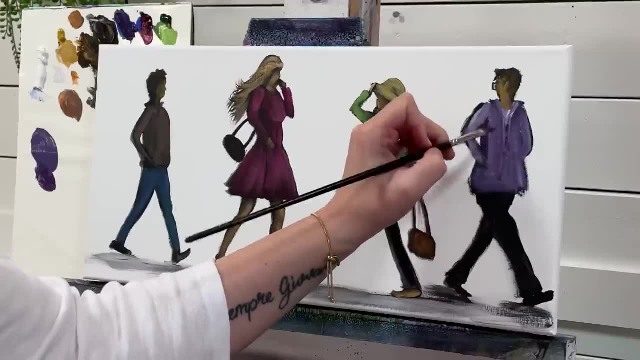 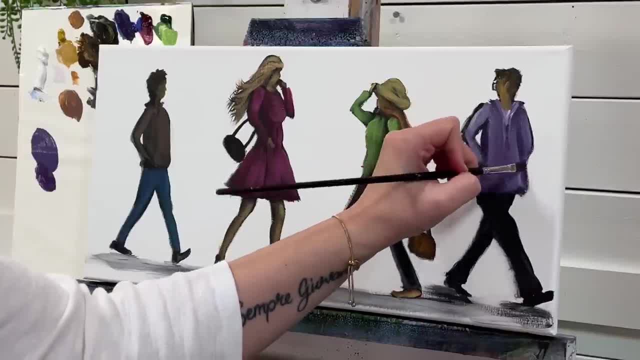 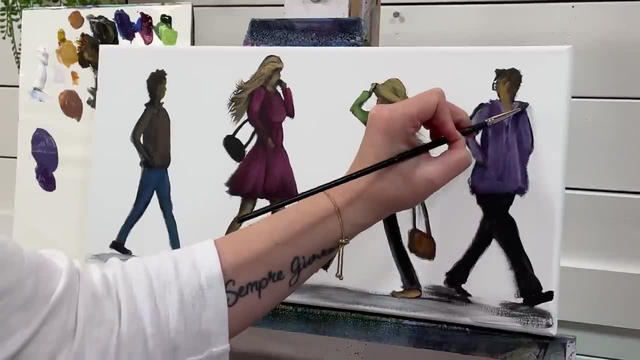 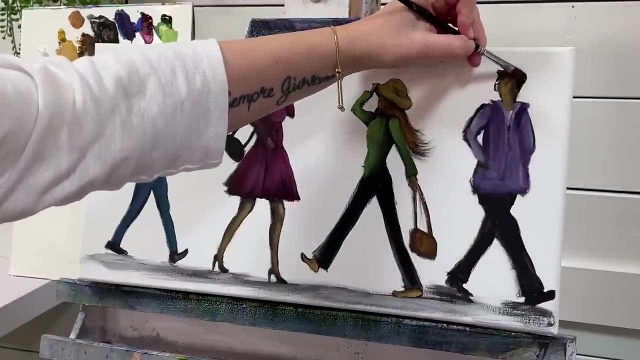 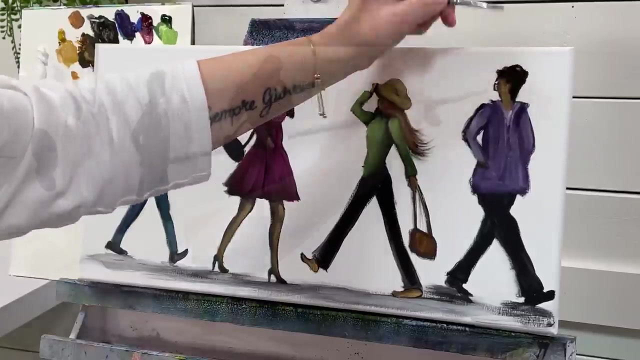 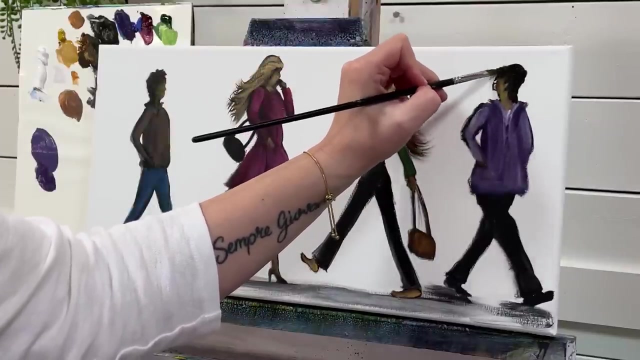 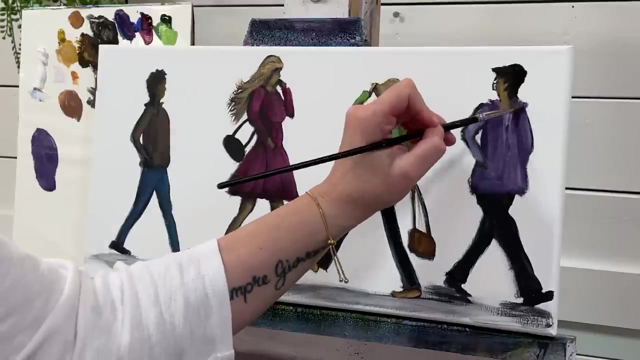 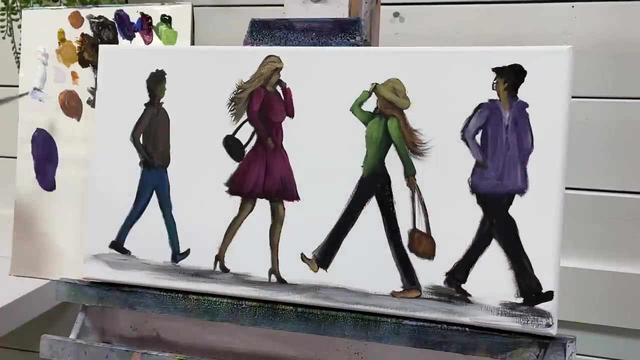 and here's the darker shade: take a little bit more black, take a little bit more black, take a little bit more black, bring his, bring his, bring his head up a little bit higher here, head up a little bit higher here here, here, if you give him maybe some. 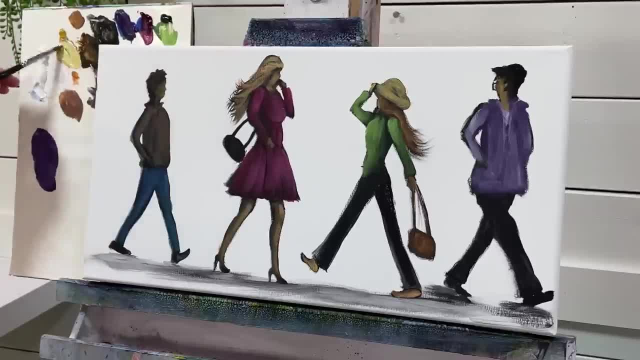 if you give him maybe some, if you give him maybe some khaki colored pants, we'll take some green khaki colored pants. we'll take some green khaki colored pants. we'll take some green, yellow ochre, yellow ochre, yellow ochre and some white. 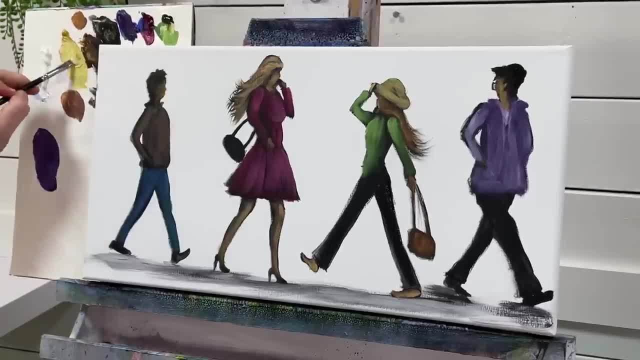 and some white and some white. make sure i don't have, make sure i don't have. make sure i don't have too too much, too. too much too, too too much. paint on my brush, just mix it up and then. paint on my brush, just mix it up and then. 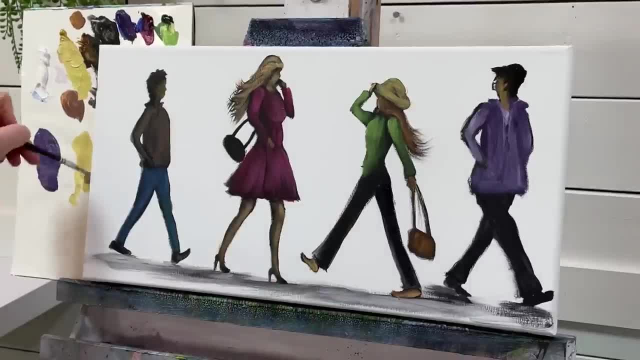 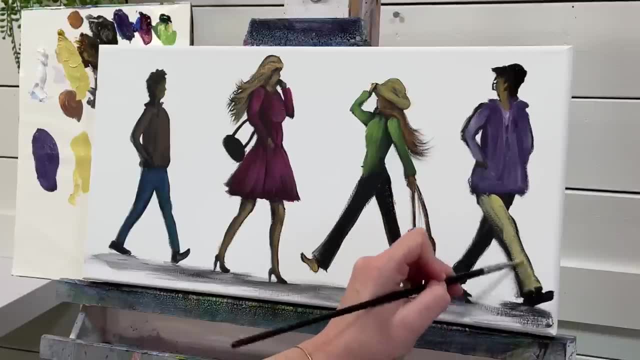 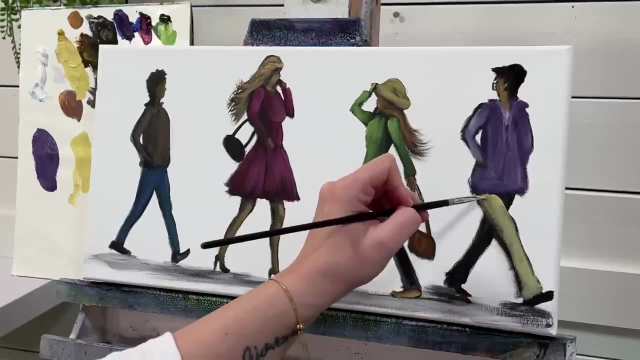 paint on my brush, just mix it up and then have the excess, have the excess, have the excess out of the brush. okay, we're gonna just leave it a little. okay, we're gonna just leave it a little. okay, we're gonna just leave it a little darker in between. 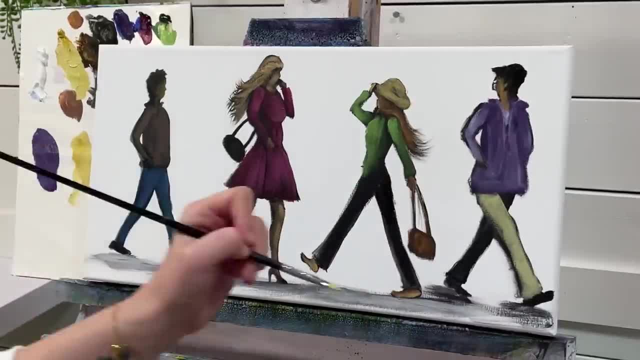 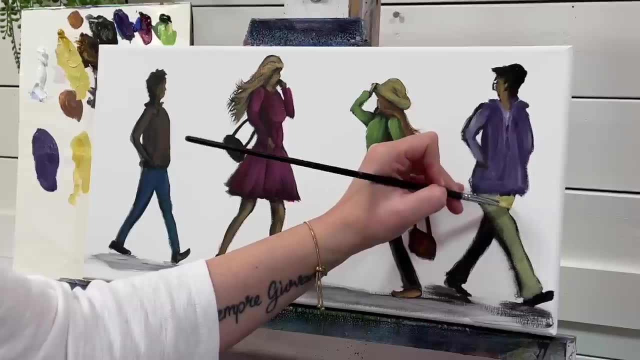 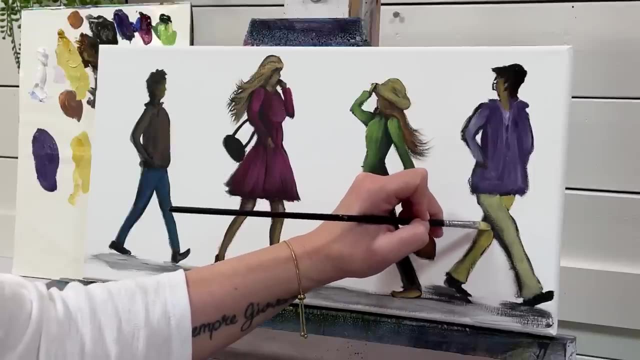 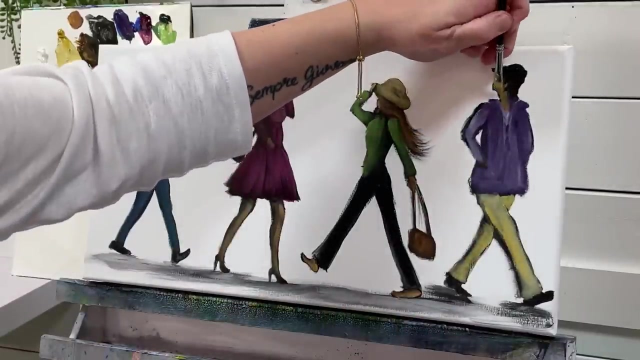 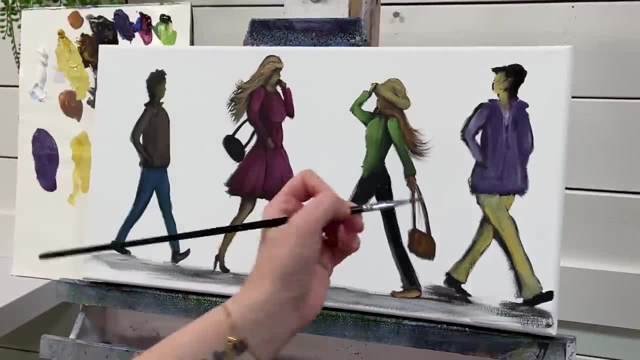 that's behind. that's behind. i'm gonna add some more black with my purple. i'm gonna add some more black with my purple. i'm gonna add some more black with my purple. make it darker, make it darker, make it darker under the base of the coat. 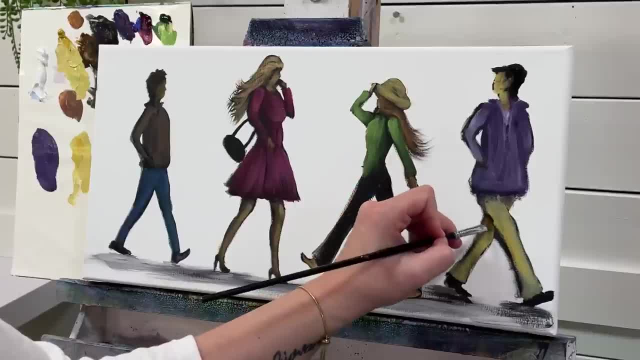 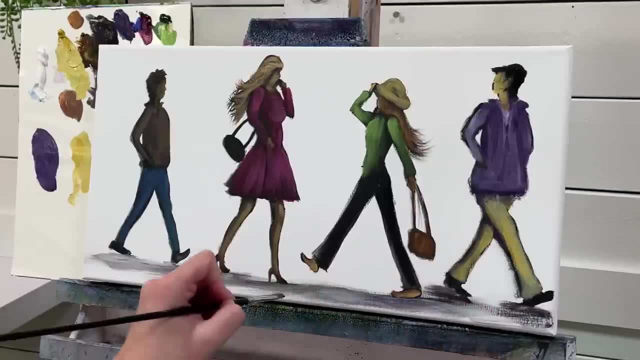 under the base of the coat, under the base of the coat, a little bit of a shadow. i'll just use this for. i'll just use this for. i'll just use this for some more shadows down here as well. some more shadows down here as well. some more shadows down here as well. 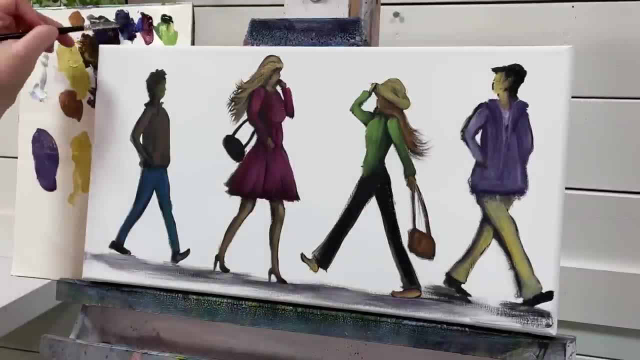 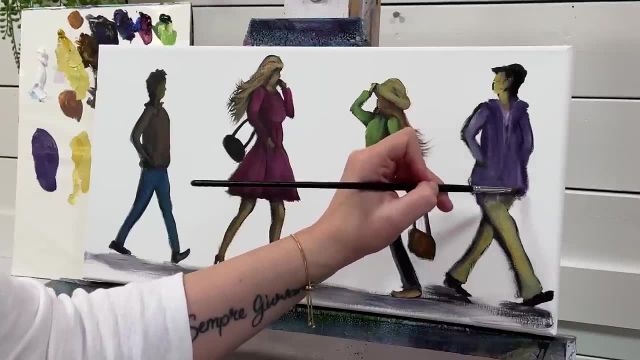 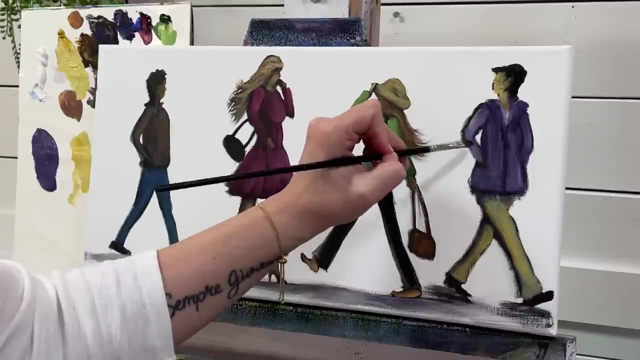 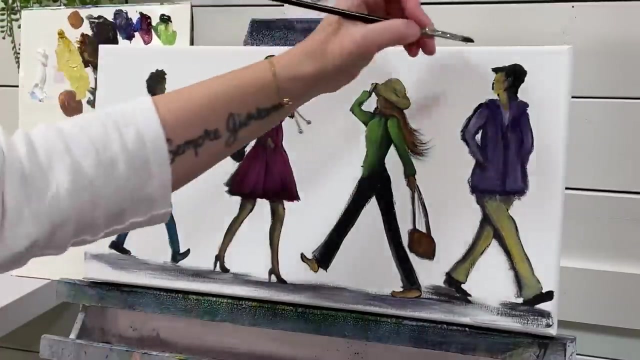 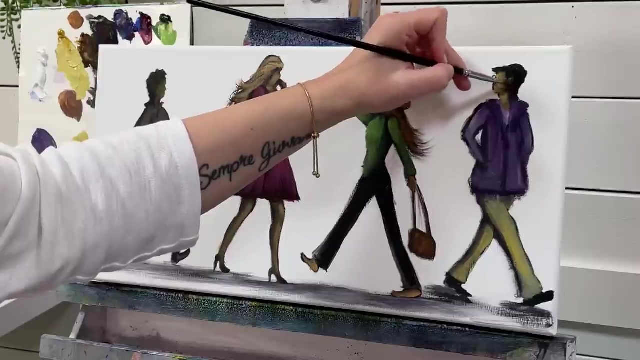 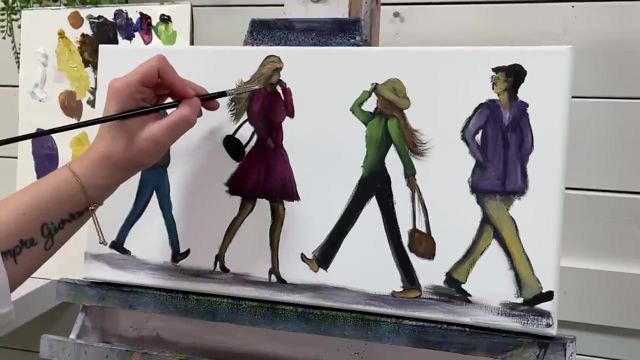 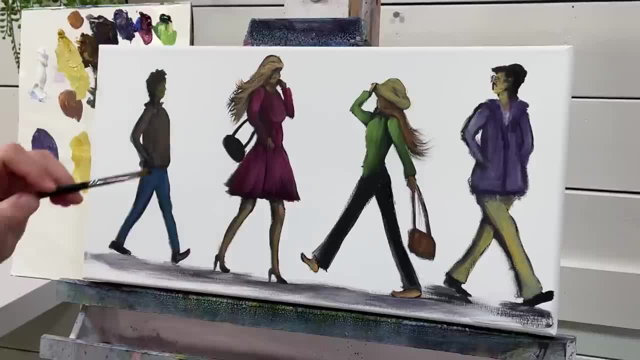 add a little bit of burnt sienna. and add a little bit of burnt sienna and black right in here. black right in here, black right in here. make that a bit darker. let's take our. make that a bit darker. let's take our make that a bit darker. let's take our round brush. 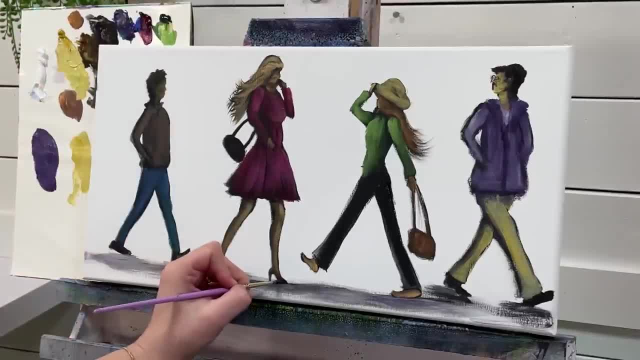 round brush, round brush. pick up some black and a little bit of pick up some black and a little bit of pick up some black and a little bit of water on there, water on there, water on there. and just define her heels a little bit. and just define her heels a little bit. 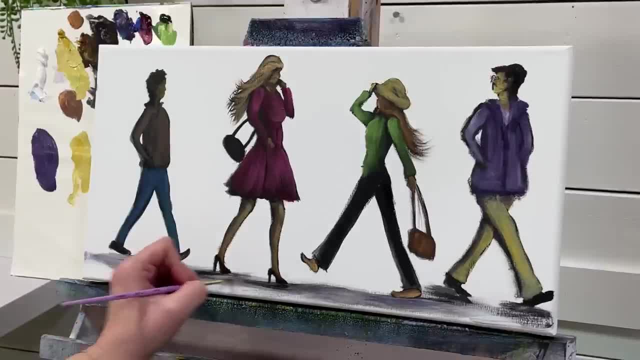 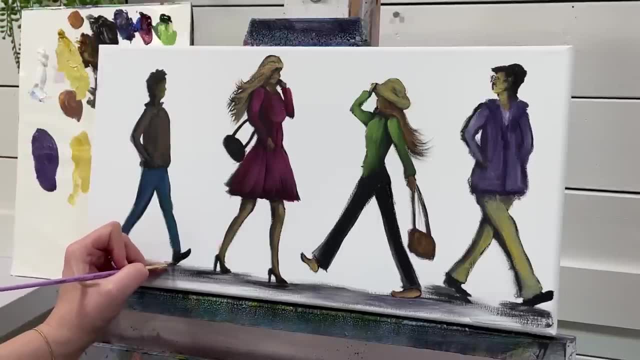 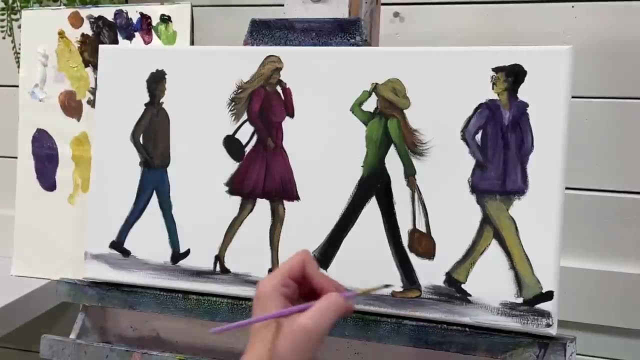 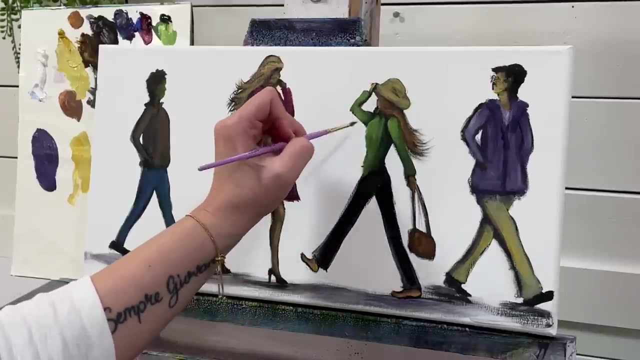 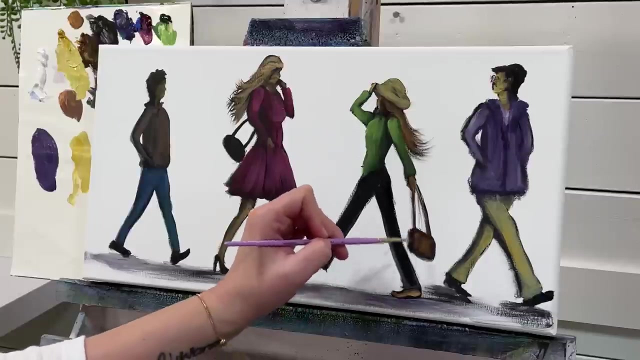 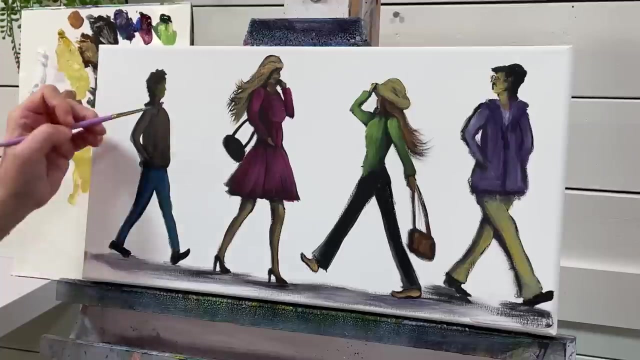 and just define her heels a little bit more so they more so, they more so. they aren't see-through, aren't see-through. add those last little details. shadows, add those last little details, shadows, add those last little details. shadows and highlights. and maybe a last little highlight here: 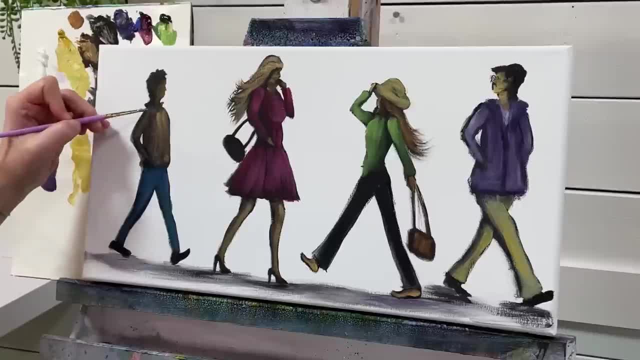 and maybe a last little highlight here, and maybe a last little highlight here, on the jacket, on the jacket, on the jacket, once it has had time to dry, once it has had time to dry, once it has had time to dry, it fades quite a bit. i'll just add a little bit more there. 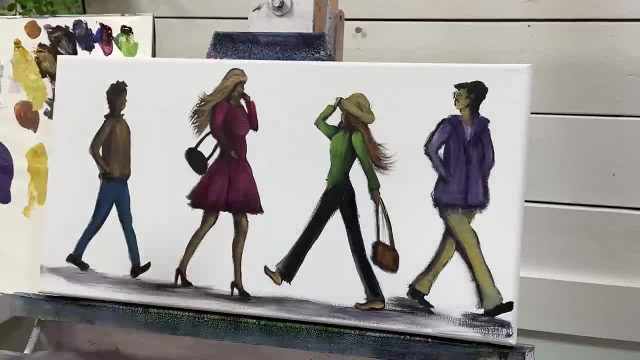 i'll just add a little bit more there. i'll just add a little bit more there. okay, i'm going to add. okay, i'm going to add. okay, i'm going to add a hat to this man over here. it already. a hat to this man over here, it already. a hat to this man over here. it already looks like he's got a hat on, so i'm looks like he's got a hat on. so i'm looks like he's got a hat on, so i'm going to just go with that. going to just go with that. 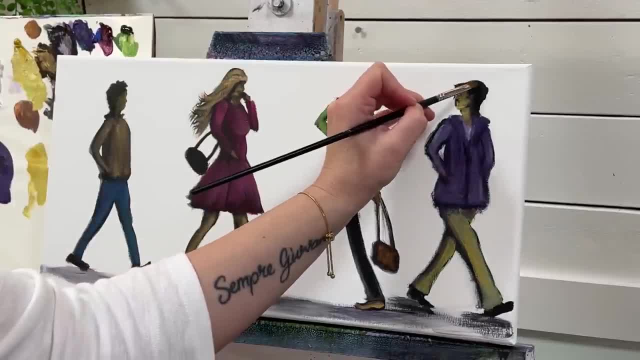 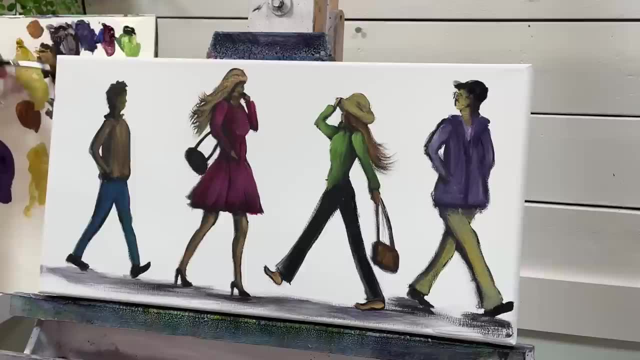 going to just go with that and just shape it a little bit better. and just shape it a little bit better and just shape it a little bit better. so round like ball cap, so round like ball cap, so round like ball cap. get a little bit of what i've got left. 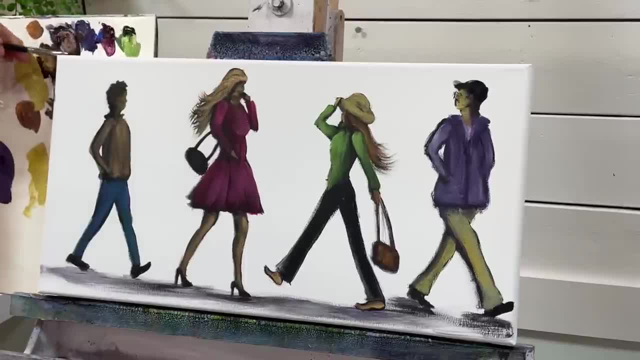 get a little bit of what i've got left. get a little bit of what i've got left here i can make a nice here. i can make a nice here. i can make a nice dark color with that crimson a little bit. dark color with that crimson a little bit. 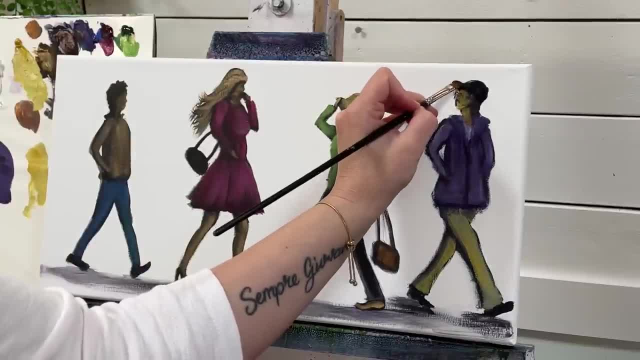 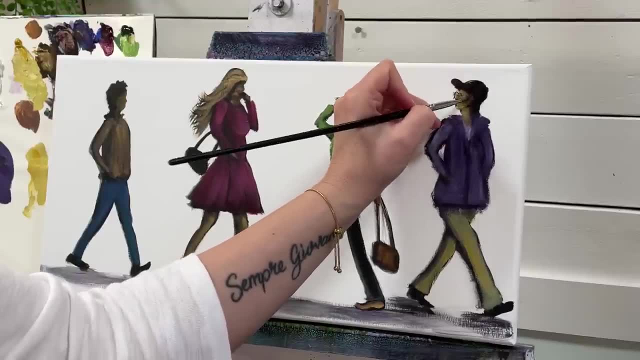 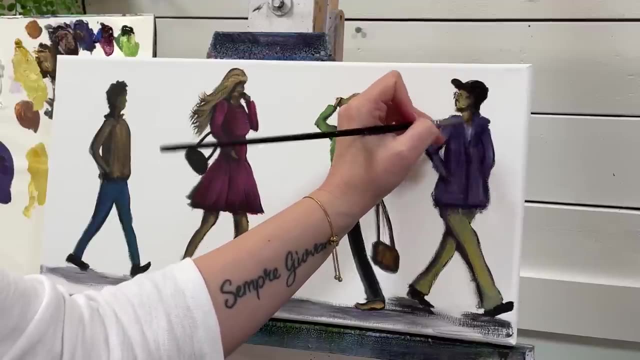 dark color, with that crimson, a little bit of of of blue and black, blue and black, blue and black. we'll just, we'll just, we'll just flip it up, flip it up, flip it up like that. his ears about right there, his ears about right there, his ears about right there, jawline. 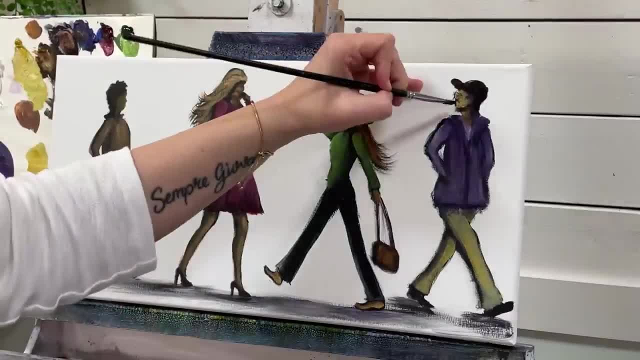 shadow. looks like he's got a bit of a beard. looks like he's got a bit of a beard. looks like he's got a bit of a beard. so so so, if you wanted to add a beard, you can. if you wanted to add a beard, you can. 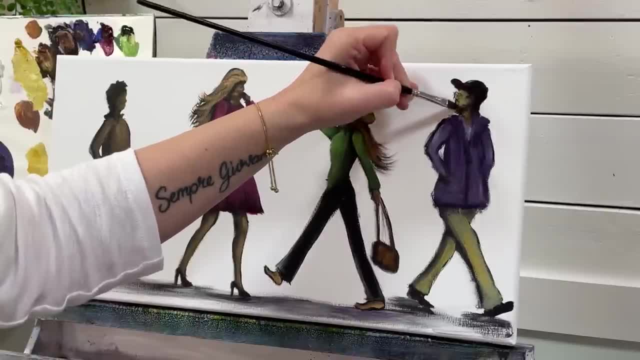 if you wanted to add a beard, you can just stipple on whatever color that of. just stipple on whatever color, that of just stipple on whatever color that of that beard you want want it to be that beard you want. want it to be that beard you want, want it to be. i'm going to add a little more to 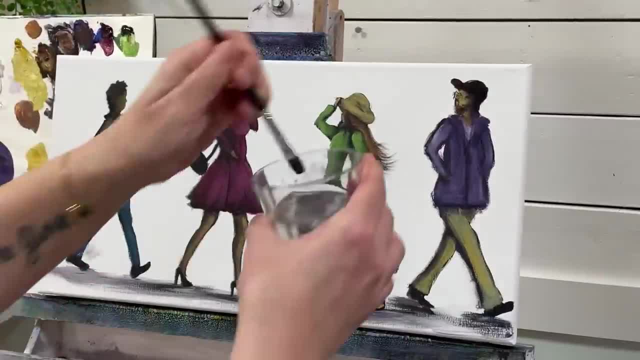 i'm going to add a little more to. i'm going to add a little more to his pants burnt, sienna, and that purple. his pants burnt, sienna, and that purple. his pants burnt sienna, and that purple color, color, color. a little bit of water, a little bit of water. 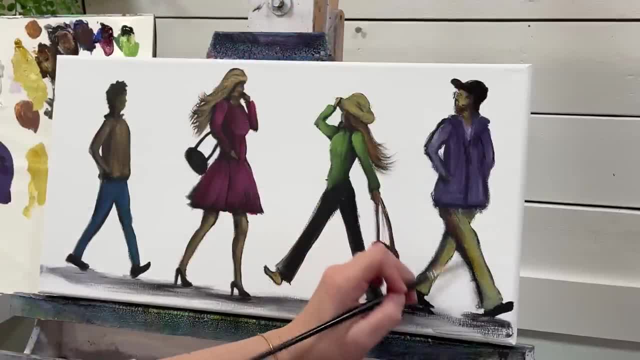 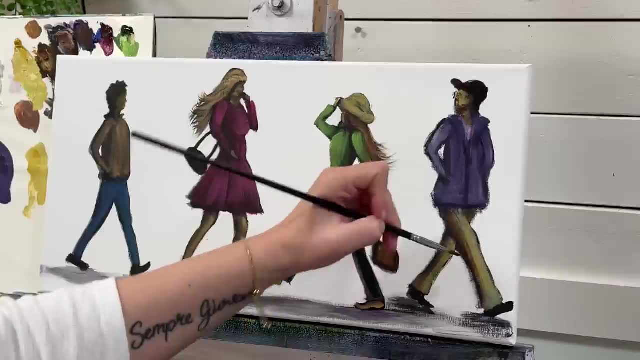 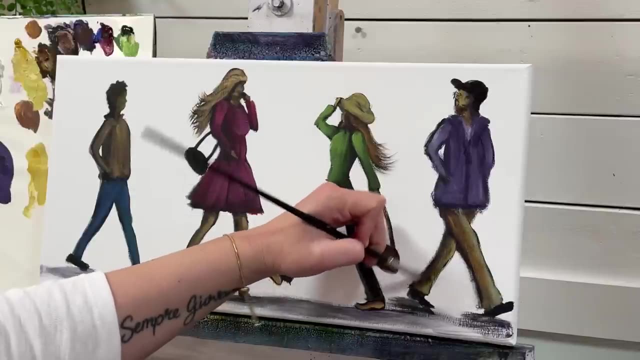 a little bit of water and i want to just kind of shadow this, and i want to just kind of shadow this and i want to just kind of shadow this in here, in here, in here. really fun showing you guys how to add. really fun showing you guys how to add. 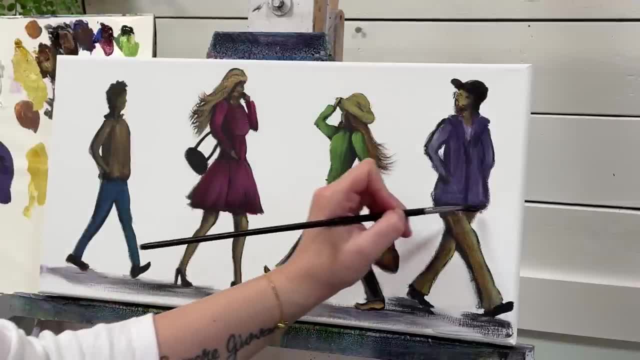 really fun showing you guys how to add figures- simple figures like this to your figures. simple figures like this to your figures. simple figures like this to your paintings. let me know if you guys are paintings. let me know if you guys are paintings. let me know if you guys are enjoying these. 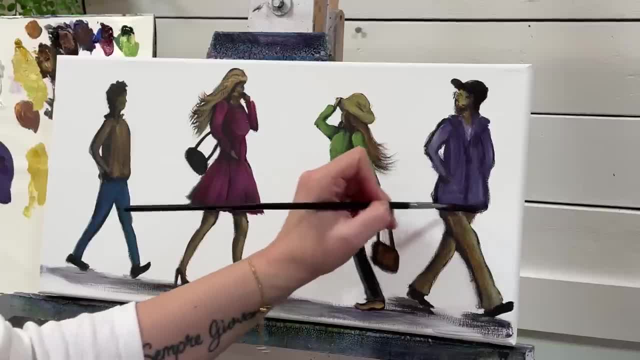 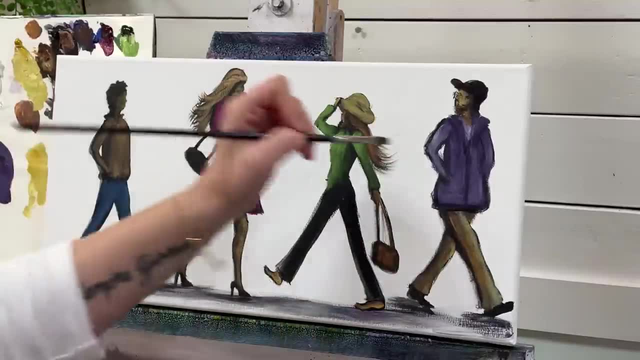 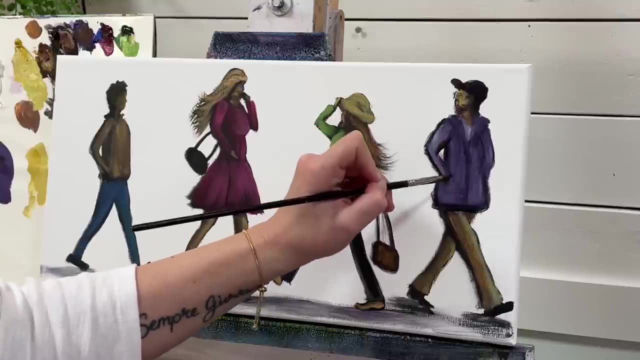 enjoying these. enjoying these, i'm going to bring his coat down a. i'm going to bring his coat down a. i'm going to bring his coat down a little lower here to find the shadow areas black right. to find the shadow areas black right. to find the shadow areas black right there. 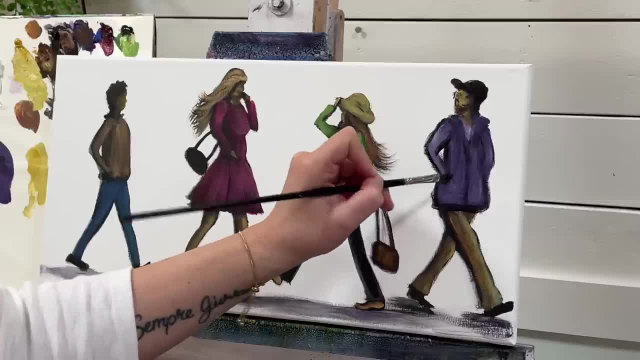 to find the shadow areas, black right there. probably got his hand in his pocket right. probably got his hand in his pocket right. probably got his hand in his pocket right there. so we'll just add a little there. so we'll just add a little there. so we'll just add a little scoop. 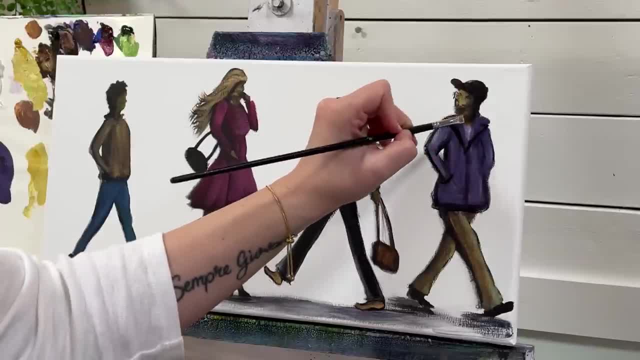 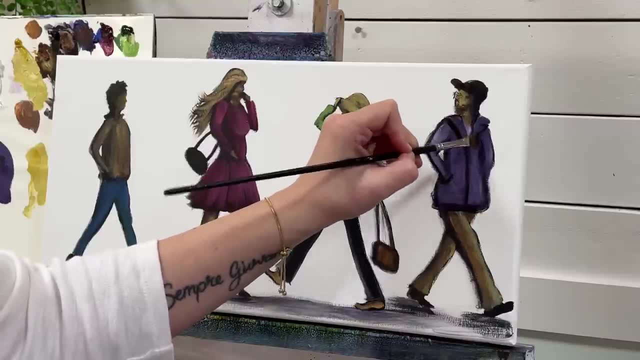 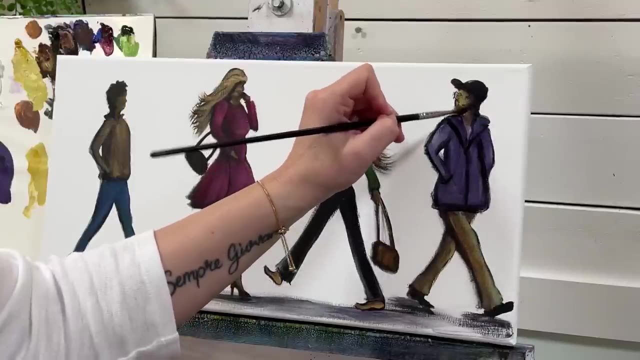 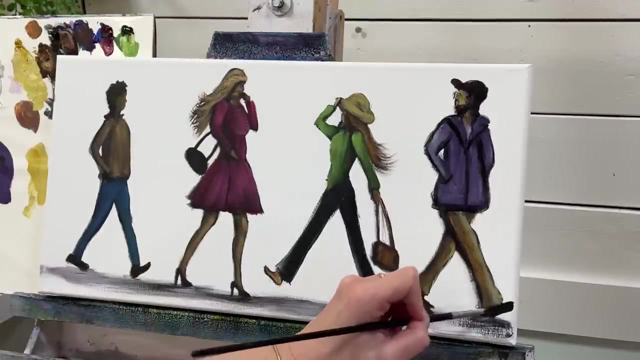 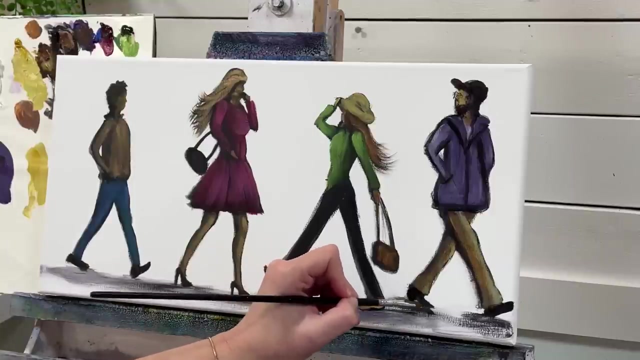 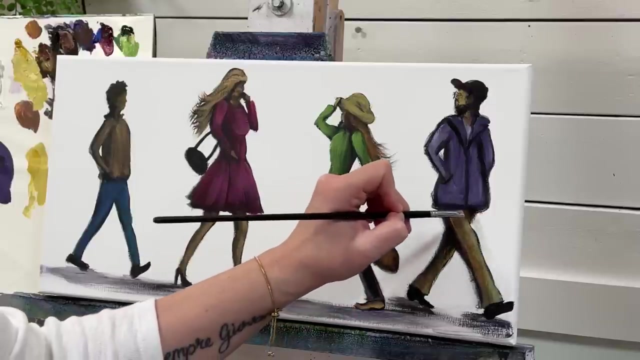 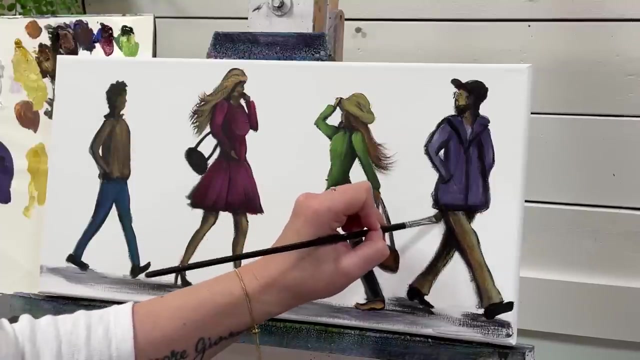 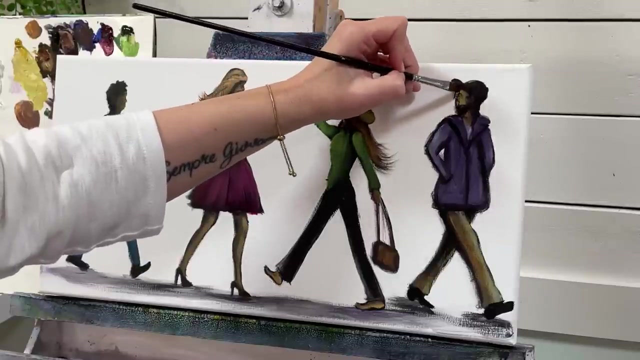 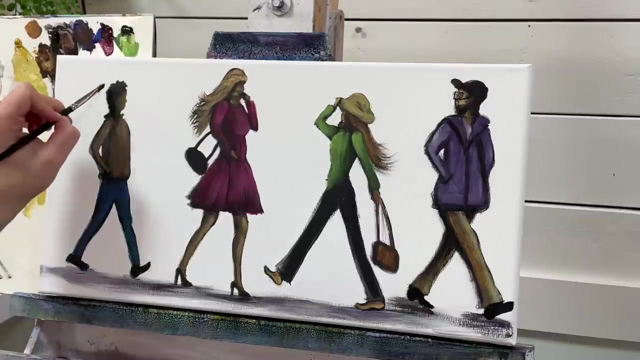 outline the collar, a shadow out this shadow, out this shadow, out this back leg, back leg. you'll see it just doesn't take very, you'll see, it just doesn't take very, you'll see, it just doesn't take very much to add, much, to add much, to add a little bit more here and there, and 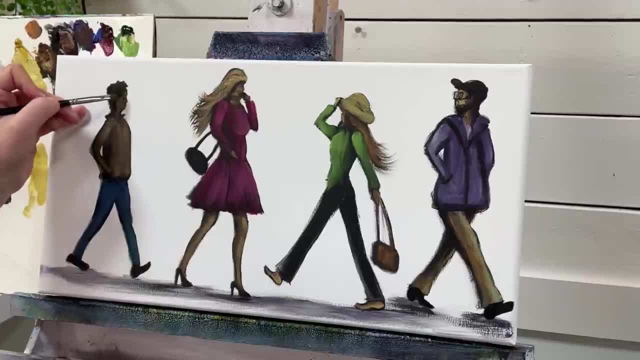 a little bit more here and there and a little bit more here and there and totally change the look of your figures. the look of your figures just subtle little shadows. a little bit just subtle little shadows. a little bit just subtle little shadows. a little bit extra black. 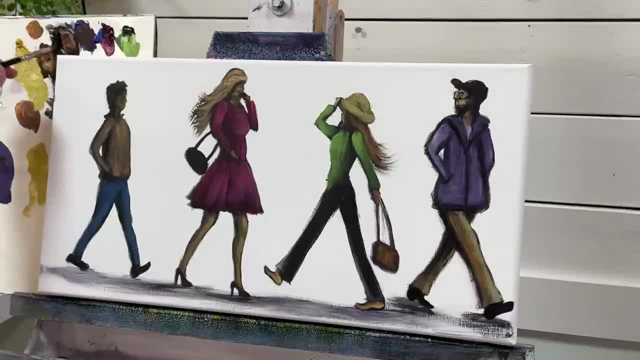 extra black, extra black, and you guys can feel free to add any, and you guys can feel free to add any, and you guys can feel free to add any colors that you want. these are just what colors that you want. these are just what colors that you want. these are just what i. 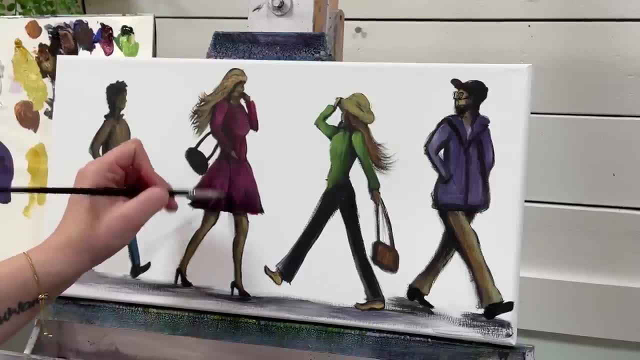 i, i chose today. if you want to make it look, chose today. if you want to make it look, chose today if you want to make it look like her fabrics, like her fabrics, like her fabrics- a little bit ruffled, a little bit ruffled, a little bit ruffled, and just add a few, or just even like: 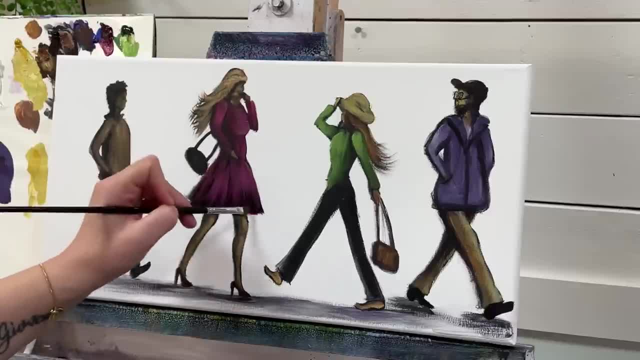 and just add a few, or just even like, and just add a few or just even like for shadows bolts for shadows bolts for shadows bolts. just add some lighter areas which we have, just add some lighter areas which we have, just add some lighter areas which we have, and then we just add a little bit of. 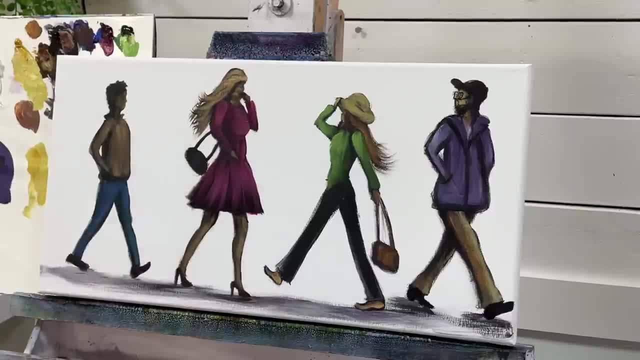 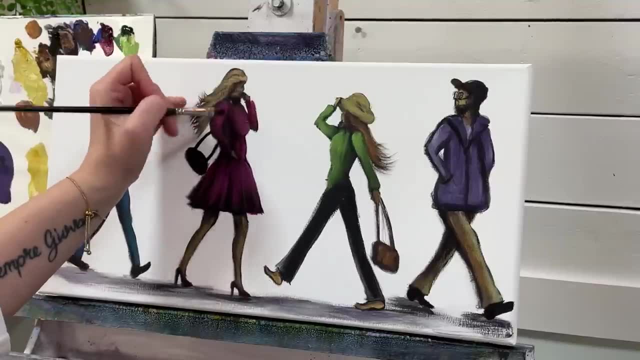 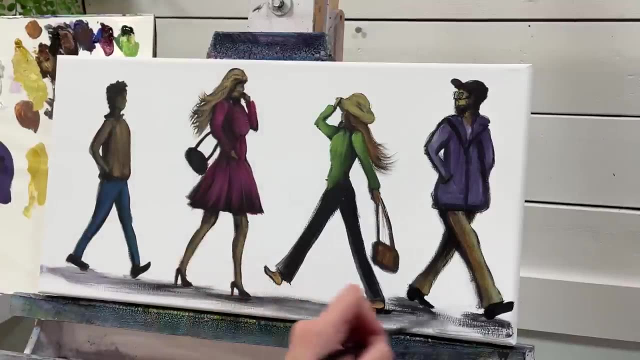 and then we just add a little bit of, and then we just add a little bit of black, okay, so i think i'm going to leave it okay. so i think i'm going to leave it okay. so i think i'm going to leave it like this: 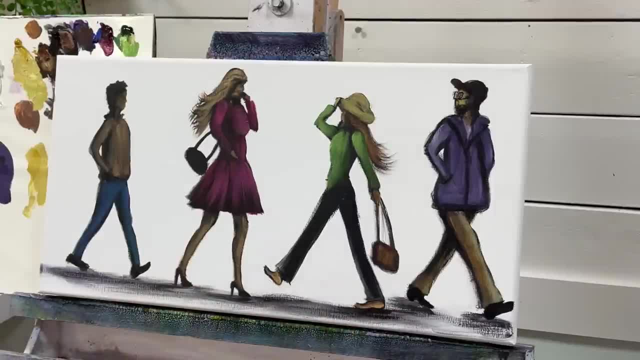 like this. like this: hopefully got a good idea of how you can hopefully got a good idea of how you can hopefully got a good idea of how you can start painting some walking figures. start painting some walking figures. start painting some walking figures. thanks so much for watching and. 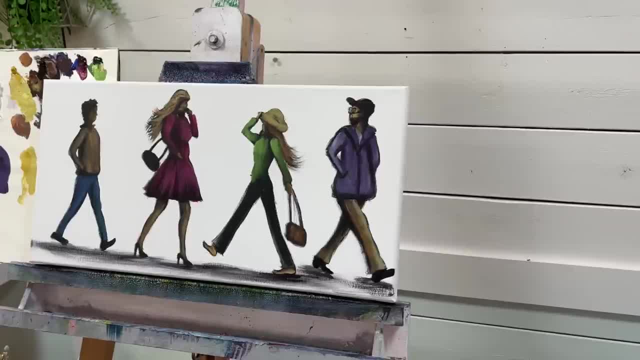 thanks so much for watching. and thanks so much for watching and don't forget to subscribe to my channel. don't forget to subscribe to my channel. don't forget to subscribe to my channel for more, for more, for more. i'll see you all soon in my next video.